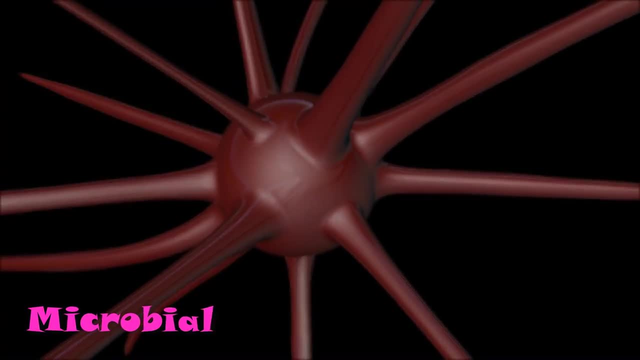 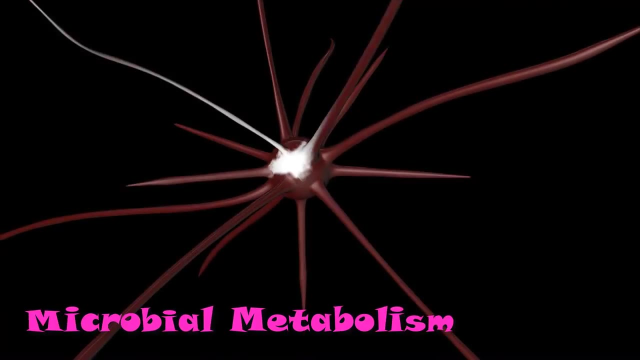 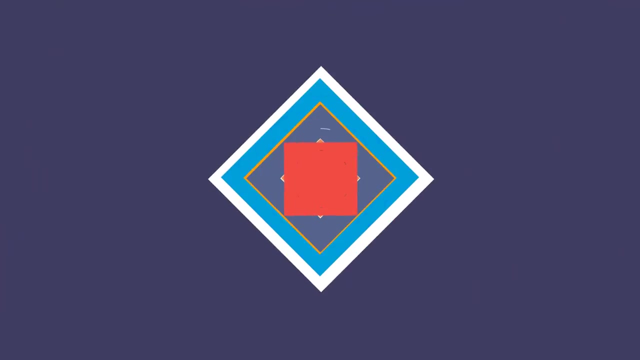 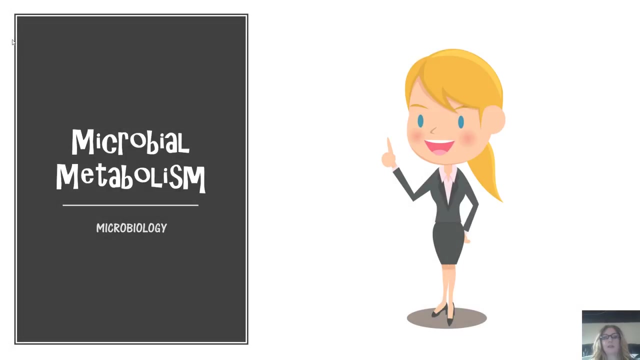 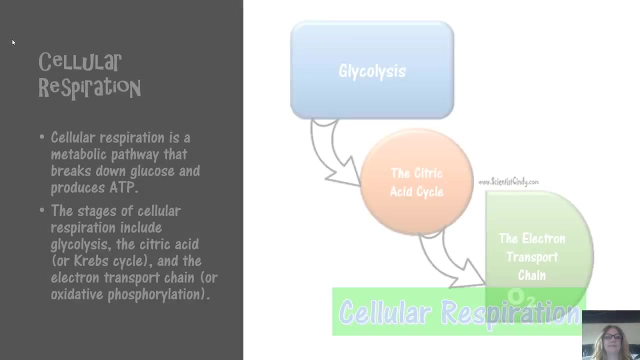 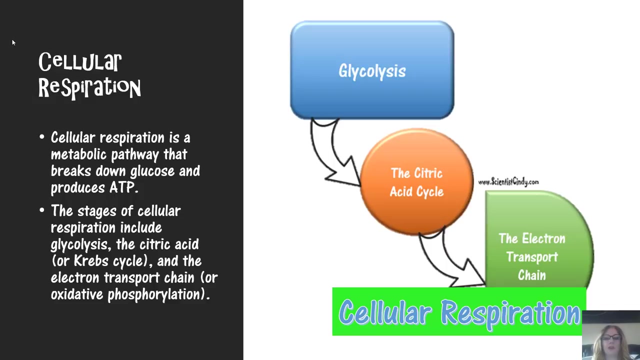 Okay, so this is your review for your next exam, which will be on Microbial Metabolism. So let's start by looking at the pathway that you are probably already familiar with from your basic biology courses or your high school biology courses. This pathway is called cellular respiration. Cellular respiration is a metabolic pathway that breaks 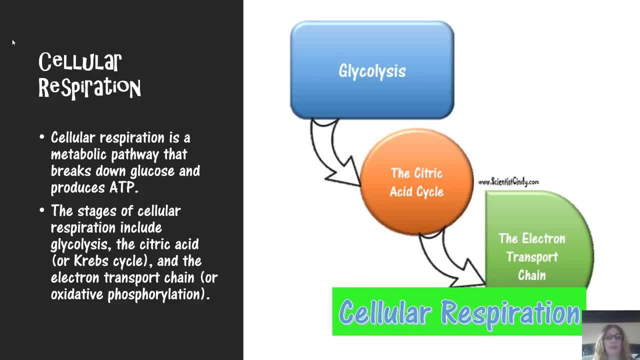 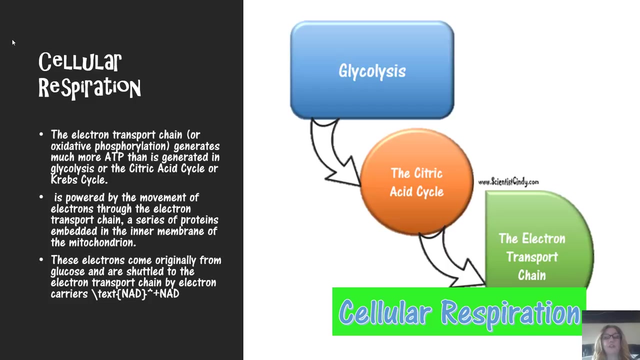 down glucose to produce ATP. The stages of cellular respiration include these three stages, which are glycolysis, the citric acid cycle, otherwise known as the Krebs cycle, and the electron transport chain, otherwise known as oxidative phosphorylation. The electron transport chain, otherwise known as oxidative phosphorylation. 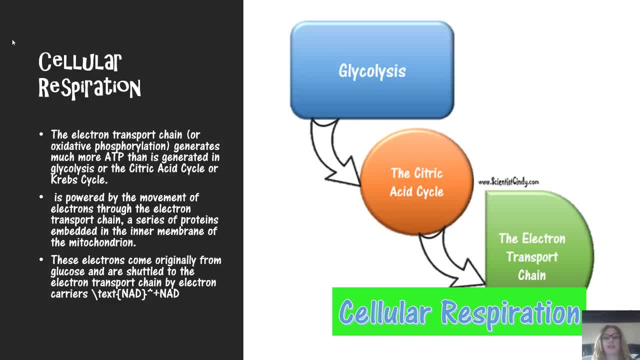 generates a cell-based cell-based cell. The cell-based cell is a cell-based cell that is much more ATP than is generated in glycolysis or in the citric acid cycle or Krebs cycle. The electron transport chain is powered by the movement of electrons through the electron. 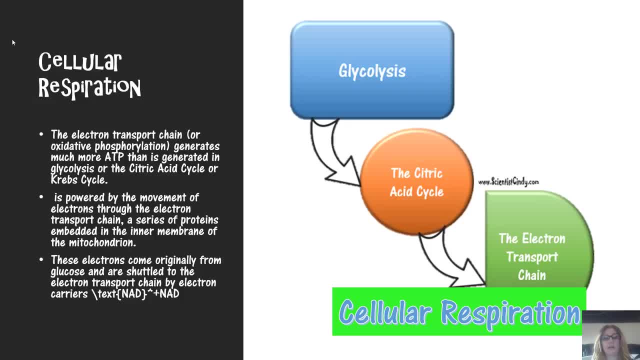 transport chain, which is a series of proteins that are embedded either in the inner membrane of the prokaryote or in the inner membrane of the mitochondria, And these electrons come originally from the glucose molecule, which is broken down in glycolysis. These electrons are shuttled to the 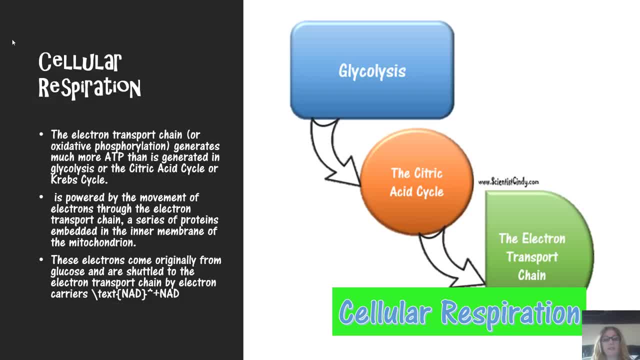 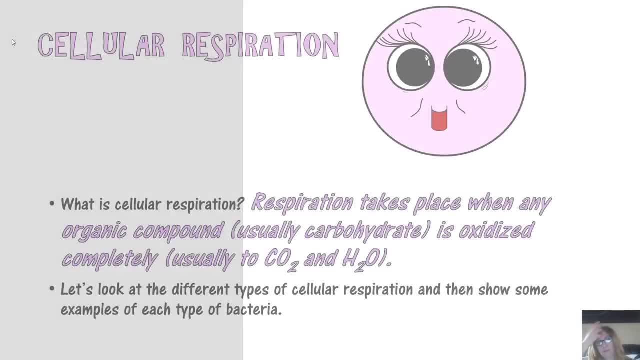 electron transport chain using electron carriers such as NADH and FADH2.. So how do we define cellular respiration? So cellular respiration: respiration takes place in the cellular respiration. So cellular respiration: respiration takes place in the cellular respiration. 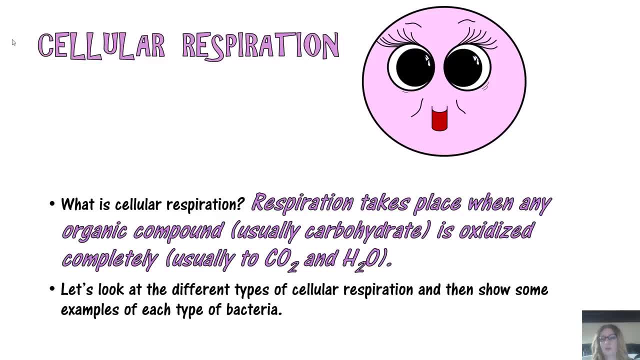 So cellular respiration takes place when any organic compound, which is usually a carbohydrate, is oxidized completely, usually to carbon dioxide and water. Now, when we say oxidized, what we really are meaning is that we're meaning that that molecule is being broken down. by breaking, 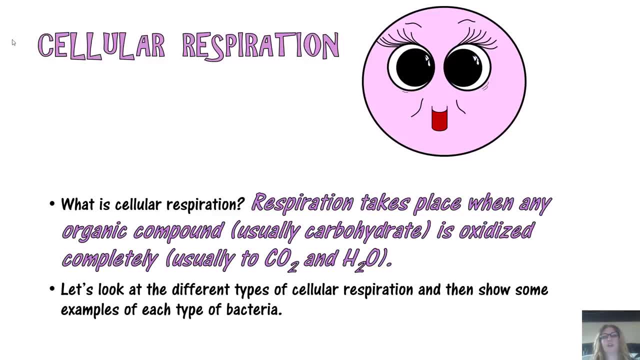 its bonds and removing the individual electrons from the molecule itself. So let's look at different types of. We'll look at different types of cellular respiration and we'll show examples of different types of bacteria in this presentation, and we'll look at a bunch of different pathways as well as some different peripheral ideas, such as enzyme function. 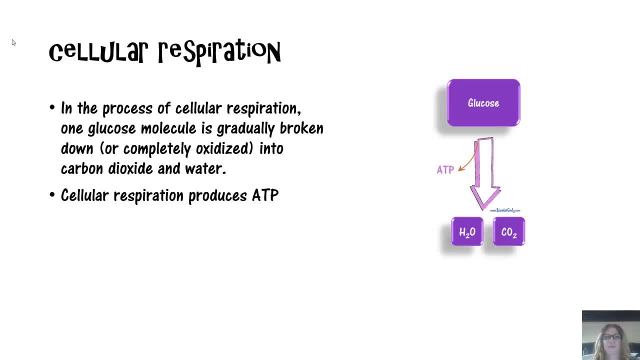 Okay, so this is literally the easiest diagram you will ever see to explain cellular respiration, and I'm very proud of it. Okay, so this is literally the easiest diagram you will ever see to explain cellular respiration, and I'm very proud of it. 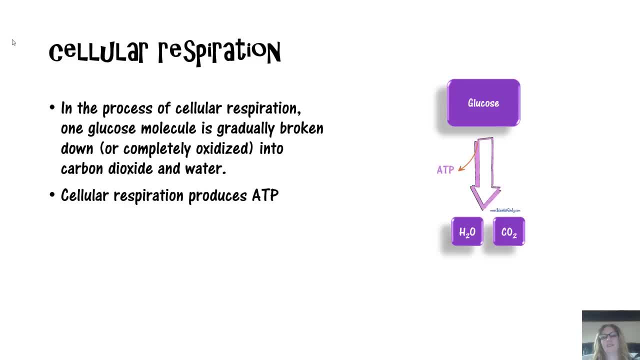 So cellular respiration, in the most concise nutshell I could think of, is literally this. The process of cellular respiration is that you will take one glucose molecule and you will break it down or completely oxidize the molecule and produce ATP in the process. 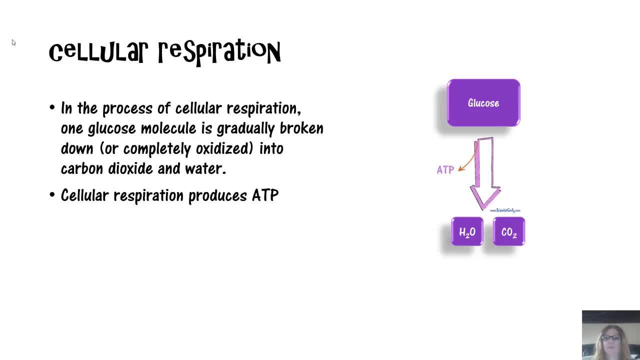 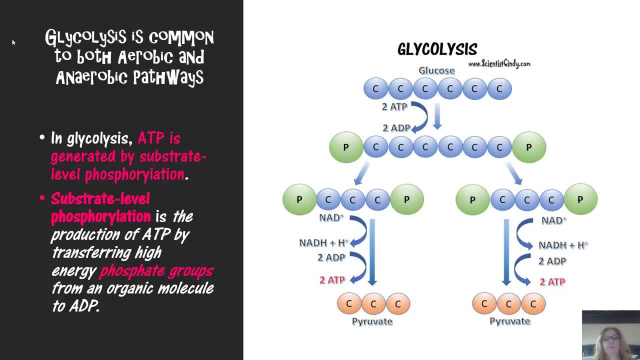 OK, so let's begin to look at this in a little bit more detail. Alright, So we begin cellular respiration with the process of glycolysis. Alright, So we begin cellular respiration with the process of glycolysis. Now, glycolysis is common to both aerobic and anaerobic pathways. 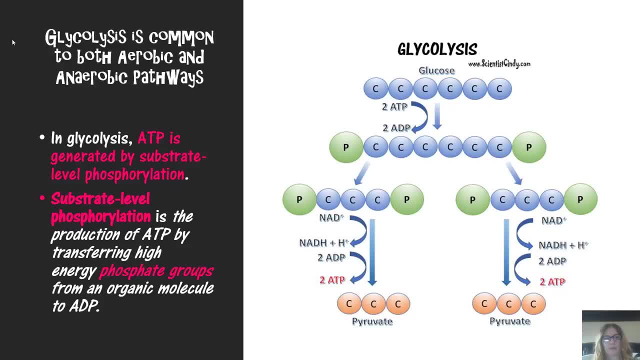 And we'll talk about those anaerobic pathways later. In glycolysis, ATP is generated by what is called substrate-level phosphorylation. Okay, so let me say that again, In glycolysis, ATP is generated by substrate-level phosphorylation. 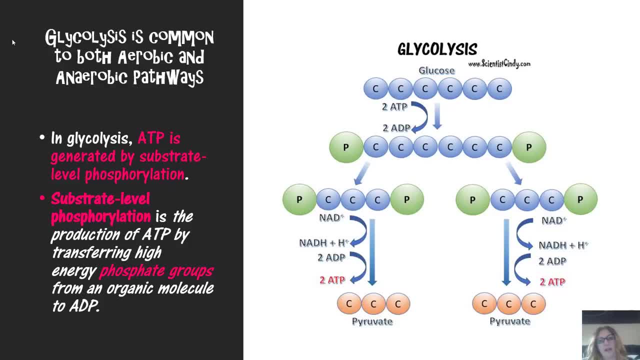 In contrast, just to bring that out, in the electron transport chain, ATP will be created through oxidative phosphorylation. So that is the contrast there. So in glycolysis, ATP is generated by substrate-level phosphorylation. Substrate-level phosphorylation is the production of ATP. 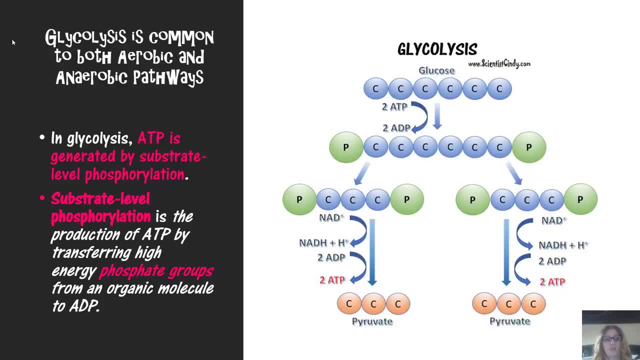 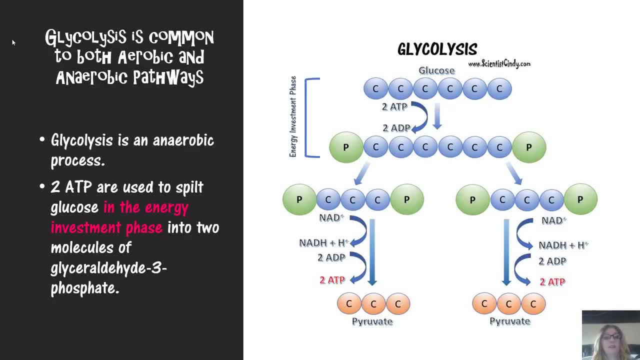 by transferring high-energy phosphate groups from an organic molecule to ADP Glycolysis. Glycolysis is an anaerobic process, so we do not need oxygen in order to undergo glycolysis. Two ATP are actually invested at the beginning of the glycolysis process. 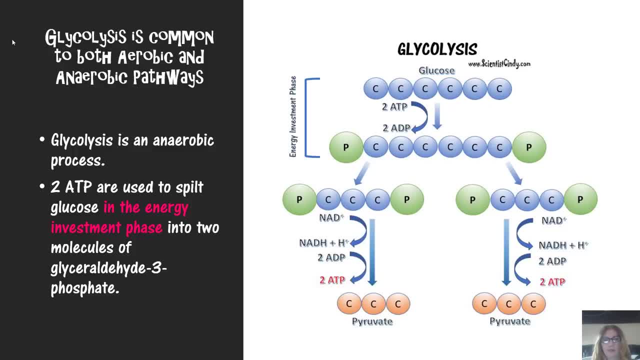 and we call this the energy investment phase here at the beginning. So two ATP are actually used or are invested at the beginning of glycolysis in order to split the glucose molecules. So the six carbon atoms that make up glucose are split into two individual molecules. 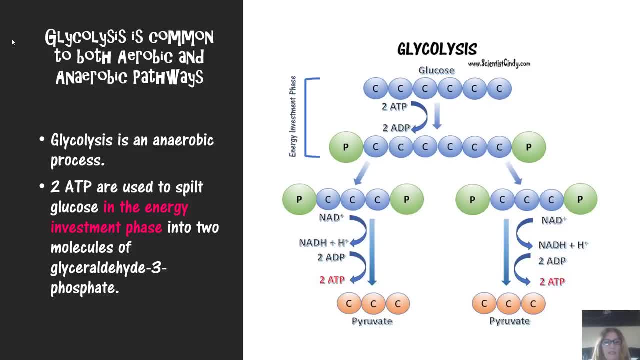 that are made up of three carbon atoms each. There's also some other atoms there too that I've omitted just for simplicity. So the two ATP are used to split the glucose molecule in the energy investment phase, and the first product that we get from splitting is actually called glyceraldehyde 3-phosphate. 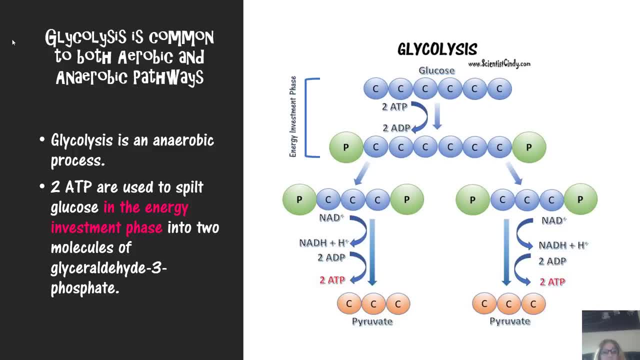 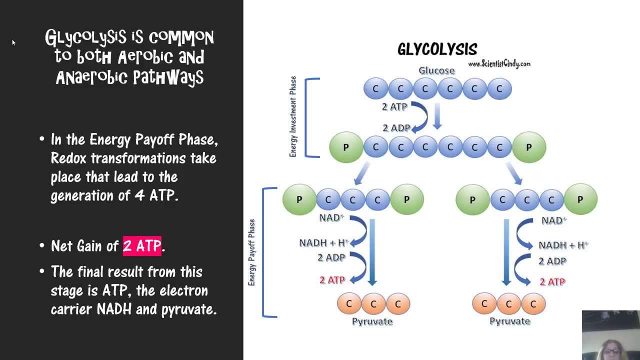 or G3P, or glyceraldehyde 3-phosphate, And then from there it will continue on and get converted into pyruvate, which I'll show you in the next video, Next slide here. So after G3P, then we enter what's called the energy payoff phase of glycolysis. 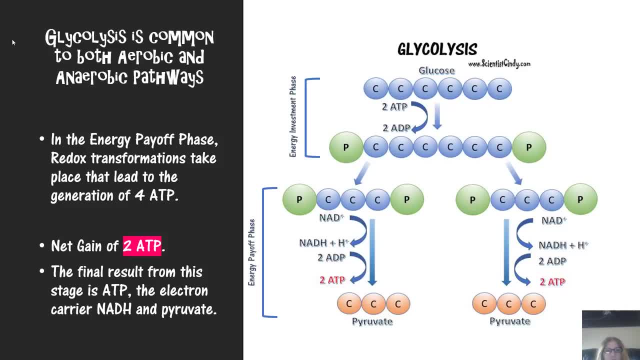 This is where we end up getting paid back with interest. So in the energy payoff phase, redox transformations take place that lead to the generation of four ATP, So we end up with a net gain of two ATP. So the final result from this stage is: 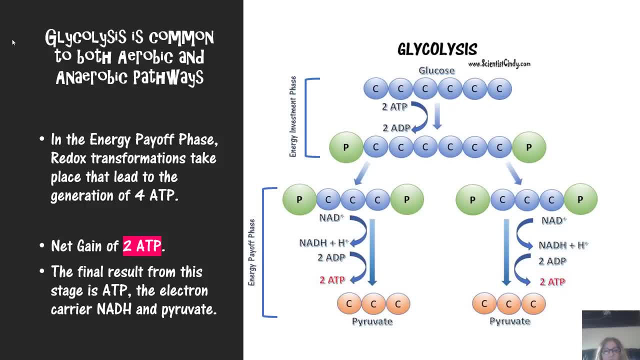 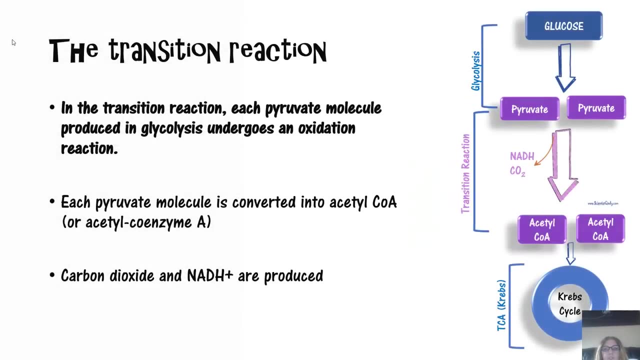 we gain two ATP and we also end up gaining two of the electron carrier, which is NADH, and we also end up with two pyruvate molecules from our glucose molecule. So we ended up making our money back and more. 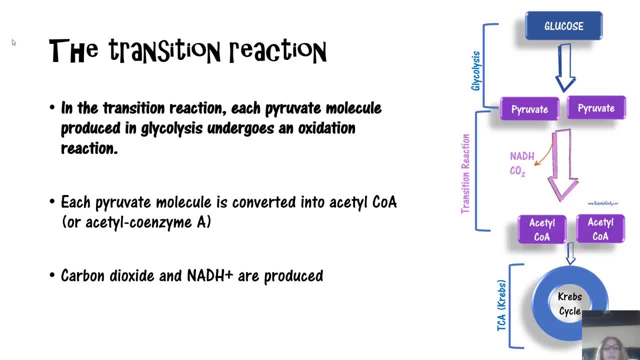 So you might remember from our first slide that we have three different stages of glycolysis. We have three stages, if you will, of cellular respiration. The first one is glycolysis that we just discussed, and the next one is the Krebs cycle. 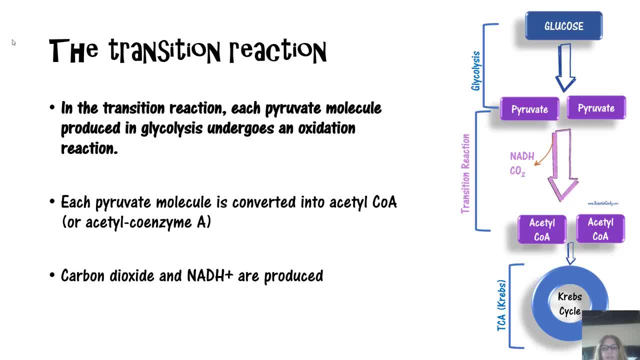 Between glycolysis and the Krebs cycle there is a small transition reaction that does take place. I have it magnified here so it looks very large, but it's not considered a real phase or stage, so it didn't really get a block. 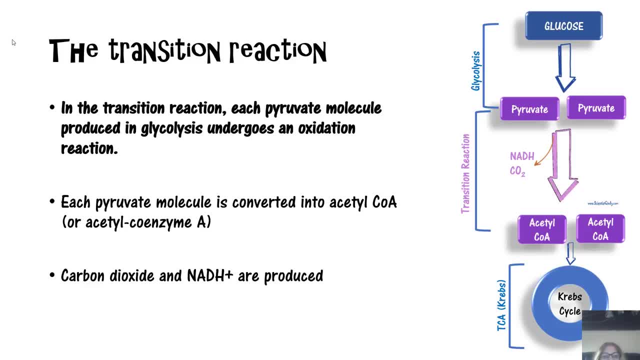 So it didn't really get a big block on that first slide. So it's just simply called a transition reaction. But nonetheless it is important and we should make note of it. So we will do that All right. so here in this diagram I have glucose in its very, very shortened form. 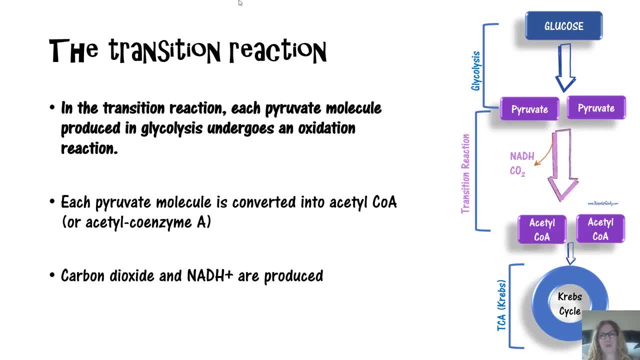 So we just have glucose going to- I'm sorry- glycolysis in its shortened form, going just to glucose to its final form. So we just have glucose to its final product of two pyruvate molecules, Those two pyruvate molecules, during the transition reaction. 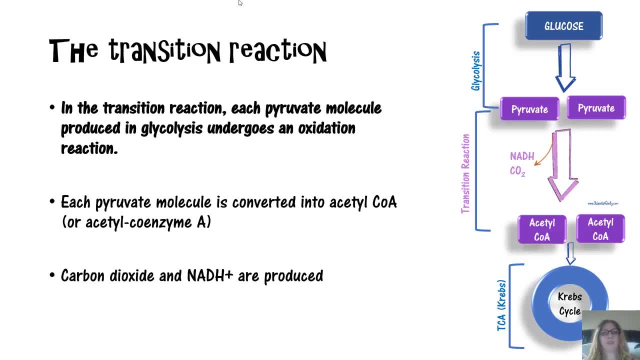 are actually going to be converted to two acetyl CoA molecules. Now, if you look at what comes out of the transition reaction, the transition reaction does not actually create any ATP, but it does create an electron carrier. It creates NADH. 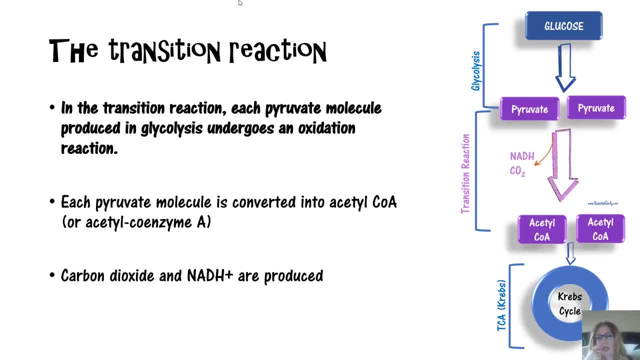 It also creates CO2.. And it does that per pyruvate molecule. I didn't really make that clear on this and I probably should have, So let me just make that clear in my words here. So for each pyruvate molecule, you will generate one NADH and one carbon dioxide. 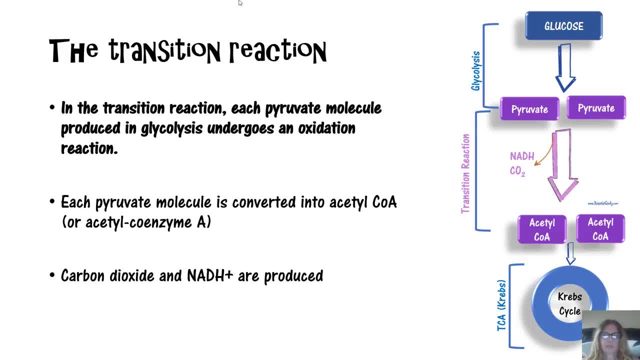 which, if I had kept the carbons on here, would have made more sense. So pyruvate, So glucose is a six-carbon sugar. Pyruvate is a three-carbon molecule And you see here that we lose a carbon in the transition reaction. 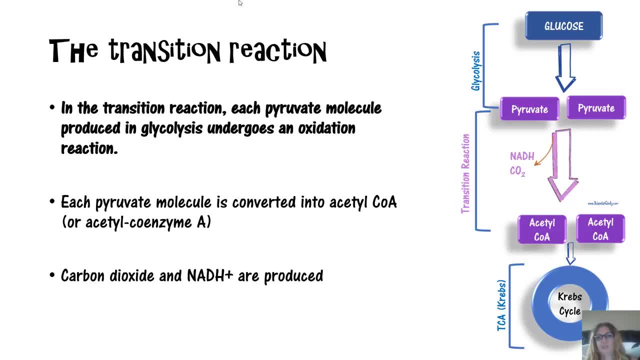 So we end up losing a carbon to carbon dioxide. So each pyruvate loses a carbon. So we end up losing two carbon dioxides and we create two NADH In the transition reaction per one glucose molecule. Acetyl-CoA is also a two-carbon molecule. 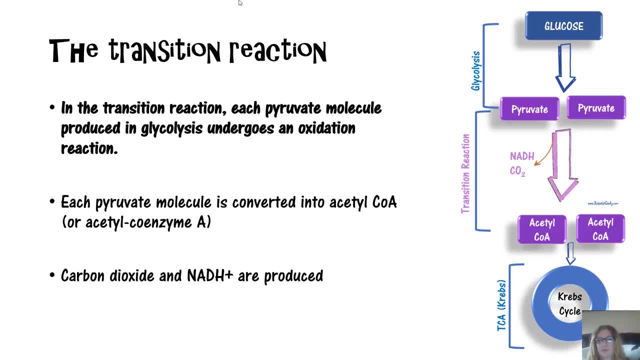 All right. So acetyl-CoA enters the Krebs cycle one molecule at a time. So one acetyl-CoA at a time enters the Krebs cycle, otherwise known as the TCA cycle or the citric acid cycle. All right? 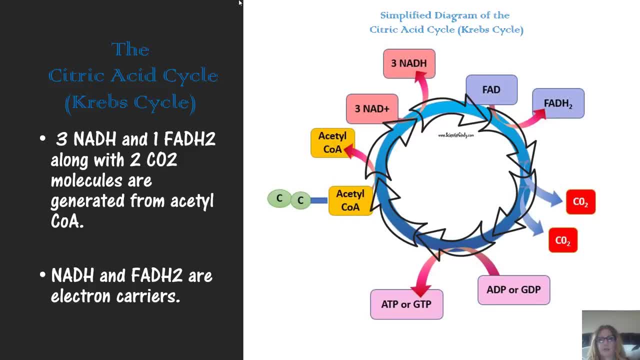 So here is my simplified diagram of the citric acid cycle, or Krebs cycle. So here I have the two-carbon acetyl-CoA entering the Krebs cycle from the side. I could have chosen anywhere. I don't know why I chose the side, but I did. 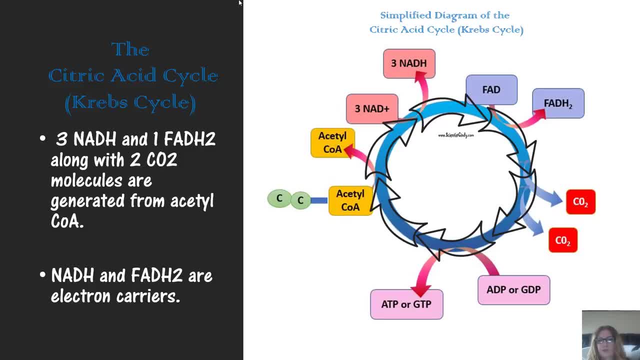 So there you have it. So these totals are actually per one acetyl-CoA. So if I have one acetyl-CoA going in here and just remember that this acetyl-CoA actually keeps getting regenerated during this process, So with one acetyl-CoA I generate three NADH, which are electron carriers. 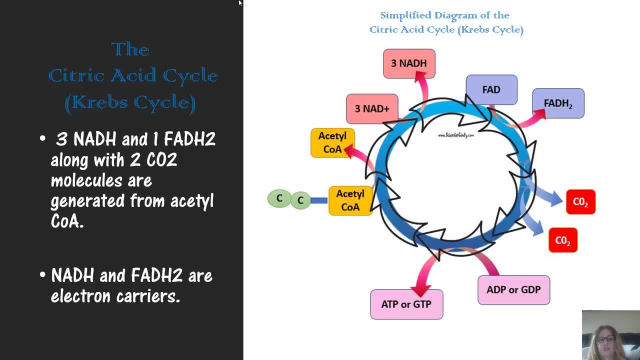 I generate one FADH2, which is another electron carrier. I'm going to generate carbon dioxide And then I'm going to generate an ATP or GTP, And GTP, just so you know, does the same job as ATP. 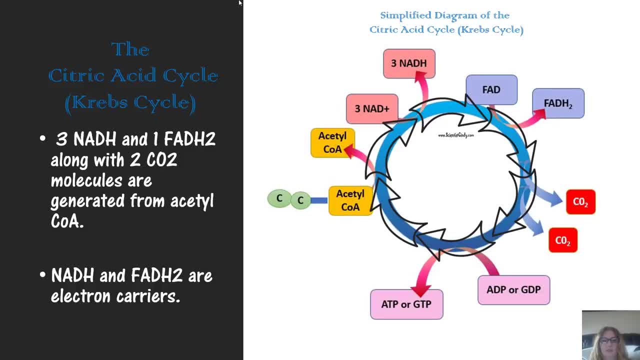 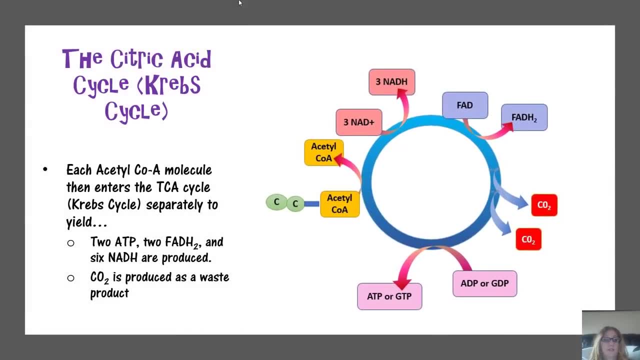 But for our sake we can just go ahead and stick to ATP. All right, So each acetyl-CoA molecule then enters the TCA cycle- Krebs cycle, separately. So we'll get two ATP, two FADH2, and six NADH per glucose molecule. 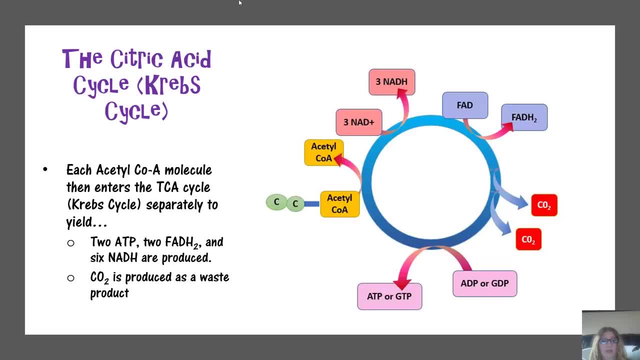 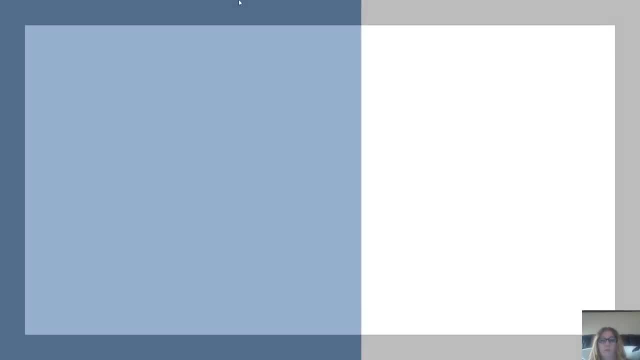 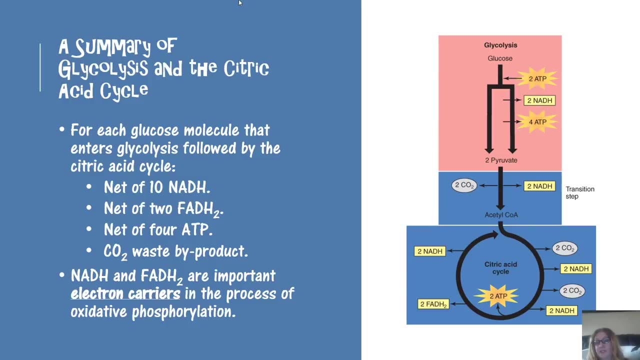 Per glucose molecule And then carbon dioxide is produced as a waste product. All right, So here is the summary of glycolysis and the transition step and the citric acid cycle per glucose molecule. Okay, per glucose molecule. So for each glucose molecule that enters glycolysis. 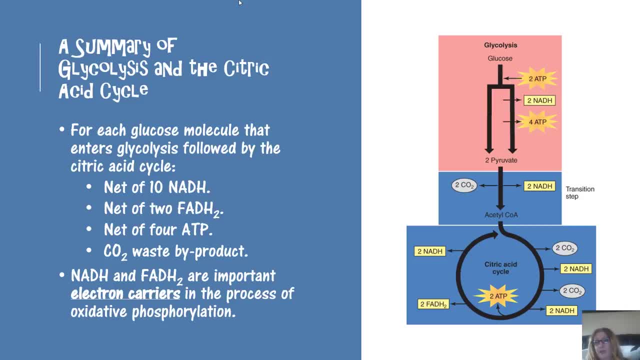 followed by the citric acid cycle. if we add this up so we get. so remember, at the beginning of glycolysis we use up two ATP but we end up making four ATP. so we get a net gain of two ATP in glycolysis. 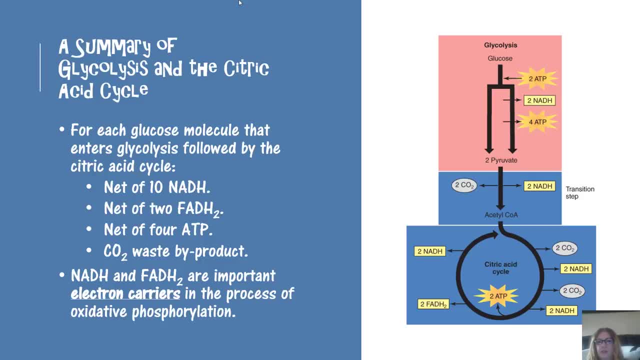 We also make two NADH during glycolysis. During the transition reaction, we make no ATP, But we do create two carbon dioxide molecules and two NADH molecules from one glucose molecule. One glucose molecule. we know that that is going to yield two pyruvates. 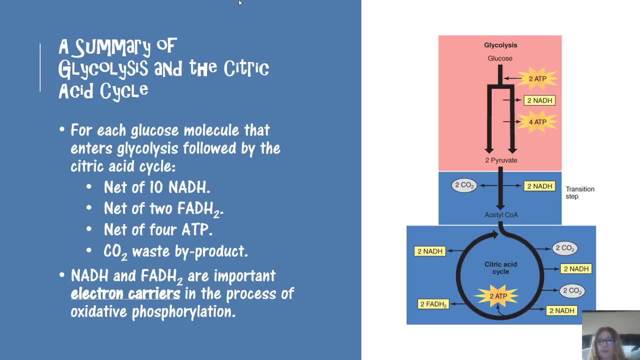 Two pyruvates gives us two acetyl-CoAs. So the diagram here is giving us all the totals for the entire glucose molecule. So we'll get two. in the citric acid cycle we will get two carbon dioxides, two NADH. 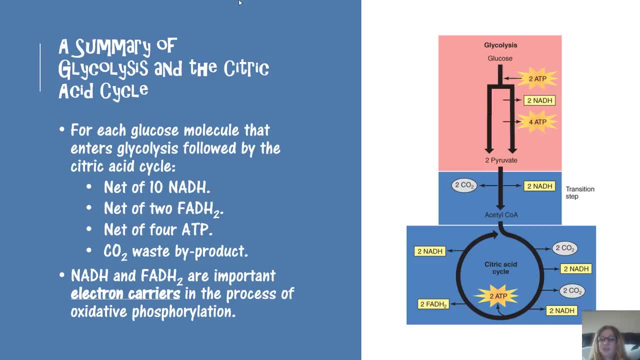 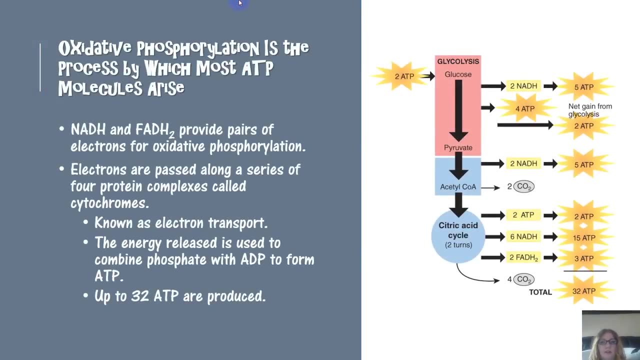 two more carbon dioxides, two more NADH, two more ATP, two FADH2,, which is another electron carrier, and two more NADH. So this is just another way to look at it. So here so this top part here in pink. 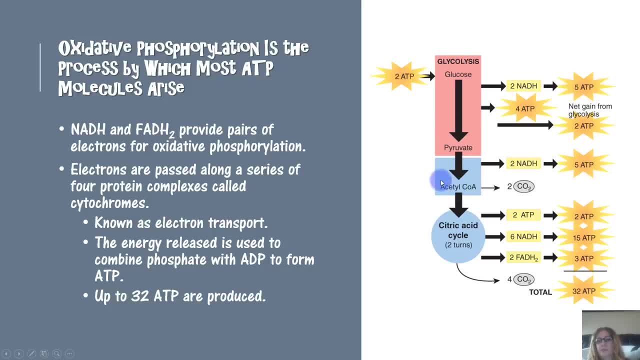 this is glycolysis. This blue middle part where it says acetyl-CoA is showing the transition reaction, And this circle at the bottom and it says two turns, because they're just reiterating that this is showing the totals for what would be. 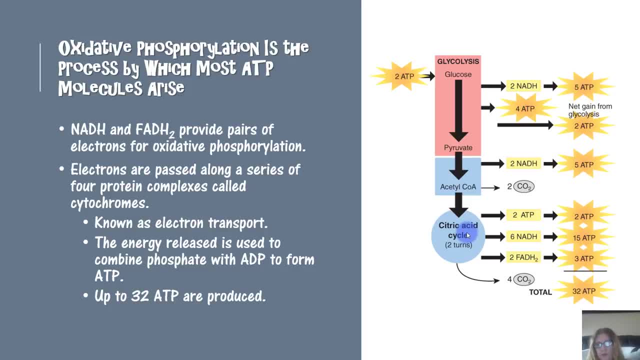 the entire breakdown of one glucose molecule. So this is one glucose molecule's worth, if you will, of what you would get out of it. So this would be two turns of the citric acid cycle, So both acetyl-CoAs of the glucose molecule. 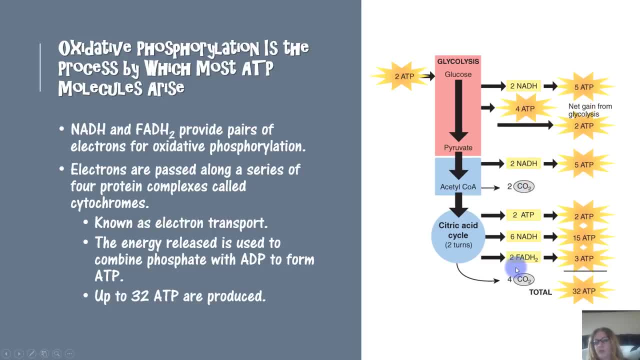 are being broken down And these are all of our outcomes. So we have two ATP at the beginning of glucose getting used, Four ATP coming out. So we have a net gain of two ATP. We have our electron carrier here getting generated. We have another electron carrier here getting generated. 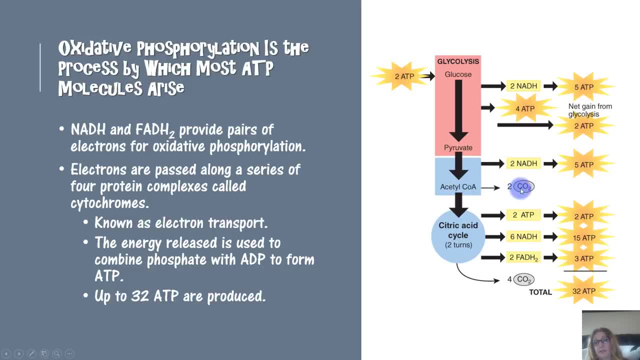 in the transition step We have some carbon dioxide, which is a waste product that we exhale from our bodies. It doesn't do anything for us. In the citric acid cycle we have two more ATP that are generated And then we have quite a few. 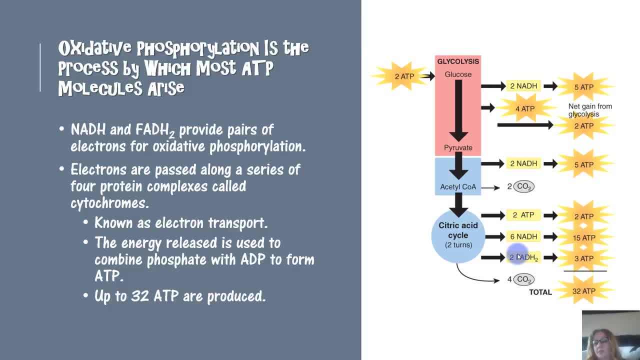 in the citric acid cycle. we actually have quite a few additional NADH, and we have some FADH2 also, which are additional electron carriers that are generated, And then some more carbon dioxide, which we exhale as a waste product. 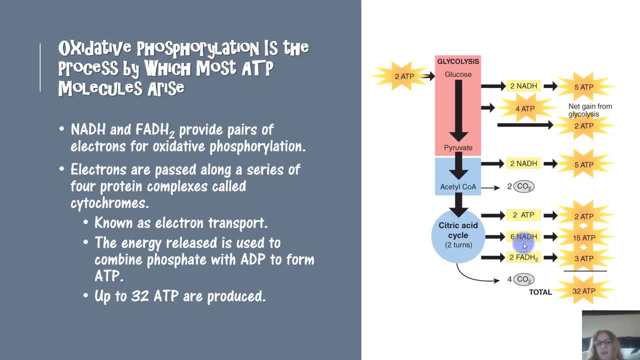 So what is the purpose of all of these electron carriers? So these electron carriers are going to carry electrons, hence the name- And they carry their electrons to the electron transport chain. So what this is showing here, in this last column, with all of these stars here. 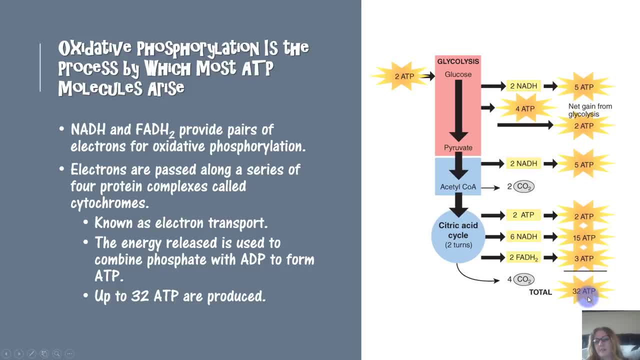 this is showing what the ATP that will be the final outcome, the predicted outcome for the gain of ATP that those electrons that these electron carriers that deliver to the electron transport chain will potentially produce in oxidative phosphorylation in the electron transport chain. Okay, 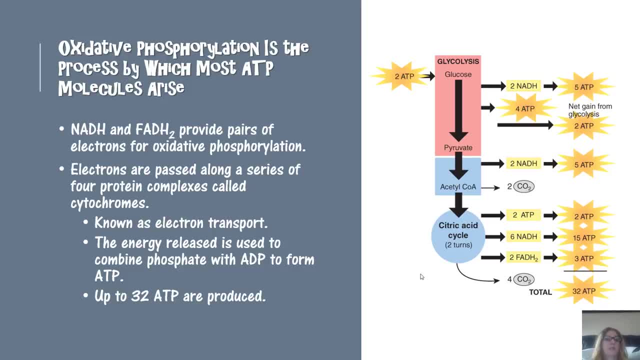 So let me elaborate on that Alright. So oxidative phosphorylation is the process by which most of the ATP molecules arise from cellular respiration. NADH and FADH2 provide pairs of electrons. for oxidative phosphorylation, Electrons are passed along a series of four proteins. 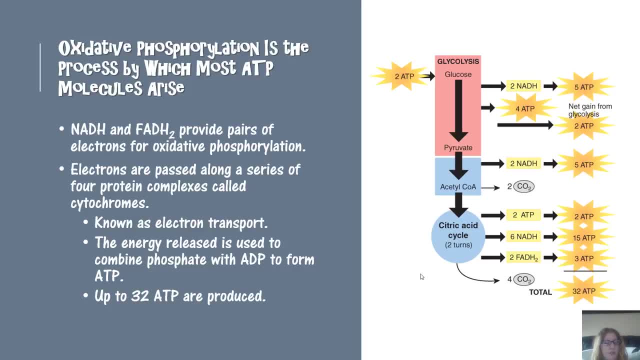 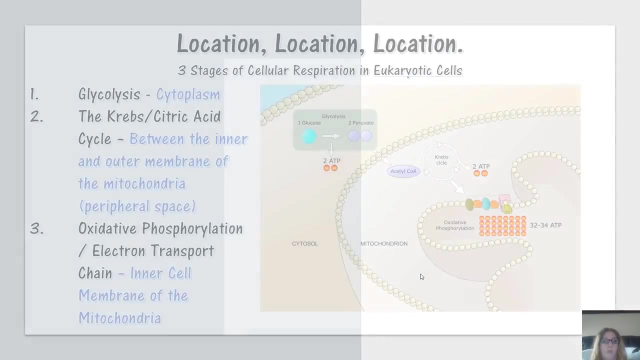 called cytochromes, And they're known as electron transports. The energy released is used to combine phosphate with ADP to form ATP, And up to 32 ATP are produced in that process. Okay, So let's take a moment to talk about location. 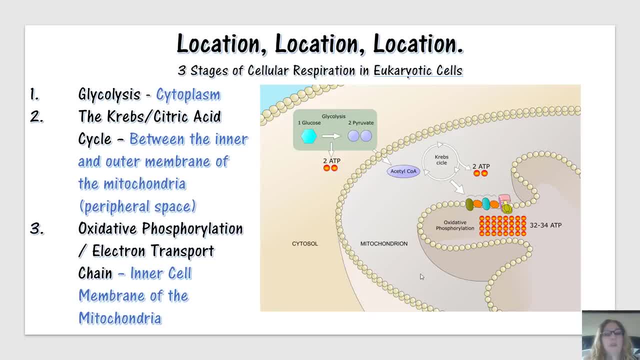 Okay, So the location is going to vary depending on whether we are in a prokaryote, such as a bacteria or an archaea cell, or if we are in a eukaryotic cell. So location, location, location. So let's look at the three stages of cellular respiration. 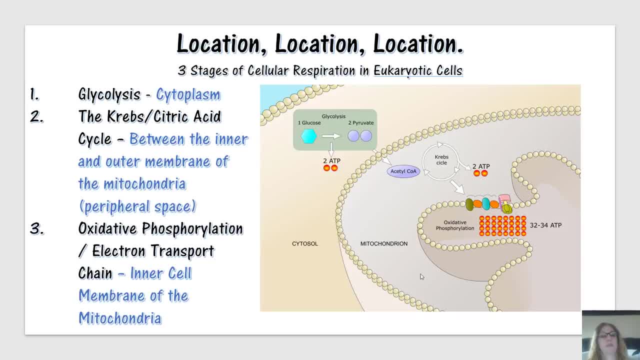 and let me define where those different stages take place. In a eukaryotic cell, glycolysis is going to take place in the cytosol or in the cytoplasm, Just so you know, in prokaryotes in the next slide. 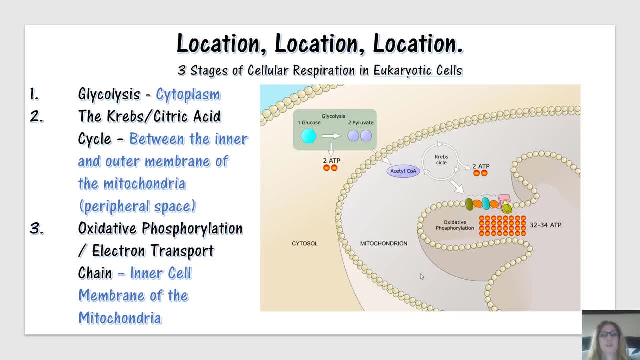 you'll notice that that is also the same. So eukaryotes and prokaryotes both have the location of glycolysis will take place in the cytoplasm. You could also say cytosol, Which is just the intracellular fluid. 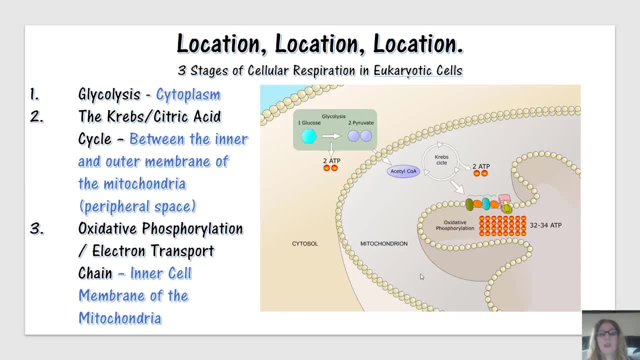 That would also be correct. Okay, For the Krebs cycle or citric acid cycle in eukaryotic cells, this will take place between the inner membrane and outer membrane of the mitochondria. Now, this area between the inner and outer membrane of mitochondria. 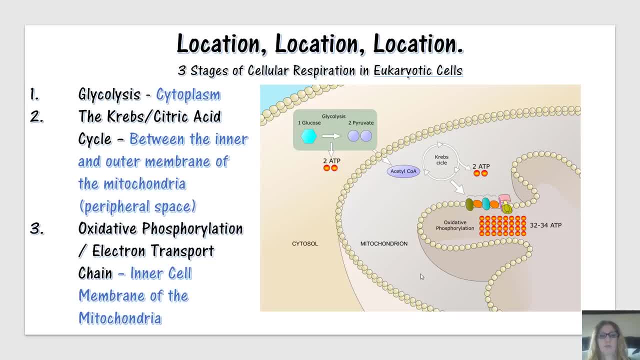 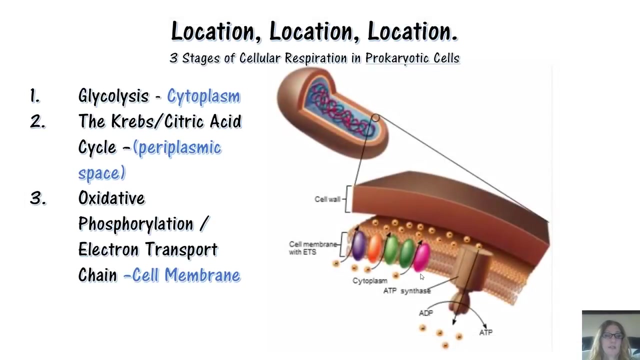 is called the peripheral space. The peripheral space, Then the final stage of cellular respiration, called oxidative phosphorylation or the electron transport chain, will take place in the inner membrane of the mitochondria Versus looking at the prokaryotic cell, Glycolysis will still take place in the cytoplasm. 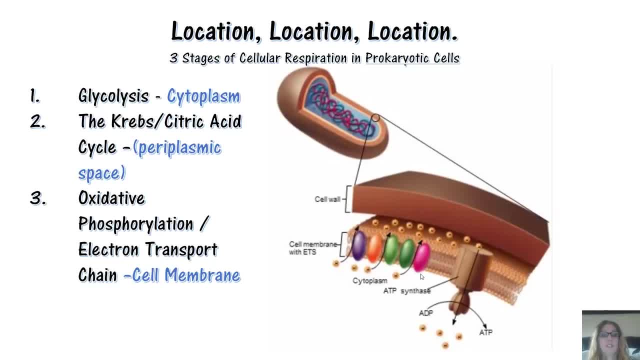 just like in eukaryotic cells. But when we get to the Krebs cycle or citric acid cycle, that is going to take place in what is called the periplasmic space. The periplasmic space is the space between the cell wall. 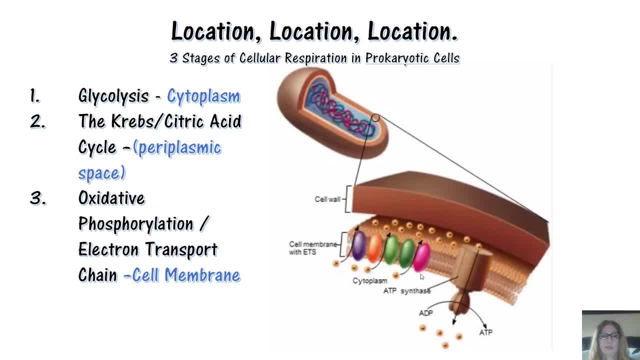 and the cell membrane of the prokaryotic cell. We also have oxidative phosphorylation and the electron transport chain that occurs in prokaryotic cells And that is going to occur in the inner cell membrane of the prokaryotes. So prokaryotes do not have mitochondria. 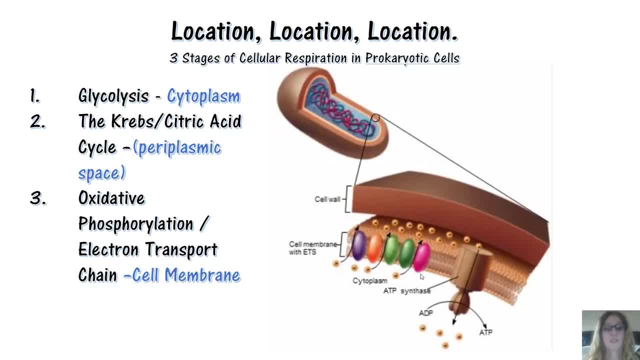 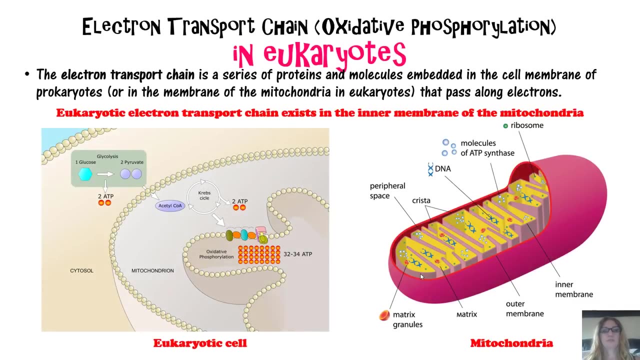 In a sense, you can kind of think of them as they are mitochondria. We believe that our mitochondria probably evolved from prokaryotic cells, So you can kind of think of it like that. Alright, So electron transport chain or oxidative phosphorylation. 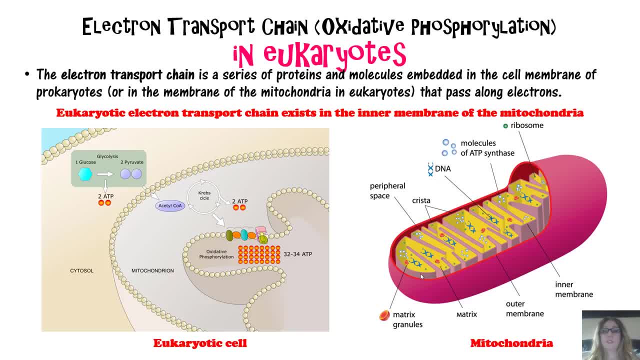 in eukaryotic cells. The electron transport chain is a series of proteins and molecules that are embedded in the cell membrane of prokaryotes or in the membrane of the mitochondria in eukaryotes, And what they do is they pass along electrons. 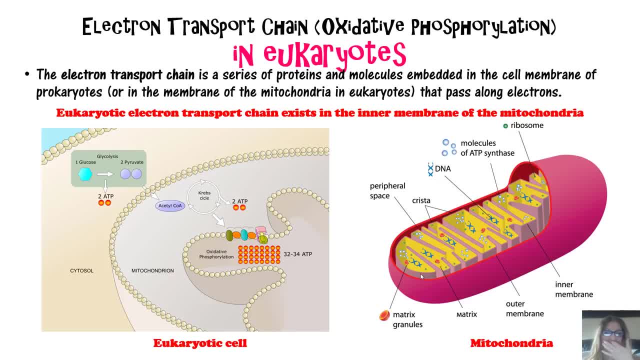 So the eukaryotic electron transport chain exists in the inner membrane of the mitochondria. Here I have a blowup of the mitochondria And here you can visualize the inner membrane of the mitochondria and the outer membrane of the mitochondria. 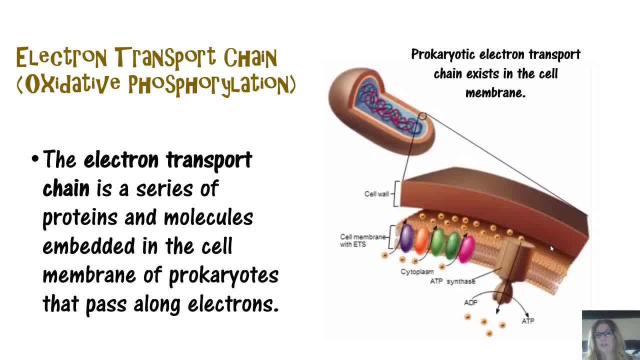 And the electron transport chain in the prokaryote. And you can see here the series of proteins and molecules are embedded in the membrane of the prokaryote And they are passing along electrons. So prokaryotic electron transport chains exist in the cell membrane. 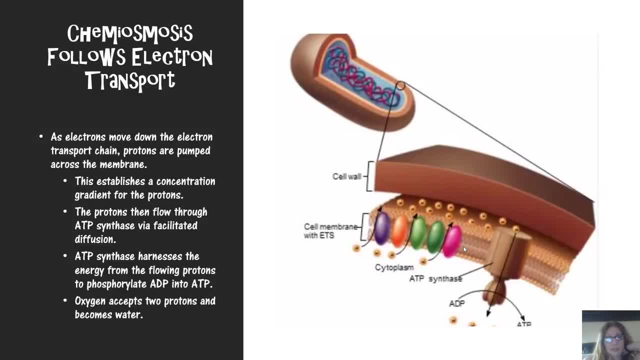 Okay, So let me introduce the concept of chemiosmosis and electron transport. So, as electrons move down the electron transport chain, protons are pumped across the membrane. This establishes a concentration gradient for the protons. The protons then flow through the ATP synthase. 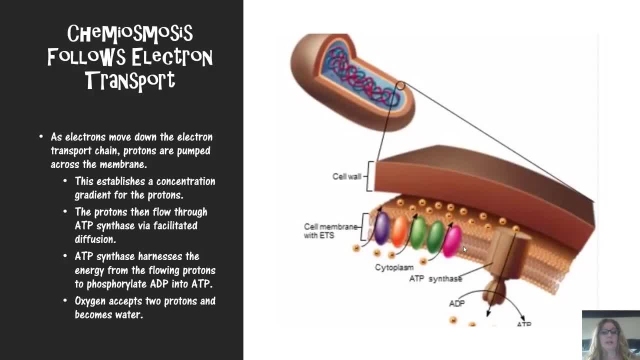 which is shown here, And it does this through what we call facilitated diffusion. So ATP synthase then harnesses the energy from the flowing protons And it will use that energy to phosphorylate ADP into ATP. Oxygen is going to be the final, or terminal, electron acceptor. 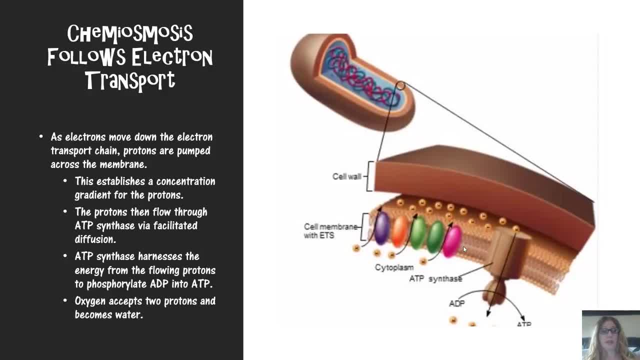 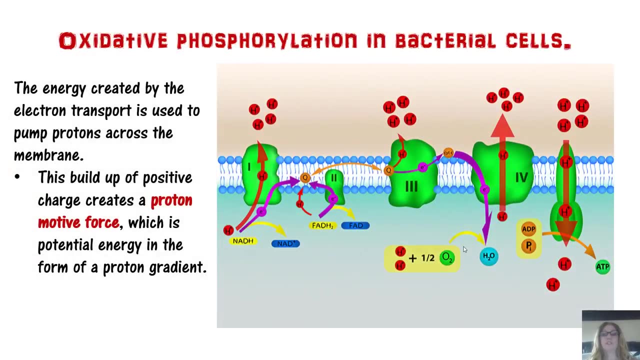 in the electron transport chain. Oxygen accepts those electrons and it will actually become water. So let's zoom in so we can get a better picture. Let's get a better look at what's going on here. All right, So this is the electron transport chain. 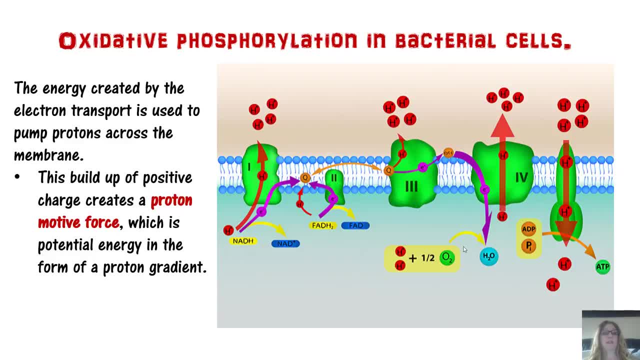 And we're zooming in. So the energy created by the electron transport chain is used to pump protons across the membrane. The buildup of the positive charge creates a proton motive force, which is the potential energy in the form of a proton gradient. 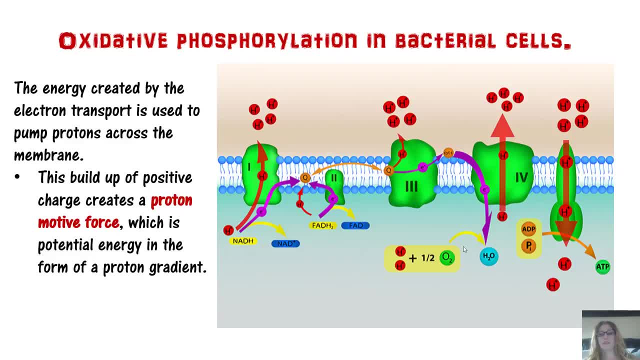 Okay, So we're splitting up the positive and negative charges. So I'm going to have this buildup of positive charge in the periplasmic space of our prokaryotic cell. Okay, That's going to be building up a proton motive force. 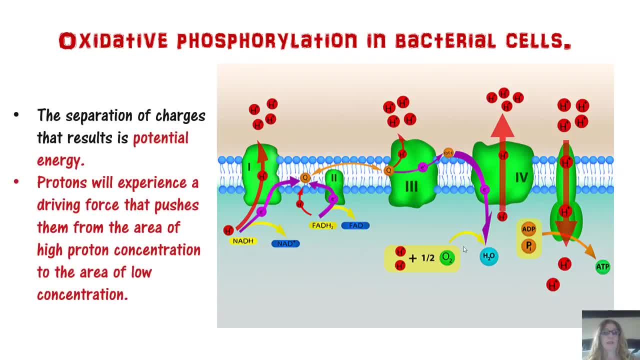 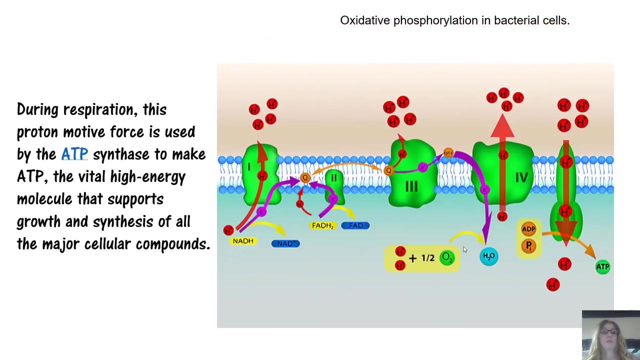 that can be used. The separation of charges that results is a potential energy Protons will experience a driving force that is directing them to want to go from the area of high proton concentration to the area of low concentration. So during respiration, this proton motive force, 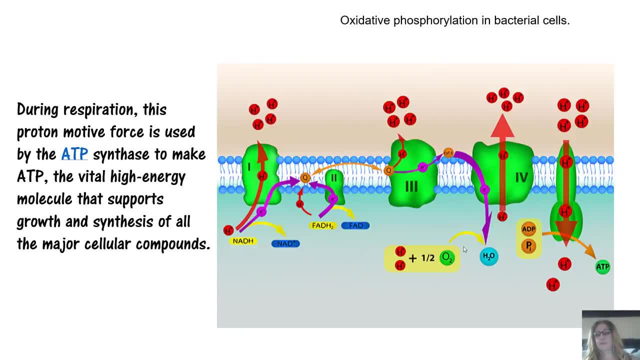 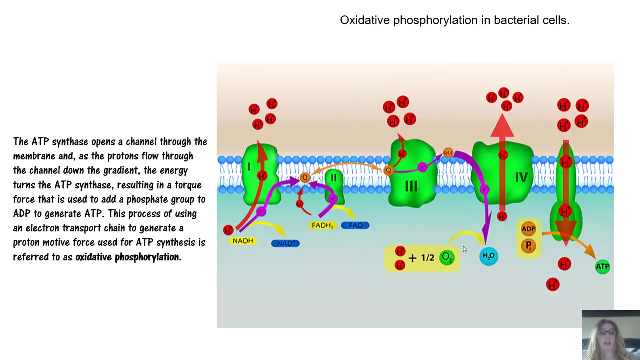 is used by the ATP synthase, which is the last structure here to make ATP the vital high energy molecule that supports growth and synthesis of all major cellular components. The ATP synthase opens a channel through the membrane and allows the protons to flow through. 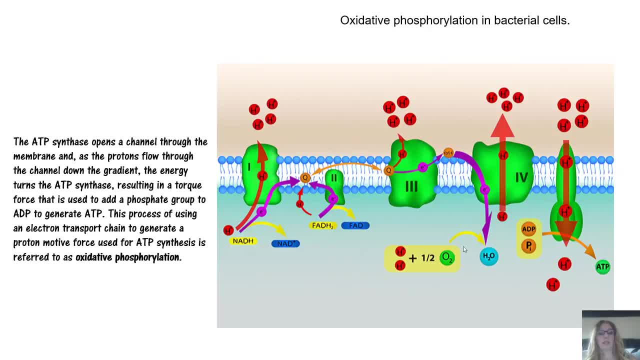 down its own electrochemical gradient, or proton gradient. The energy then turns the ATP synthase, resulting in a torque force. So it actually turns, physically turns the ATP like a little motor, And this torque force, or turning force, is used to add a phosphate group to ADP. 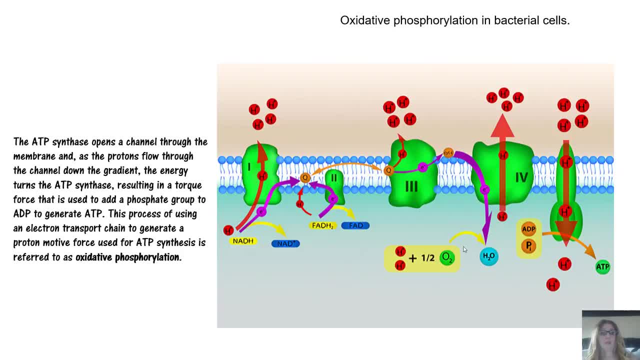 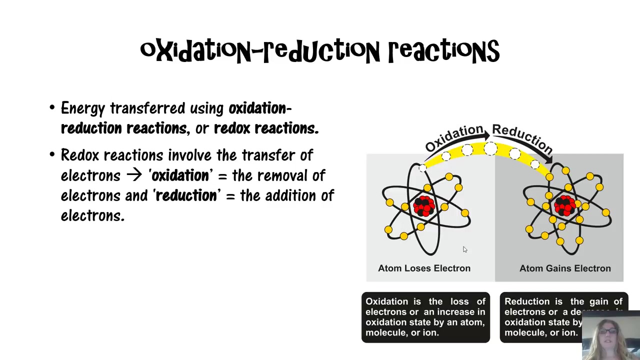 to generate ATP. The process of using an electron transport chain to generate a proton motive force used for ATP synthesis is referred to as oxidative phosphorylation. Okay, And since we're talking about oxidation reduction reactions on occasion, let me go ahead and give you my acronym. 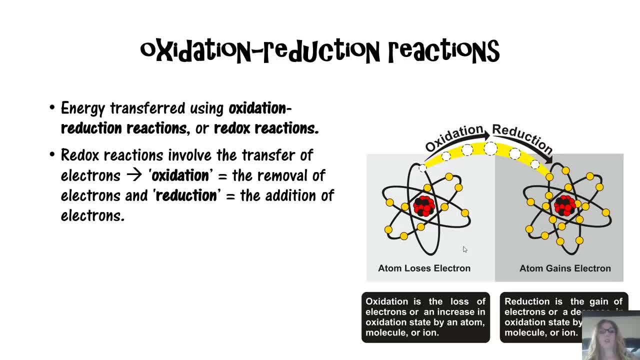 to remember oxidation reduction reactions, otherwise known as redox reactions. So the easiest way to think of it is that LEO says GER. So what do I mean by LEO says GER? So LEO means loses electron. wait, LEO loses electrons, is oxidized. 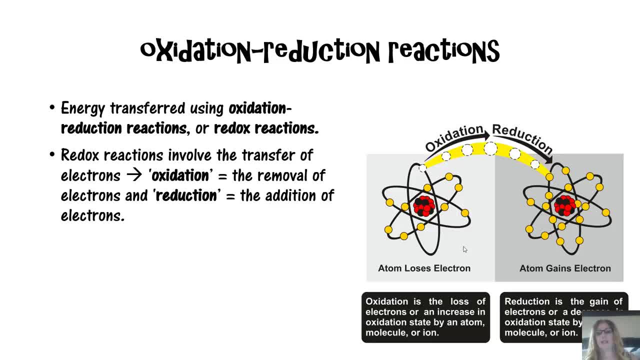 and GER is gains electrons is reduced. So LEO says GER like Leo the lion, So LEO is loses electrons oxidizes, GER is gains electrons is reduced. Okay, So when we're talking about something being oxidized, 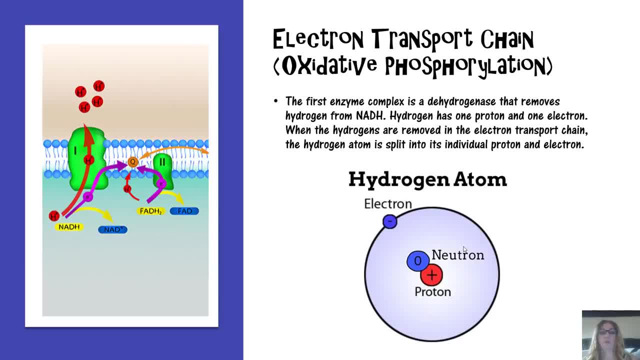 just think about it, as electrons are being removed. Okay, All right. So let's go a little bit deeper again into the electron transport chain. So, layer by layer going a little bit deeper. Okay, So the electron transport chain again. 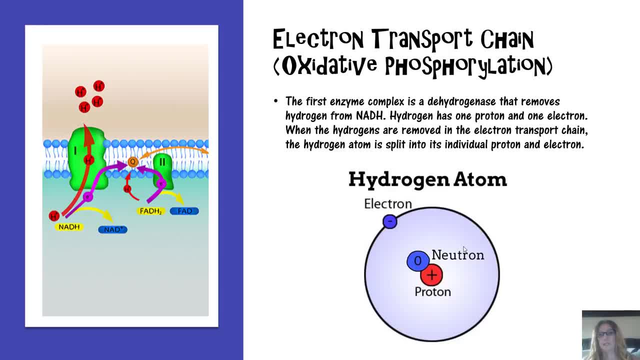 So the first complex here, the first enzyme complex, is a dehydrogenase. This dehydrogenase functions to remove hydrogen from NADH. Okay, Now, hydrogen has one proton and one electron, So when the hydrogens are removed, 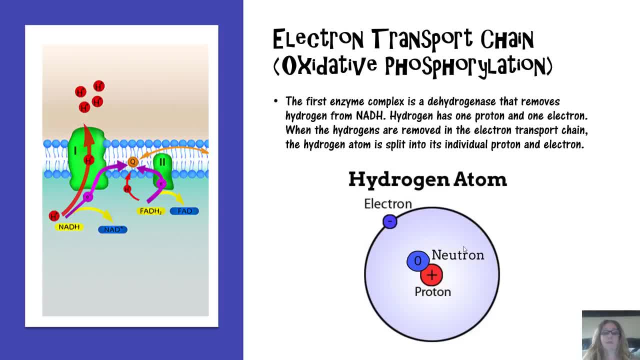 in the electron transport chain. what is going to happen is the electron is sorry. when hydrogens are removed in the electron transport chain, the hydrogen atom is split into its individual proton and electron. Those are the protons, And here in purple in this diagram. 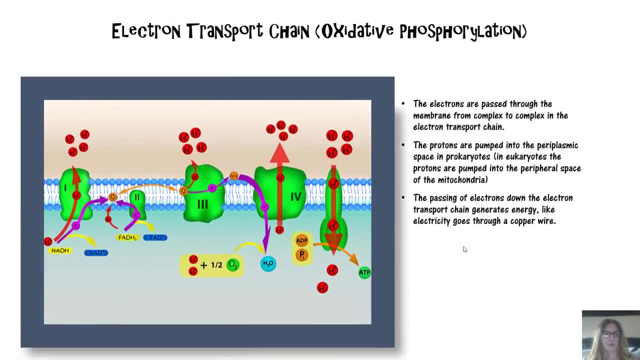 here in purple we have where the electrons are, So we can follow where the electrons are. So the electrons actually stay in that membrane as they're being passed from complex to complex. The protons are the ones that are actually being pumped across. 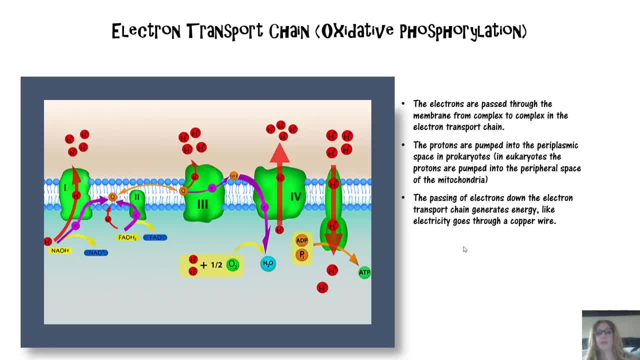 the membrane. Okay, The electrons are passed through the membrane from complex to complex. in the electron transport chain, The protons are pumped into the periplasmic space in prokaryotes. In eukaryotes, the protons are pumped into. 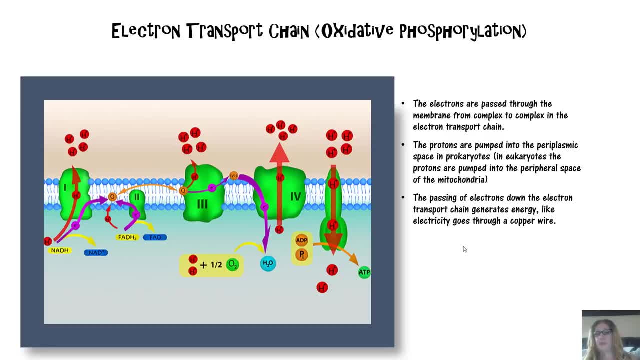 the peripheral space of the mitochondria. The passing of electrons down the electron transport chain generates energy, like electricity going through a copper wire, for example. The terminal oxidase is complex IV, So that's the last one in line. It is a proton pump that transfers the electrons to oxygen. 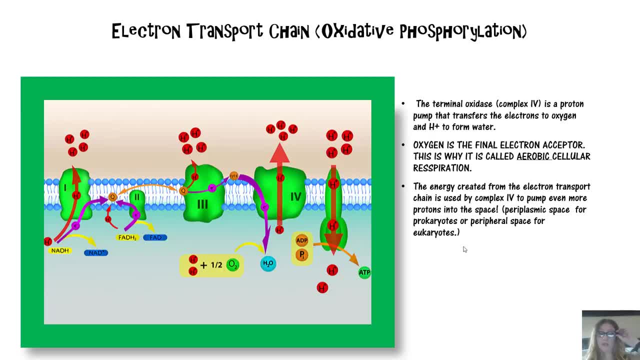 Okay, So oxygen is our final electron acceptor or our terminal electron acceptor, which is why, if that is the case, that will be considered aerobic cellular respiration, meaning, with oxygen, Okay, The energy created from the electron transport chain. 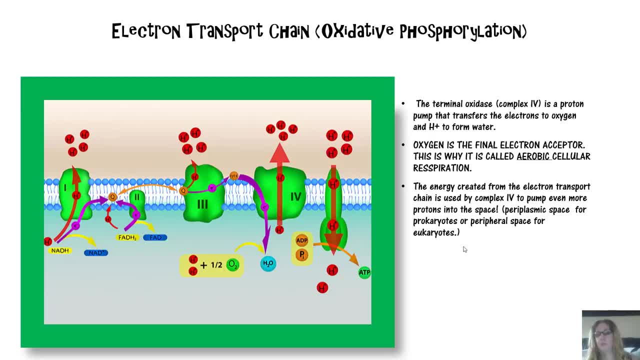 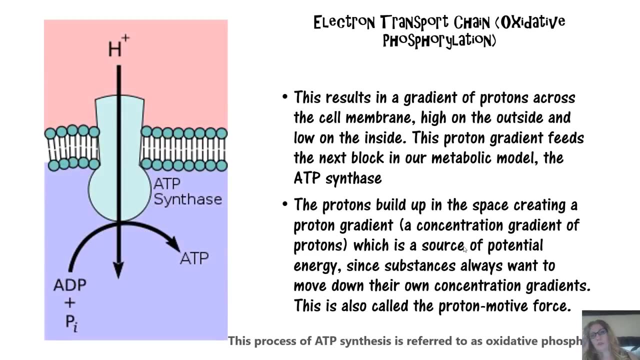 is used by complex IV to pump even more protons into the periplasmic space for prokaryotes or peripheral space for eukaryotes. All right, So all of this proton gradient, what is the point of it? So this results in a gradient of protons. 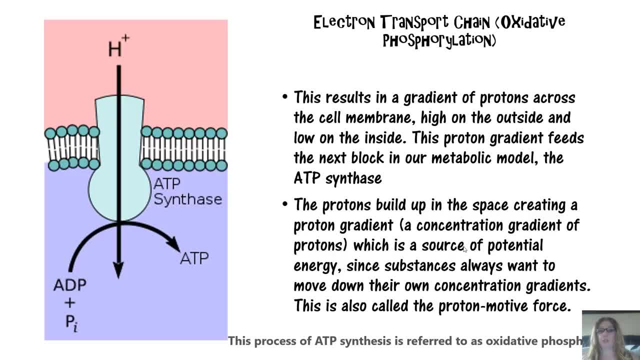 across the cell membrane, high on the outside, low on the inside. This proton gradient feeds the next metabolic model, or the next figure, which is the ATP synthase. Okay, So the ATP synthase is going to harness this potential energy of the proton motive force. 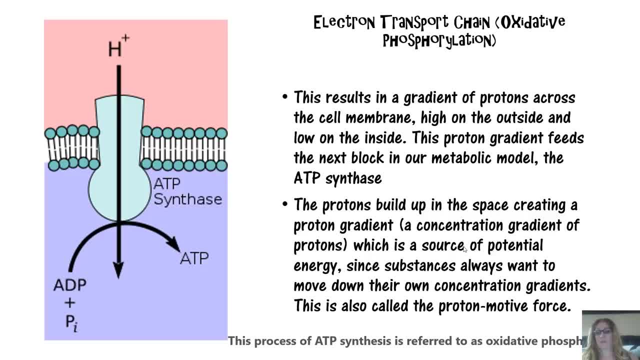 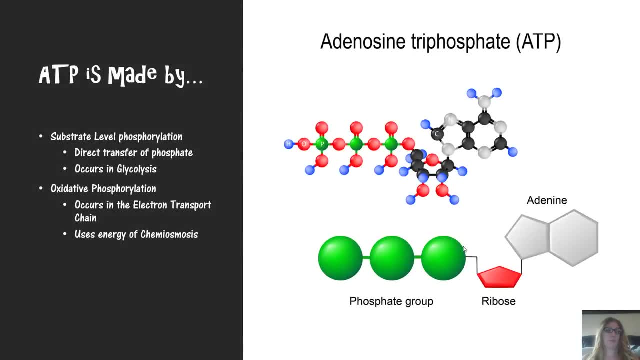 The protons build up in the space, creating the proton gradient, which is a source of potential energy, since substances always want to move down their own concentration gradients, called the proton motive force. Okay, So adenosine triphosphate is the real name of ATP. 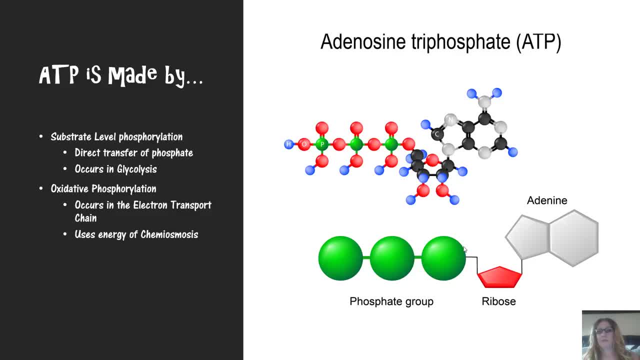 And here we see the structure of ATP. Okay, So ATP is. I just noticed that it says adenine. huh Huh, interesting. So it's actually adenosine triphosphate. So it's adenosine triphosphate. 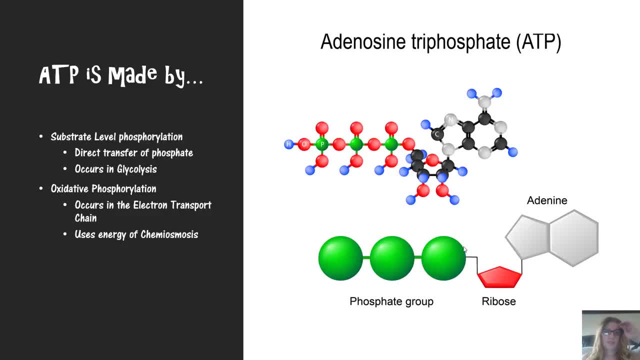 And here we have three phosphate groups. So ATP is actually made by two different mechanisms. Okay, So ATP is made by substrate level phosphorylation during glycolysis, which is the direct transfer of phosphate from one molecule to another, And in the electron transport chain. 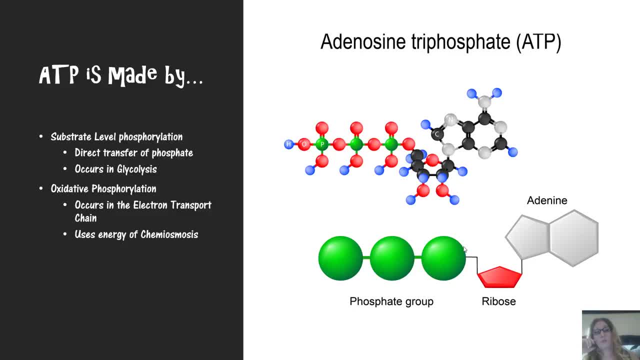 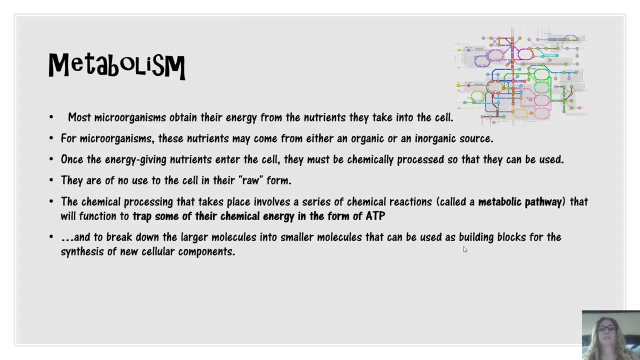 we have ATP being made by the process of oxidative phosphorylation. Oxidative phosphorylation uses the energy of the proton motive force. We call that the energy of chemiosmosis. Okay, So now that we have our foundation, let's go ahead and 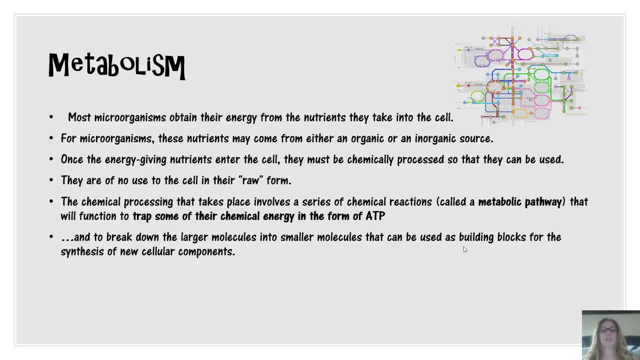 look at the much bigger view. So a lot of us go through our high school biology years and beginning biology and think that, oh well, that's all there is. All we do is just metabolize glucose and that's it. Au contraire, 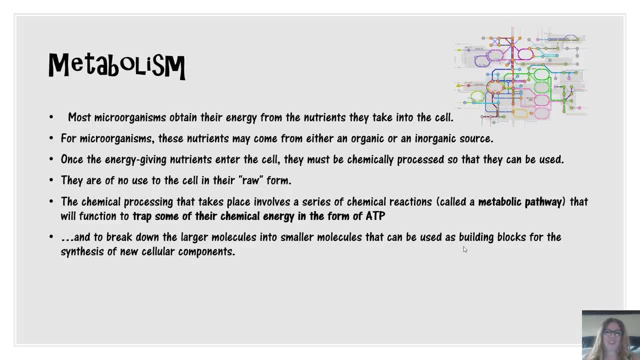 So there's so, so, so much more out there. We are just going to barely scratch the surface in this course, But hopefully at least I'll be able to open your eyes to a lot of other- at least other- possibilities. 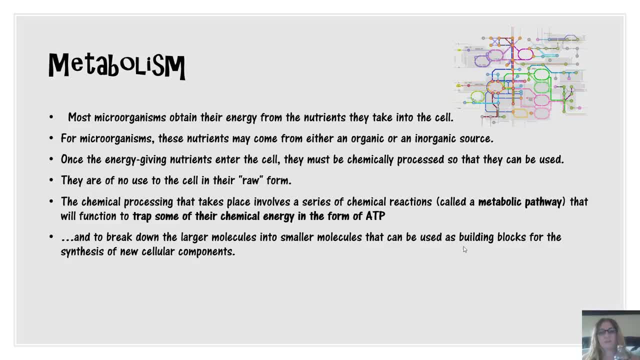 that are out there. It's so much more diverse than I can even begin to explain. So most microorganisms obtain their energy from nutrients that they take into the cell. For microorganisms, these nutrients may come from either organic or inorganic sources. 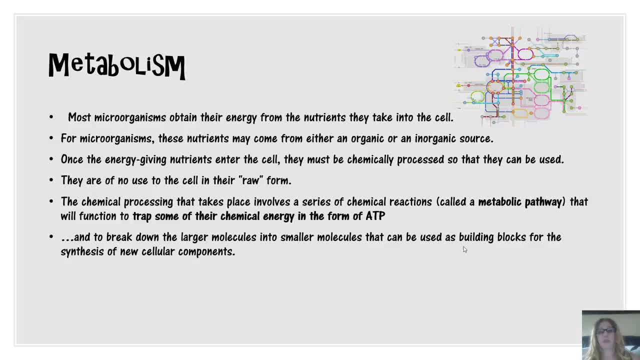 Once the energy-giving nutrients enter the cell, they must be chemically processed so that they can be used. They are of no use to the cell in their raw form. The chemical processing that takes place involves a series of chemical reactions called a metabolic pathway. 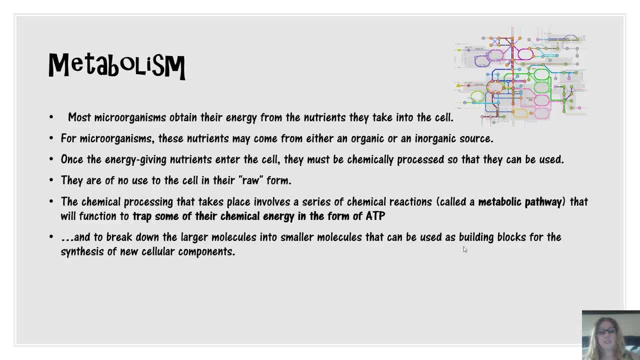 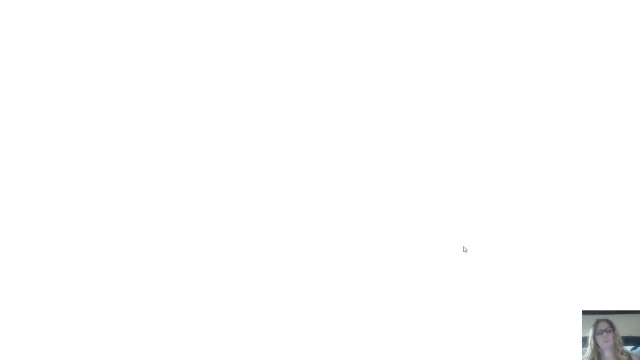 This metabolic pathway functions to trap some of the chemical energy in the form of ATP. Also, metabolic pathways will function to break down larger molecules into smaller molecules that can be used as building blocks for the synthesis of new cellular components. So living organisms must synthesize polymers. 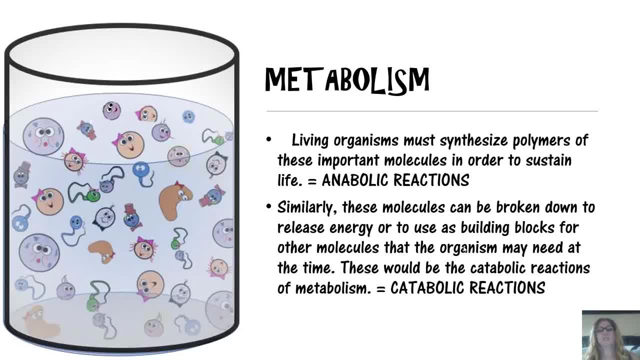 of these important molecules in order to sustain life. This would be an example of anabolic reactions. Similarly, these molecules can be broken down to release energy or to use as building blocks for other molecules that the organisms might need at the time. These would be considered. 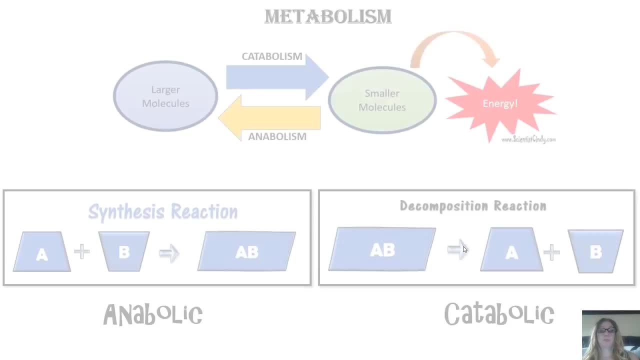 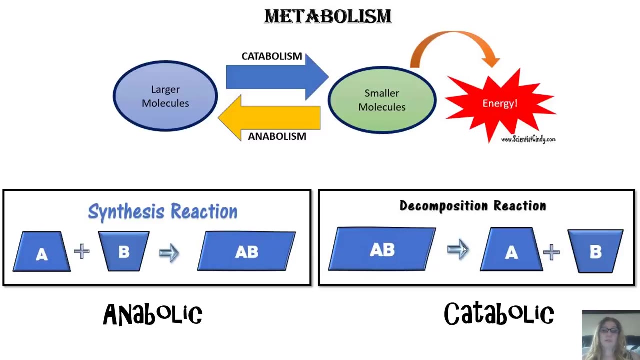 the catabolic reactions of metabolism. When we talk about metabolism, metabolism is actually defined as all of the chemical reactions going on within the organism. This includes everything that is being broken down as well as being built up, So this includes chemical reactions. 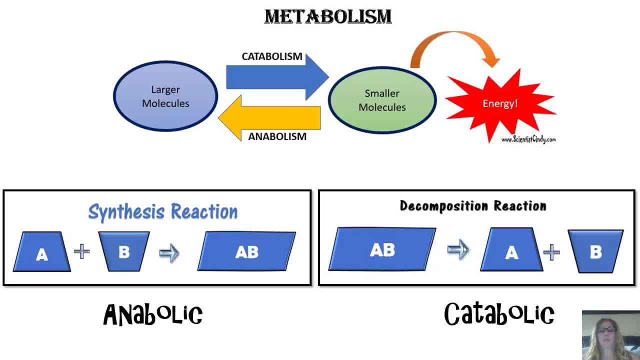 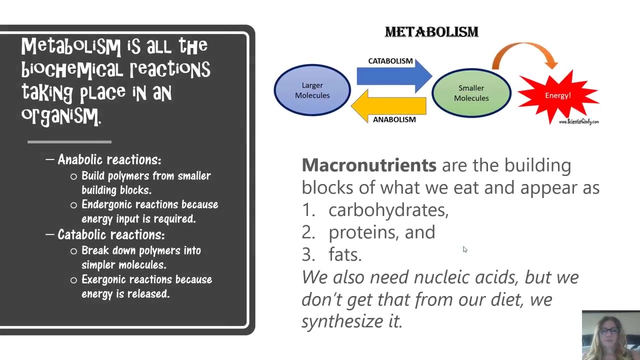 that are going to be synthesis reactions, which are building bonds and creating larger molecules out of smaller molecules, or decomposition reactions, where I'm taking larger molecules, breaking them down, breaking bonds so that I can get smaller molecules. So when we talk about these building blocks- 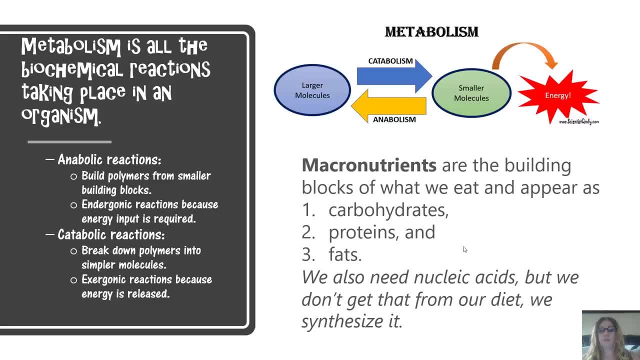 we get these building blocks from our food. What building blocks do we need? Well, we need four things really: We need carbohydrates, we need proteins and we need fats and we also need nucleic acids, But we don't get nucleic acids. 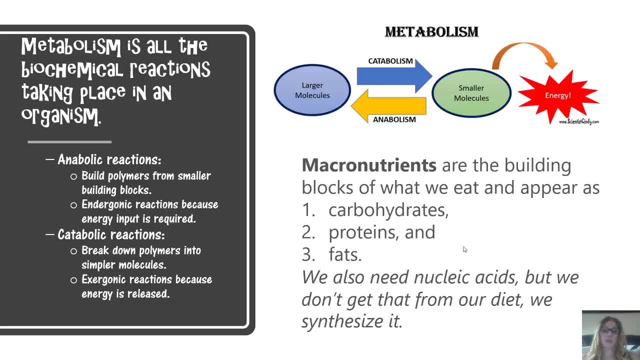 from our diet, We synthesize them in our bodies. So metabolism is all of the chemical reactions taking place in an organism. The anabolic reactions are going to build polymers from small building blocks, and when we do that, those are called endergonic reactions. 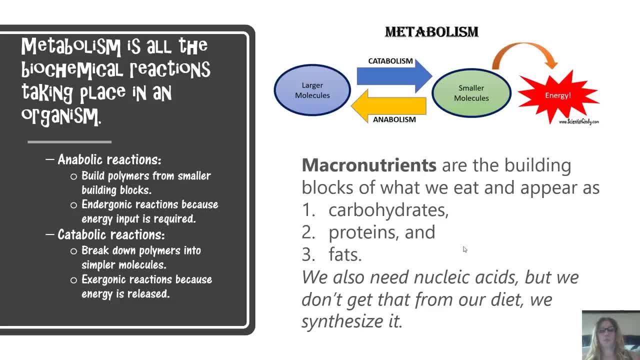 The reason they're called endergonic reactions is because energy is required for those reactions. So endergonic means energy has to be put in. Catabolic reactions means that you're breaking down a polymer. you're taking a larger molecule, breaking it down into a smaller molecule. 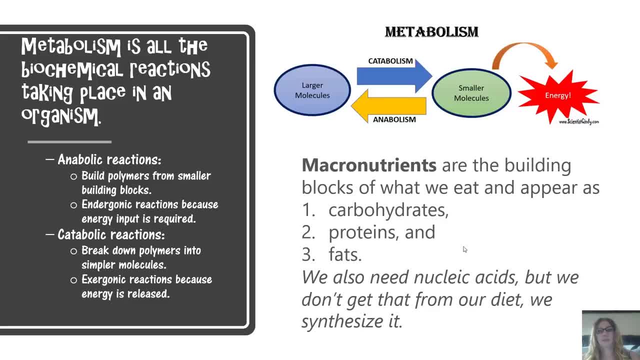 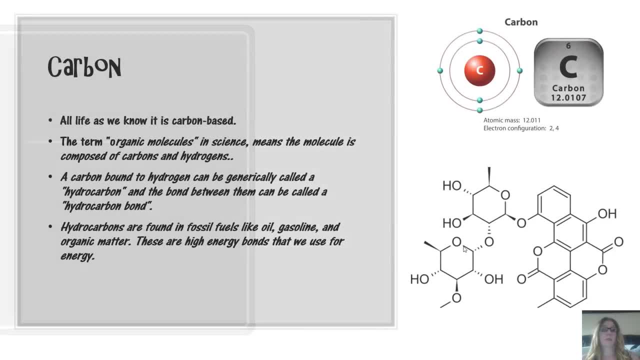 This would be an exergonic. an exergonic reaction. You're breaking a bond and energy is being released. So all life as we know it on planet earth is carbon based. Now, when you go to the grocery store and you see the sign that says: 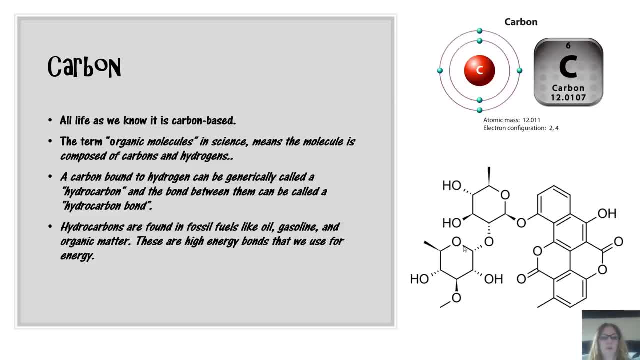 organic, organic bread or organic vegetables. that means something very, very different than what it means in science. Now, when we talk about organic molecules, organic chemistry, it means something very, very different. So when we talk about organic, we're talking about it having a lot of carbon. 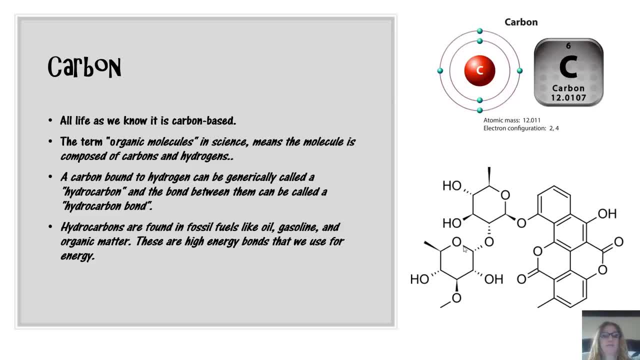 and hydrogens. So, in other words, if it has just hydrogen carbons, it's a hydrocarbon, Like a fossil fuel, for example. Those are hydrocarbons. Why are hydrocarbons so sought after? Because they have energy, Our energy sources. 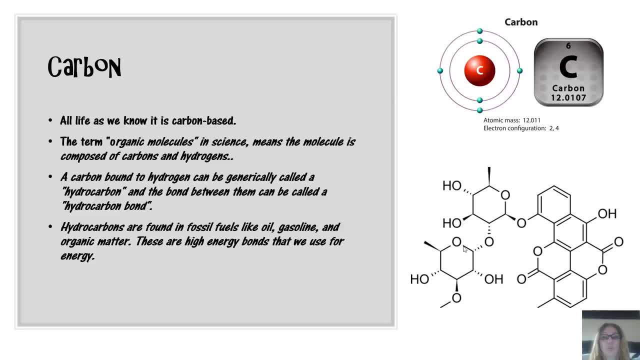 not only of our body but of the world. we're getting better with utilizing alternative energy sources, But when you look at history, there's a lot of fossil fuel use. We've used hydrocarbons for a very, very long time as a source of 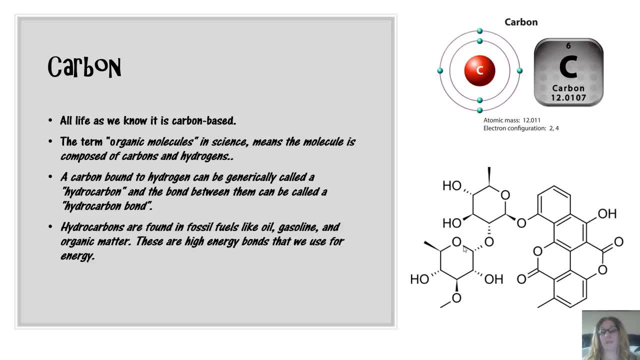 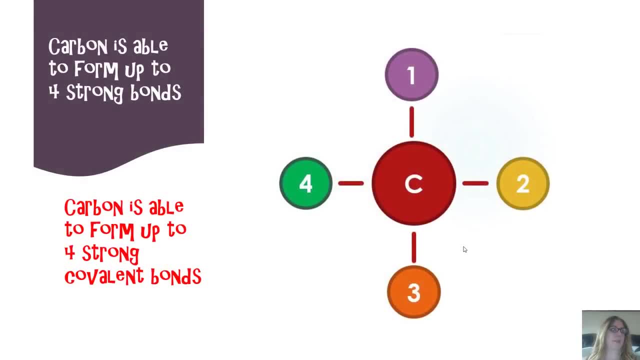 energy. So you can kind of think of it as that's what biological entities also do. So what is the big deal? Why carbon? What's the big deal of carbon? Well, carbon is very unique. It is the only element capable. 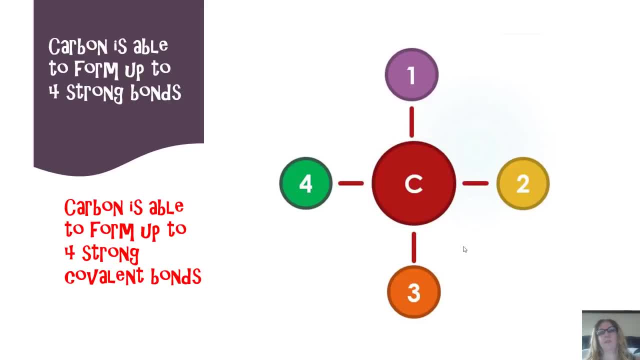 of building four strong covalent bonds with up to four different atoms or molecules. So if you do the math, what this means is that there's more flexibility, There's more arrangements, There's more different things that you can make with carbon. 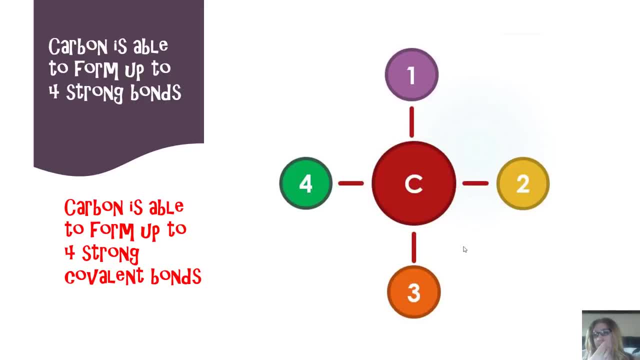 There are larger macromolecules that you can make, Long fatty acid chains that you can make, for example, Large aromatic rings, Different configurations, like we see with diamonds, for example. There's just all sorts of configurations that you can make with carbon that you just 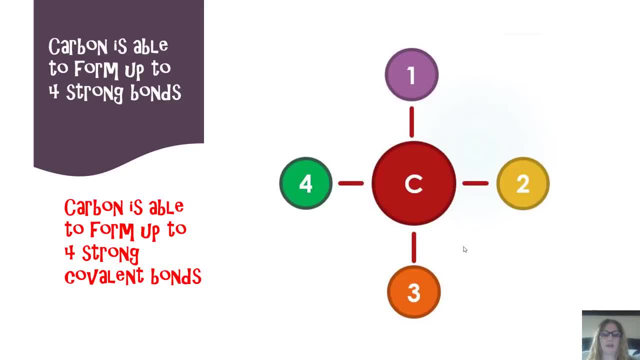 can't really make in a stable form with other elements. Now, now you might be thinking, well, wait a minute. There are other things in that same group that, sorry, hold on a second. So you might be thinking that 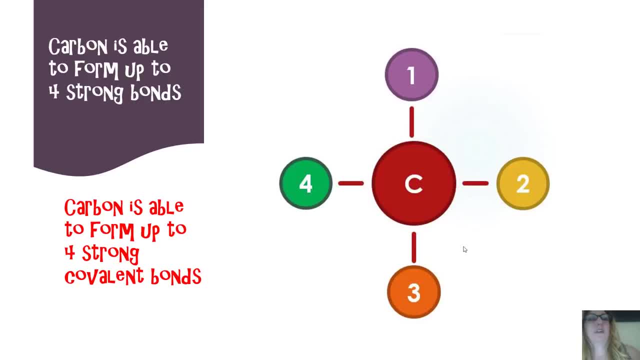 that there are other elements in that same group and anything in that group is going to be able to make four bonds, And you're right. However, carbon is in the How's that Okay? So the electron shell? that is because remember. 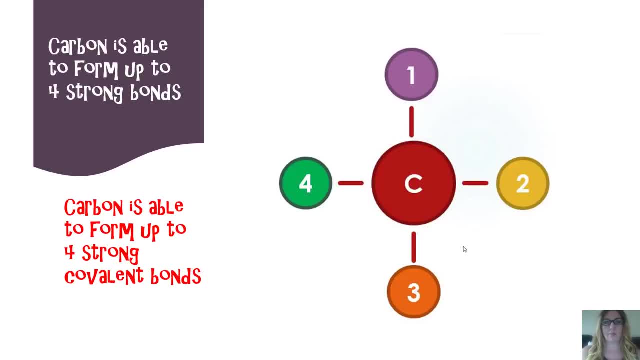 that it's only the electrons in the outer shell that can make bonds. So as you continue down the periodic table, the electrons available for bonding are going to be further and further away from that positively charged nucleus. What that means is, even though we have 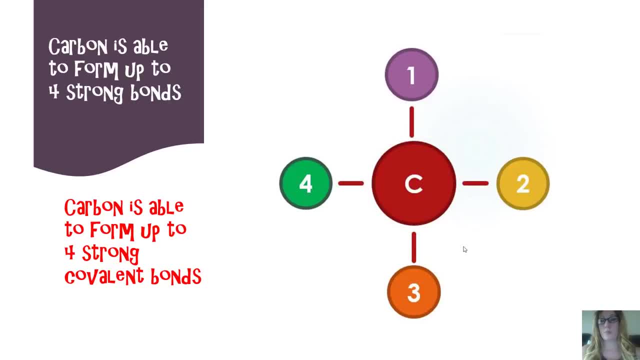 other elements that can make four bonds, they will not be as strong because they're further away from the nucleus, So that's why it's unique. So you really have to say that not only is it able to make four bonds, but it makes four. 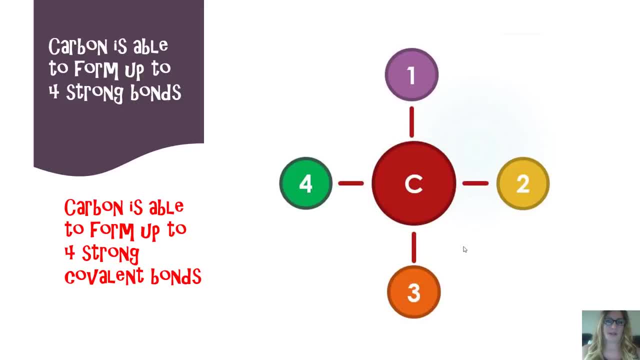 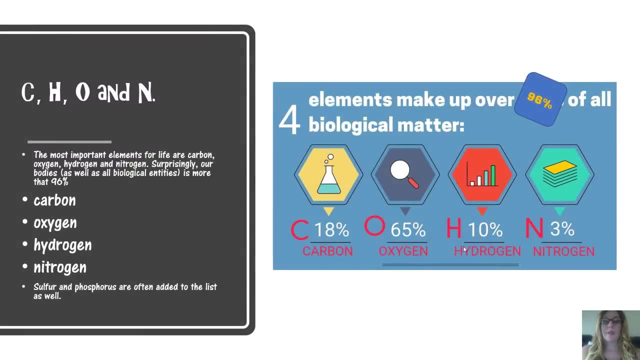 strong covalent bonds, And that is what makes it unique. Okay, Alright. So surprisingly, about 96% of all living matter is made up of just simply carbon oxygen, hydrogen and nitrogen, And sulfur and phosphorus come in at a very close. 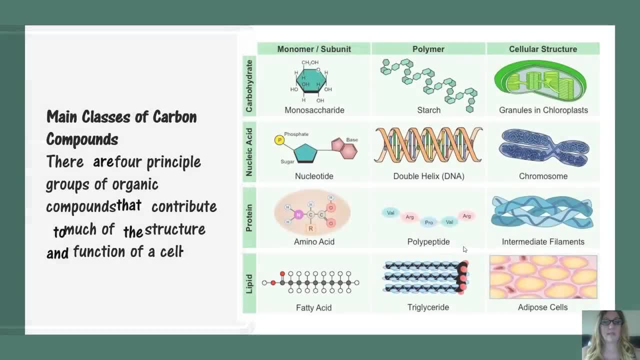 second to these. So it's pretty amazing that we can get such a wide variety of our macromolecules and cellular components with so few elements. So there are actually four principal groups of organic compounds that contribute to almost all of the structures of the cell, And those 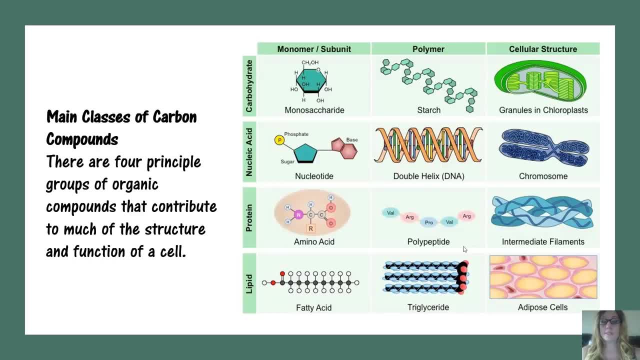 go back to again our carbohydrates, our nucleic acids, our proteins and our lipids once again. So let me just give you some terminology. So, when we are looking at our cellular components and a lot of these macromolecules, 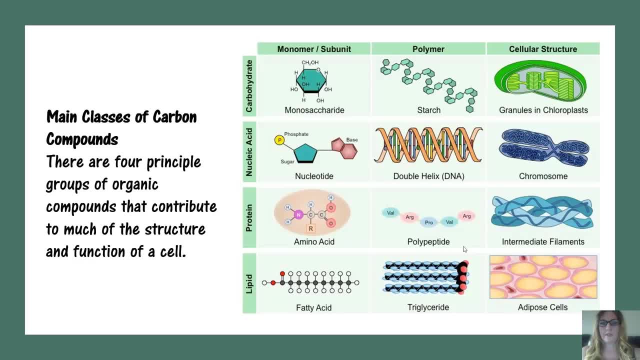 inside of the body we have a lot of these macromolecules are polymers. Now, a polymer is a general term. that just means that it's a large molecule that's made up of individual subunits that repeat. Now, the individual subunits that repeat. 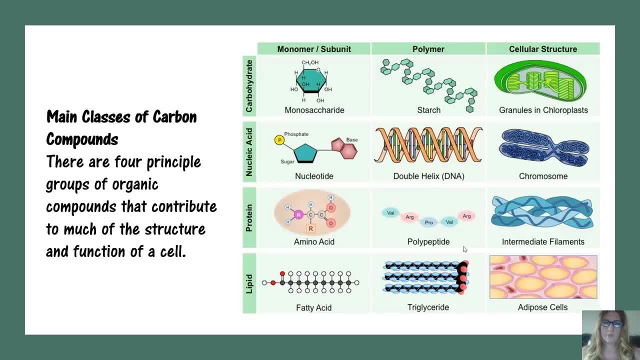 are referred to generically as monomers. So let's take a carbohydrate as an example. If you have a carbohydrate which is a sugar, if you have just one single unit, we call that a monosaccharide or a simple. 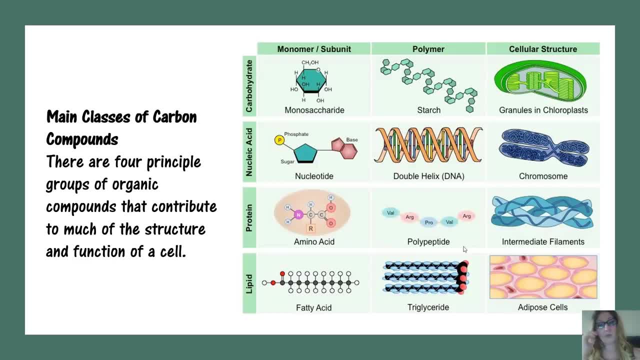 sugar. So we have our monosaccharide. Now if we put two monosaccharides together, we get a disaccharide, And eventually, if we get a bunch of them together now, we've got a polysaccharide. 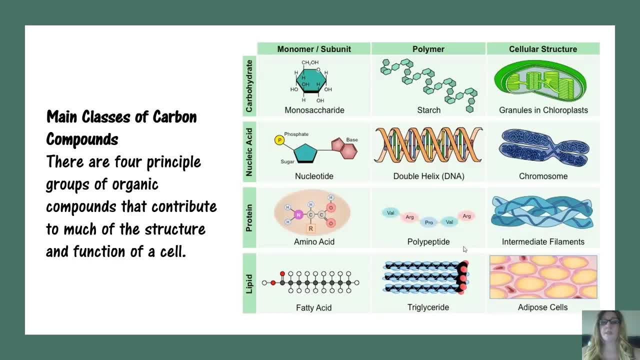 So our polysaccharides are going to be our polymers of saccharides, or polymers of carbohydrates or sugar. These are our complex carbohydrates, And starch would be an example of that. Nucleic acid make up our RNA. 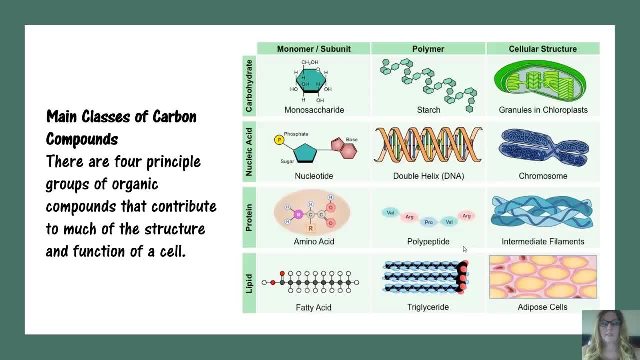 and our DNA, for example, And nucleic acids come together through the formation of phosphodiester bonds to form those larger polymers. So the DNA molecule and the RNA molecule would be considered a polymer made up of nucleic acids, which are 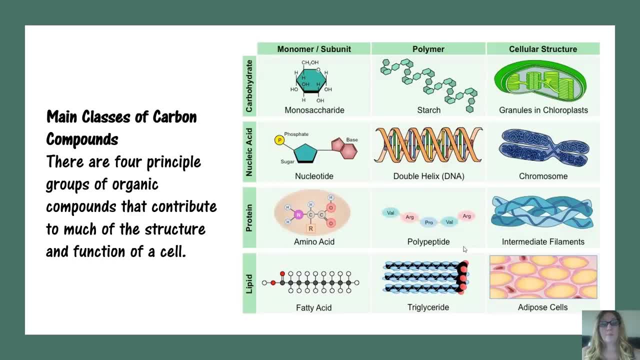 the individual monomers. Proteins are made up of individual monomers, which are the amino acids. So we have our amino acids and then those individual amino acids will be able to come together and form peptide bonds And we've got proteins that come together. 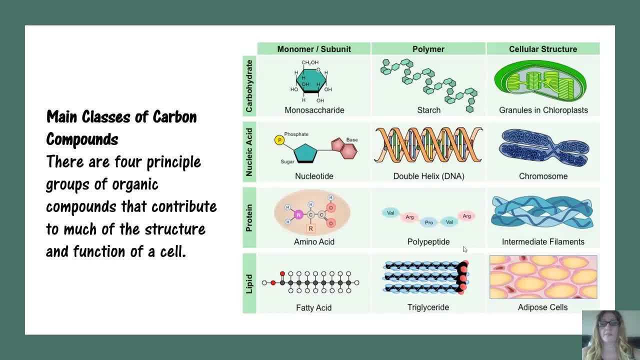 I've got two of them. I've got a dipeptide. If I have a small string of amino acids that becomes a polymere, A polypeptide, as that string gets very, very large, then it becomes referred to as a protein. 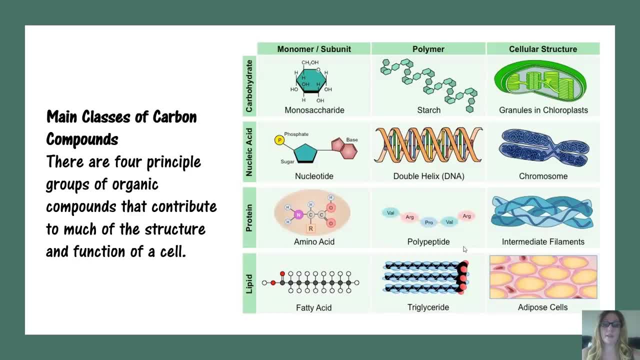 So a protein would be a polymer, A polypeptide would also be a polymer, And then the individual monomers would be the amino acids, Depending on the textbook you read, sometimes lipids are not considered monomers because the lipid molecule itself is not. 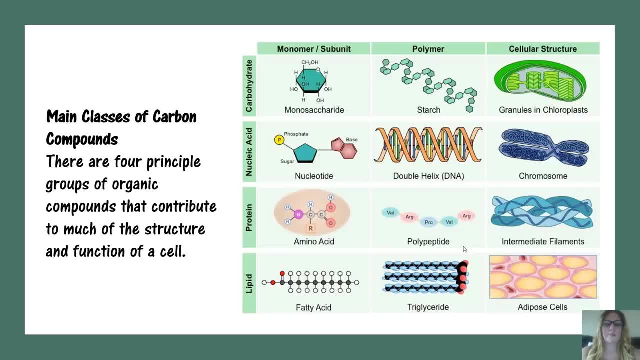 absolutely a repeating unit But nonetheless I went ahead and used this that I found because it was just convenient. But we do break down our lipids into their individual components And we separate them from the head group and so on and so forth. 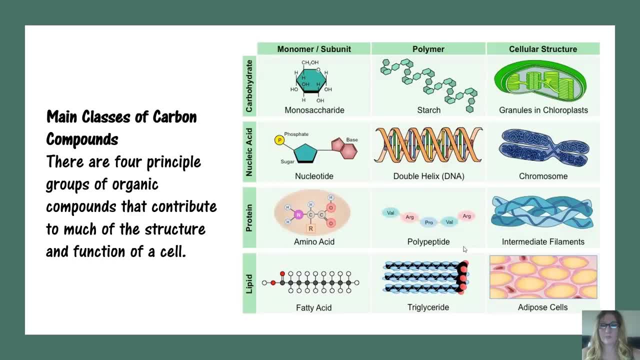 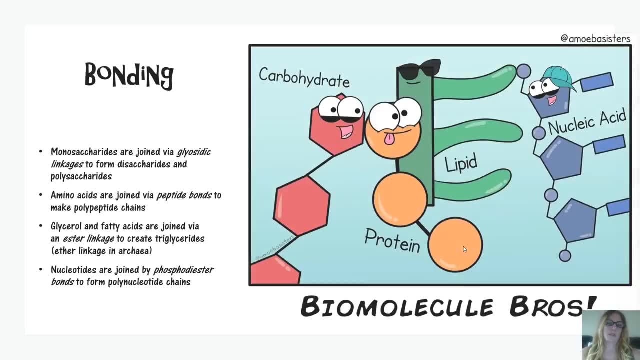 But they do make larger molecules that need to be synthesized or broken down, So it's important to know what types of bonds form these very important molecules that we depend on. Our monosaccharides are joined via a glycosidic linkage. 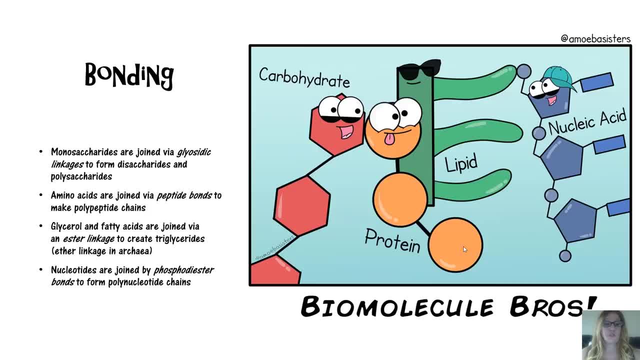 or a glycosidic bond. Amino acids join via peptide bonds. Glycerol and fatty acids are joined. as hopefully you know from our last module. They're joined using ester linkages or ester bonds, except for in the archaea, which uses 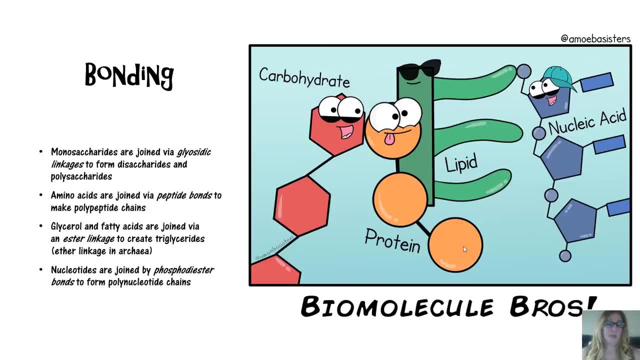 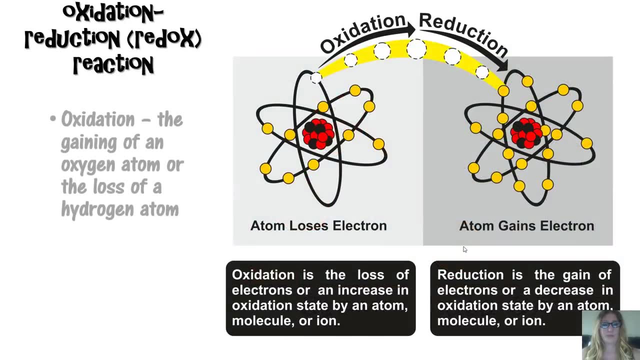 ether bonds instead, And this is true for phospholipids as well as the triglycerides, Nucleotides are joined together using the phosphodiester bonds. Okay, So I already gave you that one, so I'll skip that slide. 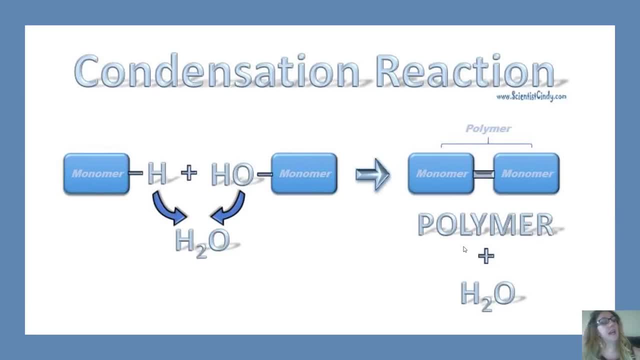 Alright. So if you look at how these larger molecules are formed from their individual monomers, when the monomers come together, what you're actually going to do is you're going to get a condensation reaction, and you can also call these a dehydration reaction. 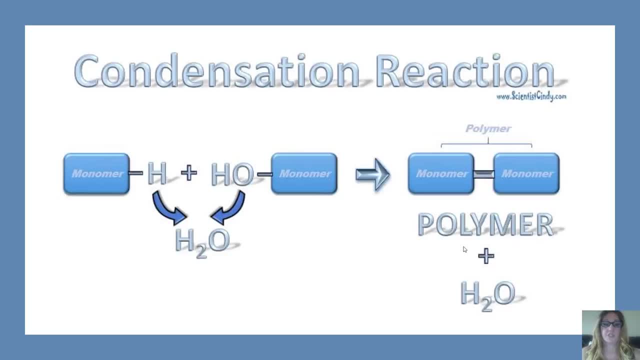 And the reason you're going to call it a condensation or dehydration reaction is because you're going to get water- oops. you're going to get water as a oops. no, go back, You're going to get water as a byproduct. 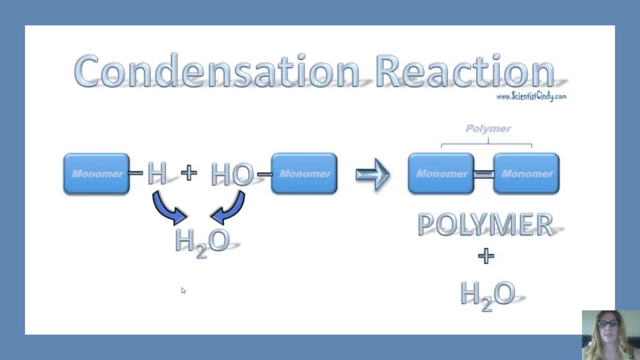 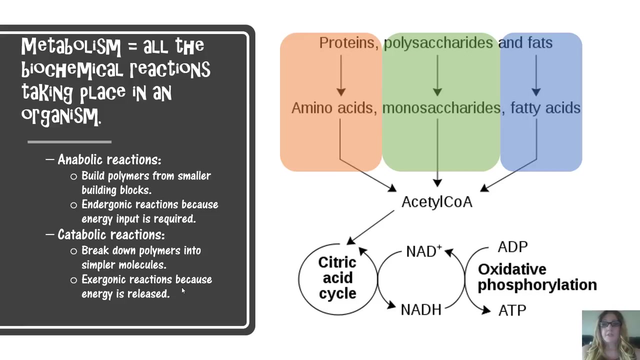 here. So you're creating the bond. This is also a type of a synthesis reaction. Anytime you have things joining together, you can call that a synthesis reaction as well. Alright, So, um, so here are just some of the, some of the. 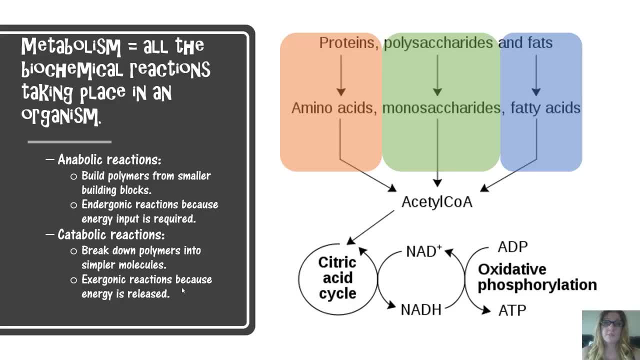 things to keep in mind. So we've got proteins that need to be broken down into amino acids. Polysaccharides need to be broken down into individual monosaccharides in order to be continued um to be catabolized further. 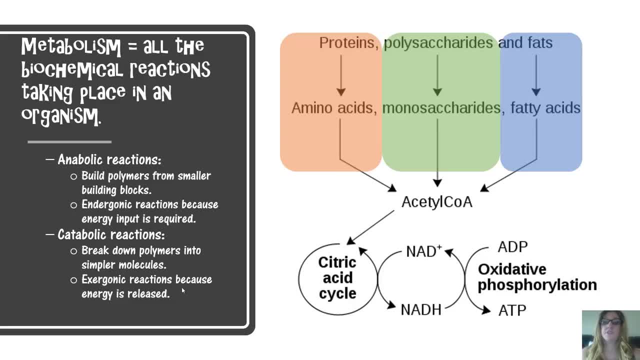 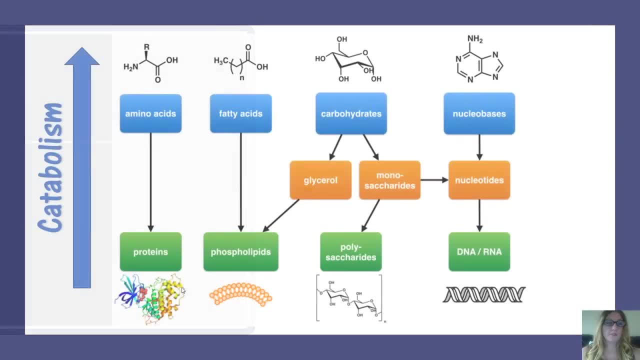 Fats need to be catabolized into um, into the individual fatty acids and um and glycerides. If we're building up molecules, we have to go, I'm sorry. if we're breaking down molecules, like I just said, we have to go um. 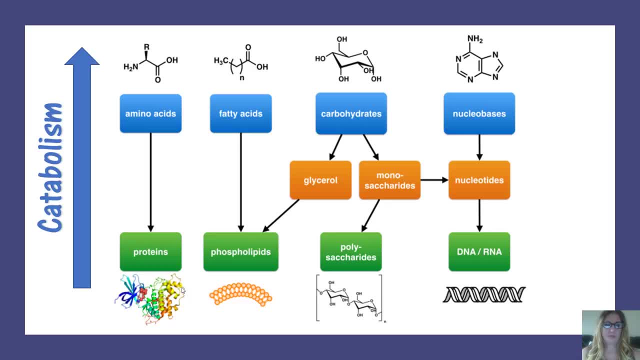 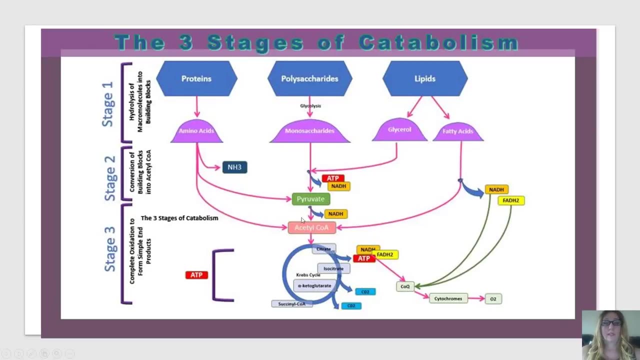 um, we have to go and break it down into from its polymer into its monomer. Okay, And so you're probably. so the um pathway that we were just discussing is actually right here, kind of in the middle, where it says: 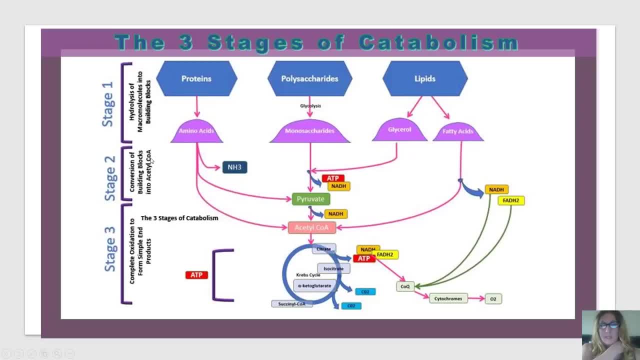 stage two, conversion of building blocks into acetyl CoA. So, um, that was actually where we took the monosaccharide. Now, glucose is a monosaccharide. Okay, so glucose was here at the beginning of glycolysis. 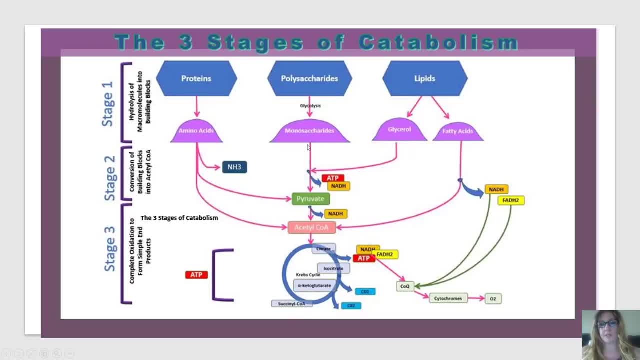 So glycolysis, um took glucose and converted that to pyruvate. After pyruvate, pyruvate was um converted into acetyl CoA And then acetyl CoA entered into the Krebs cycle. 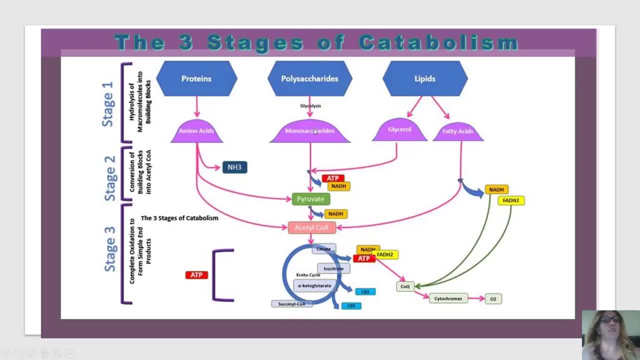 Now, that is the main pathway of your sugars, of your polysaccharides, Now, um. now, what about proteins and lipids? Well, if you look at this diagram, you'll see that, um that, their catabolic pathways. 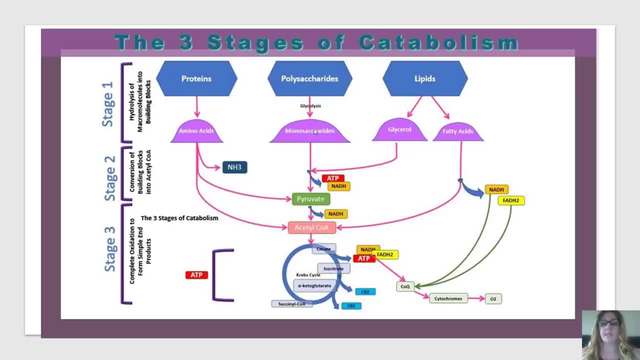 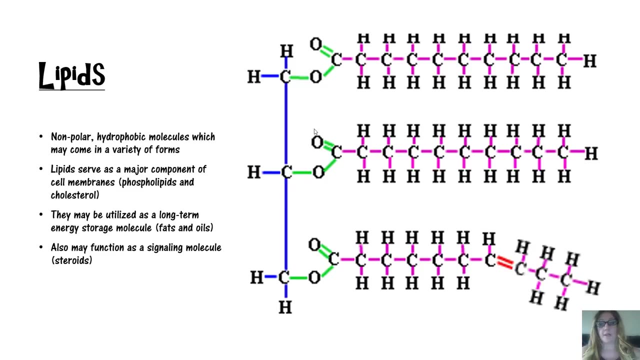 are all going to eventually feed back in to that main pathway of cellular respiration that we discussed at the beginning of the video, Which is very convenient and handy. Um, so this is the structure of the lipid. So the lipid is not, um, not a true polymer. 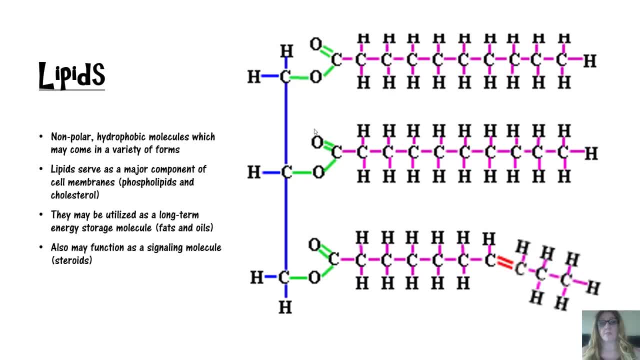 like the other ones are. Um, it's important to keep in mind that lipids are always going to be nonpolar, They're always going to be hydrophobic. Um, they are, um very important structures because they make up our phospholipids. 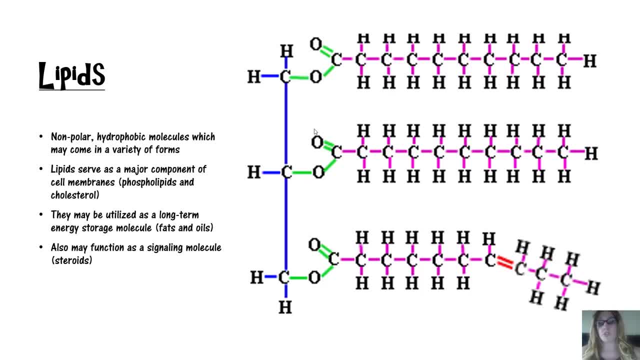 of course, They are great for long-term energy storage. Alright, so these are our fats, our oils. um, they're also used as signaling molecules, like steroids, for example. Most of our fats come in the form of triglycerides, and that's. 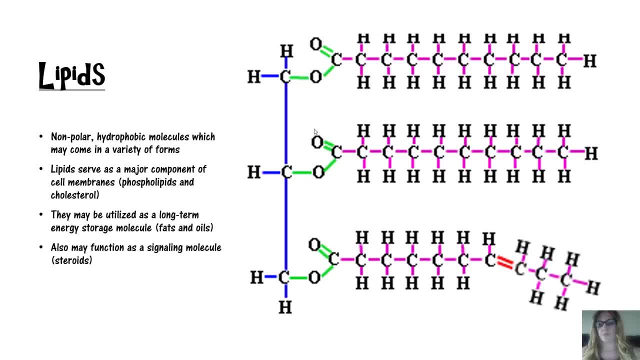 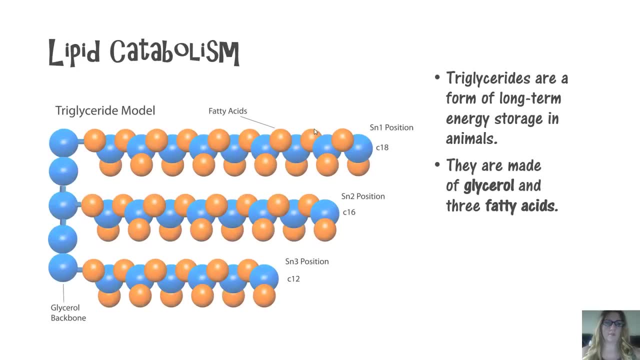 what this is here. So here you have your three fatty acids. okay, This is your triglycerides, And um and this. these uh fatty acids are attached to a glyceride here at the top, So when? 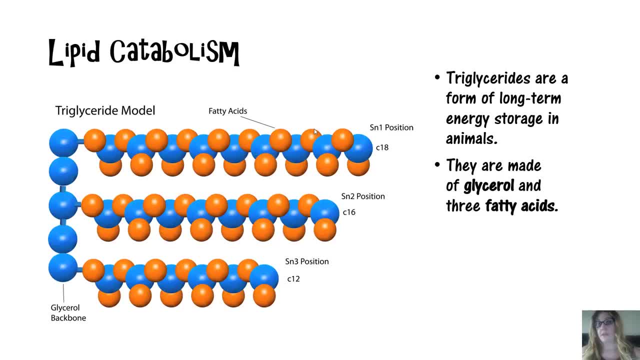 you're breaking down a lipid, you have to um, um, you have to break this uh molecule apart. So triglycerides are a form of long-term energy storage in animals and in um uh many prokaryotes. 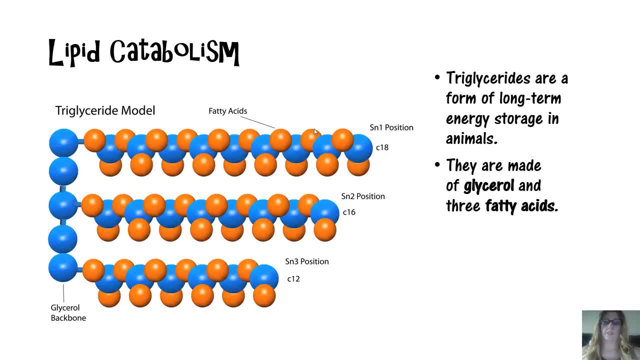 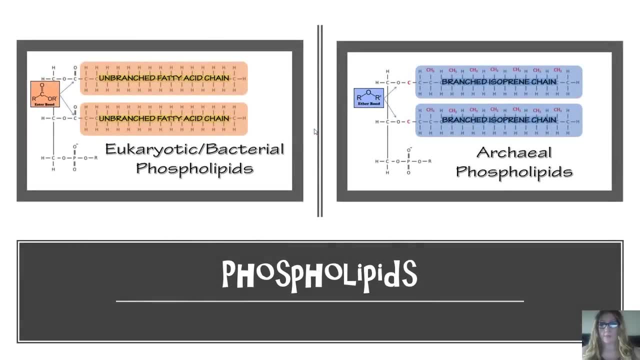 as well. So they're made of glycerol or glyceride and three fatty acids. Okay, Now the fatty acids. if you look at the fatty acid, maybe this one's a little bit easier. Okay, so if you look at this, 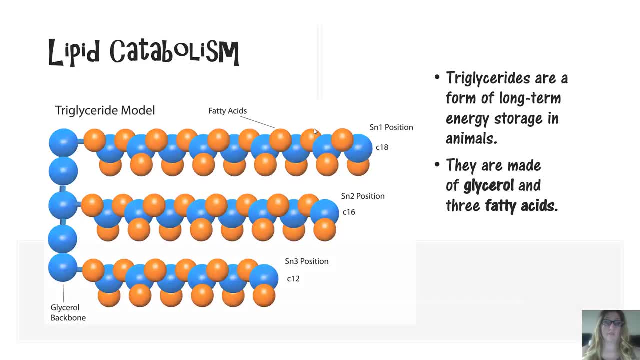 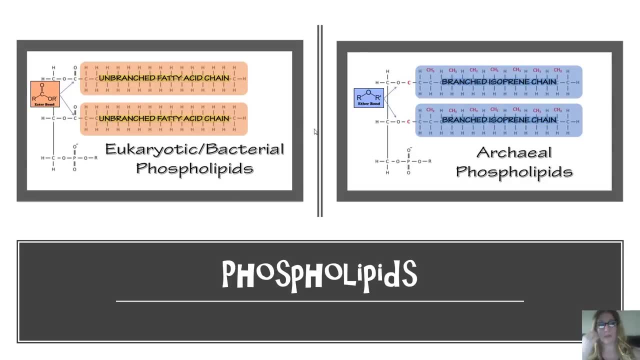 fatty acid. and then you look at the phospholipid. hopefully you see that they're remarkably similar, at least the eukaryotic bacterial phospholipid. The difference is that um, instead of having a third fatty acid chain here, 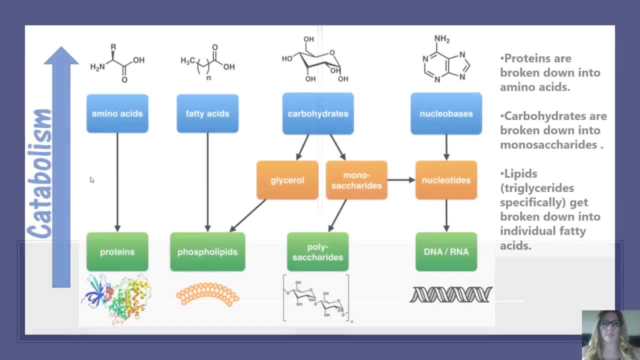 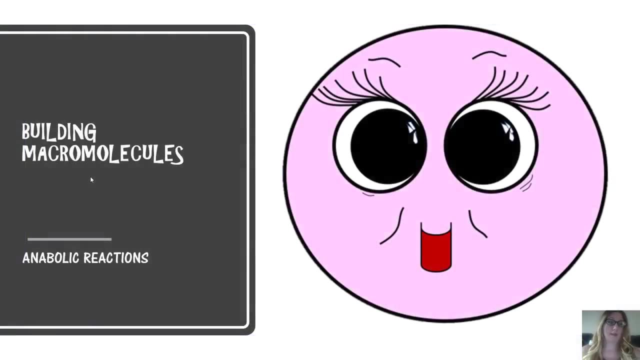 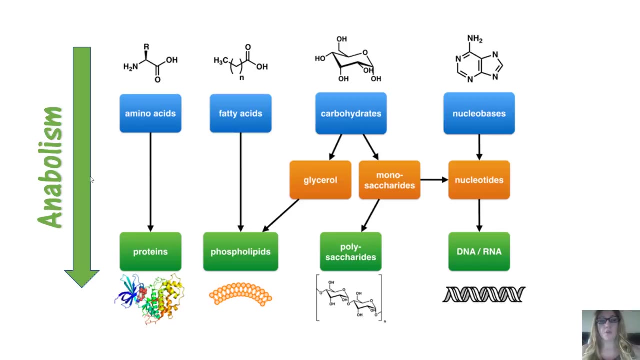 you're gonna have a phosphate, So very, very, um similar, And they're both considered fats. Alright, So let's just talk about some anabolic reactions for a moment. Let's talk about how do we build things when we, when we, 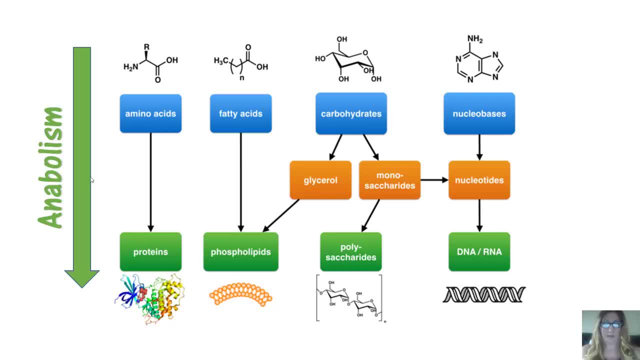 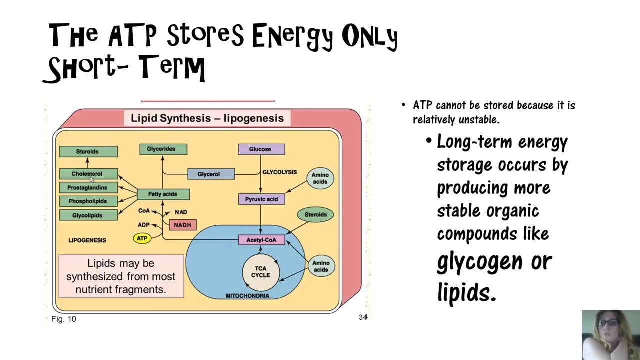 need them. Um so, cells are always in need of repair, Cells are in need of replacement. So sometimes we, sometimes we need to store energy long term When we make ATP. ATP does not hang out forever, Um that. 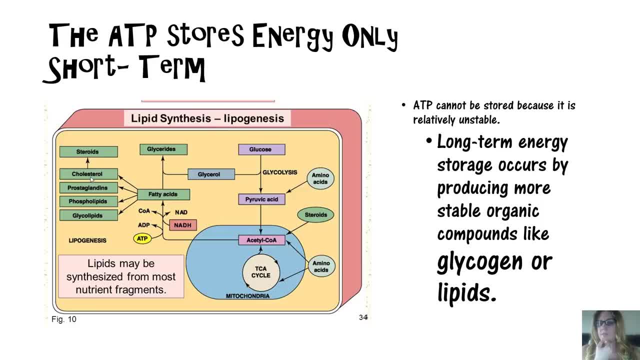 uh, high energy bond that we love so much to use for energy and ATP doesn't hang out forever, So it's short-lived. Um so if we want to have energy long term, we need to store it in a stable form. 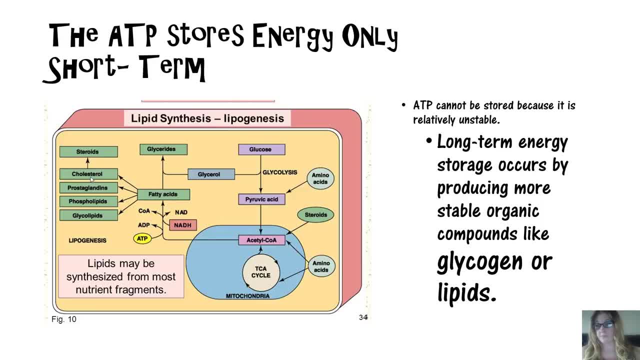 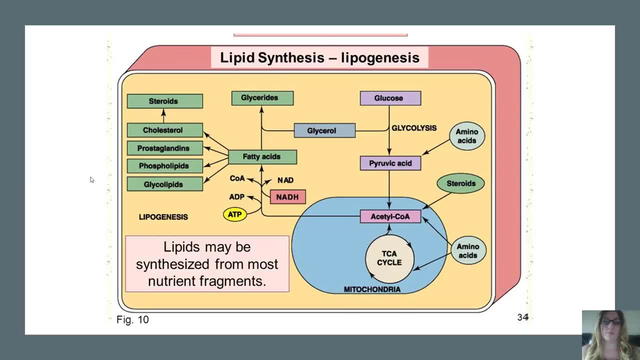 Those stable forms are glycogen or lipids. Okay, So how do we make lipids? We make lipids through lipid synthesis, otherwise known as lipogenesis. So here is a schematic of lipogenesis And I want you to realize. 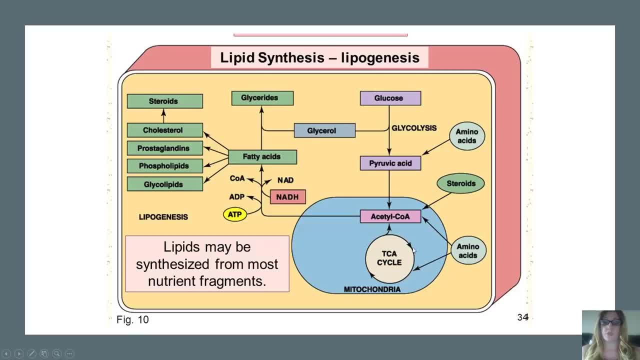 here. so the citric acid cycle is literally a cycle that goes in a circle. Now here from acetyl CoA, I can actually take acetyl CoA and form fatty acids using ATP and NADH, And I can form fatty 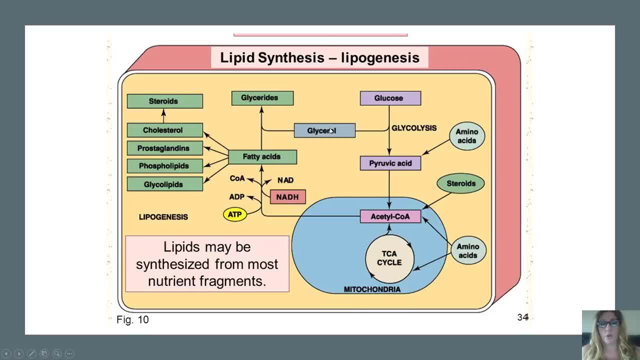 acids from there And then from there I can add other components, like I could add glycerol to make a glyceride. I can add um if I'm adding a phosphate. I can make a phospholipid If I'm. 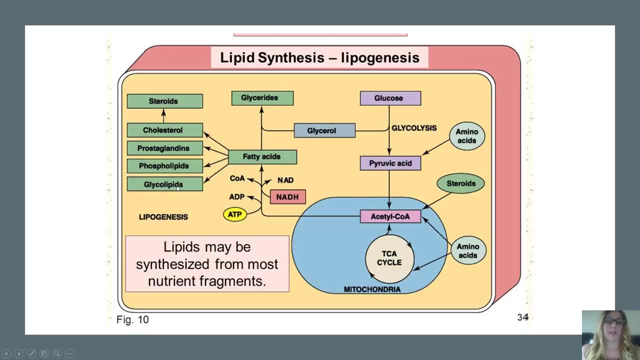 adding a sugar, I can make a glycolipid, Um, and you know, and so on and so forth. I can make my different types of molecules there. So, but you can see that it still is connected. This is still the main pathway that we 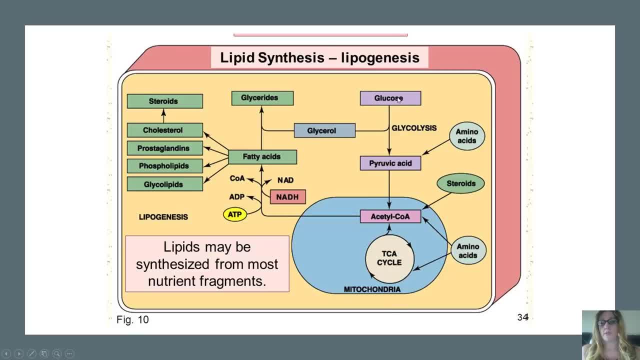 were discussing earlier at the beginning of the video. We've got our glycolysis here going from glucose to pyruvic. Pyruvic acid and pyruvate are the same thing, by the way, So glucose to pyruvate. 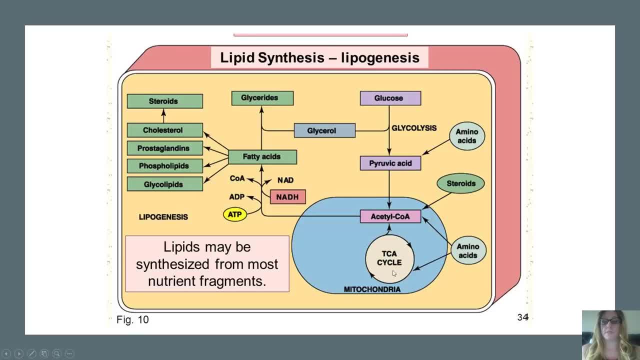 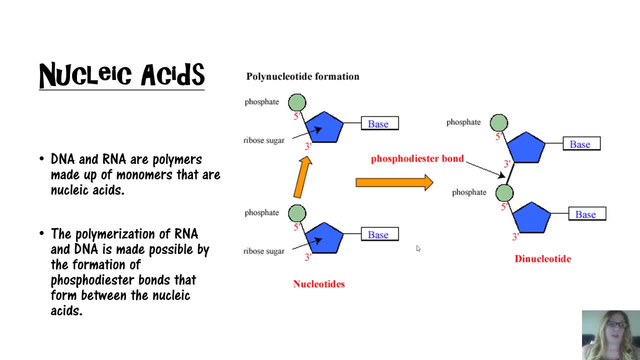 pyruvate goes to acetyl CoA and then that enters the citric acid cycle. So DNA and RNA are polymers made up of monomers of nucleic acids, and this is just showing you how those come together. Okay, so, 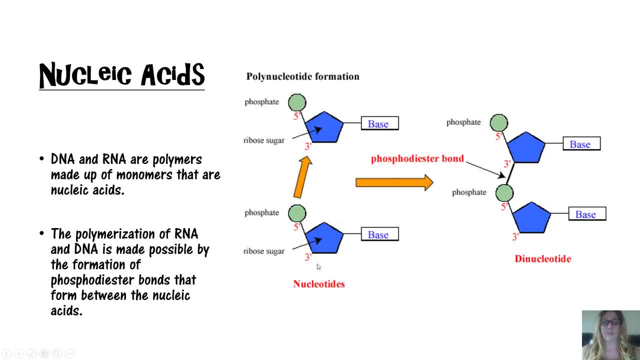 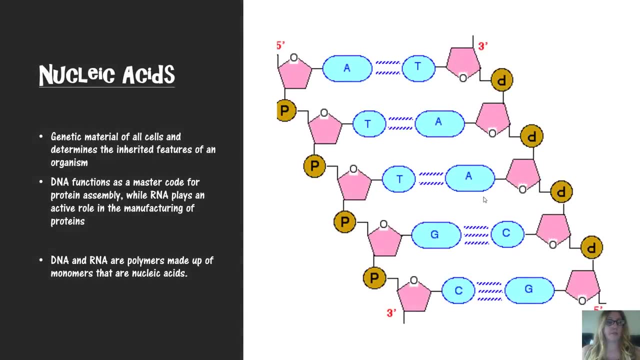 this would be an anabolic reaction, combining the nucleic acids together and forming the phosphodiester bond And phospho, because here is the phosphate, So phosphodiester bond And, in case you forgot, DNA is the genetic material of the cells. It. 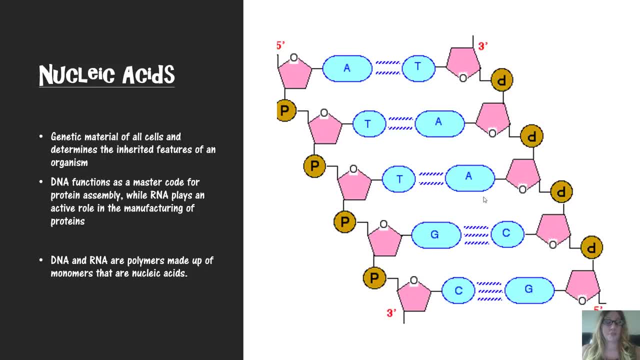 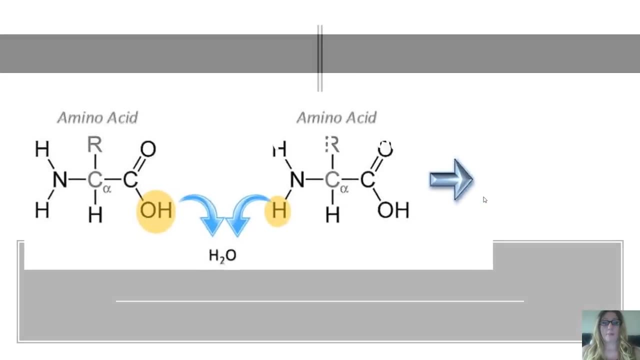 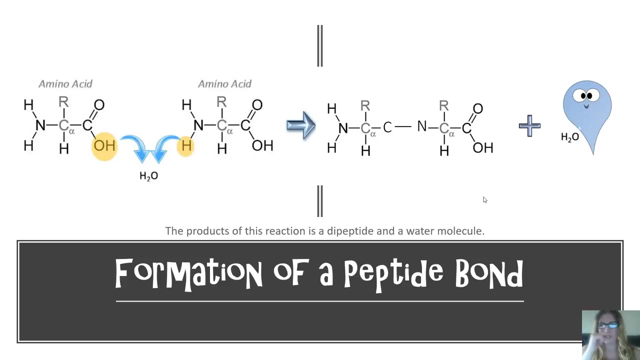 determines inherited features of the organism. It's the master code for protein assembly, while RNA plays the active role in manufacturing of the protein. When we form a peptide, this is another dehydration synthesis reaction, or condensation synthesis reaction. So we're taking 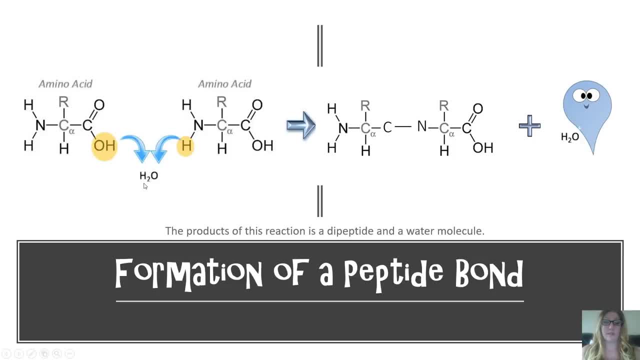 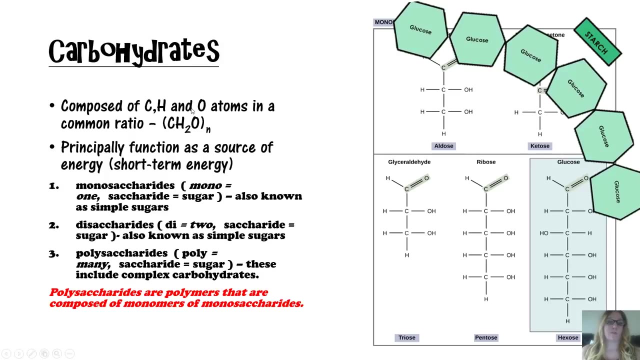 out water. Okay. so water is going to be a byproduct. So we take that out, we build the peptide bond and water is a byproduct: Carbohydrates. So carbohydrates are made up of just three elements: C, H and O. 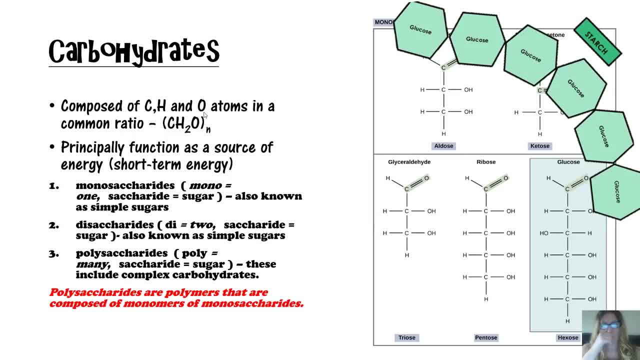 So carbon hydrogen and oxygen, And the ratio is always the same. It's always going to be C, H, O, with twice as much H as the C and O. Now, carbohydrates are good for short-term energy storage, Fats are better for. 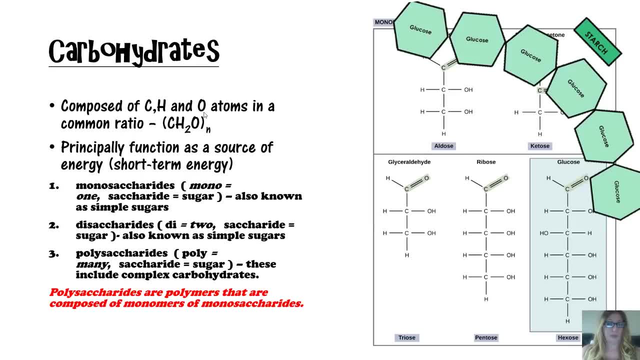 the really long-term storage If we have a monosaccharide. monosaccharides are also known as simple sugars. Simple sugars are also known as the disaccharides, because this has sucrose which is kind of like our table sugar. 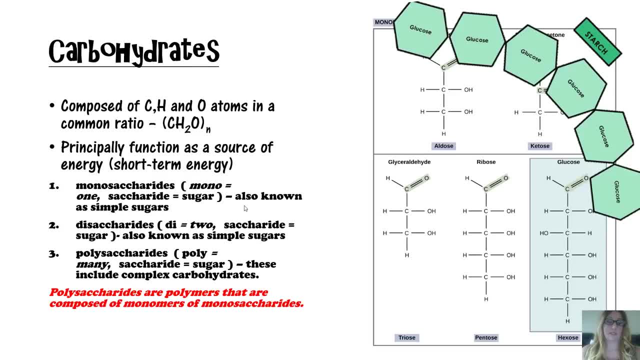 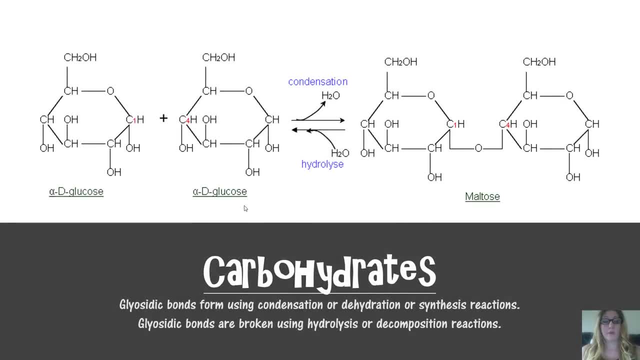 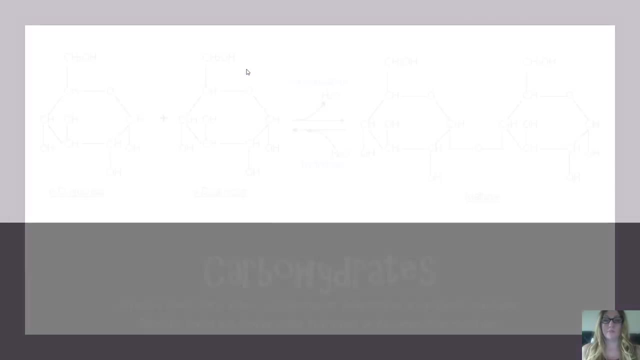 that we use, Polysaccharides are considered the complex carbohydrates. So how do carbohydrates polymerize? How do those monomers come together to form the polymer? So here we have our synthesis reaction again. Oops, We have our synthesis reaction, And. 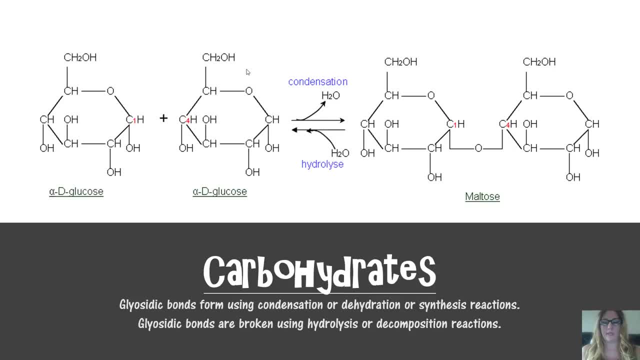 the synthesis reaction is going to be the same thing: a condensation reaction or a dehydration reaction, because we have the loss of water, And if we're going the other way, it's going to be a hydro, a hydrolysis or hydrolysis. 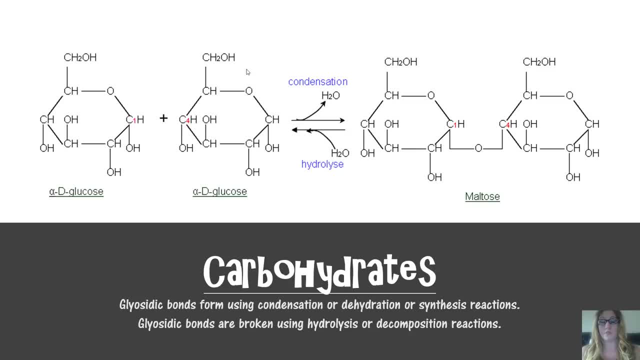 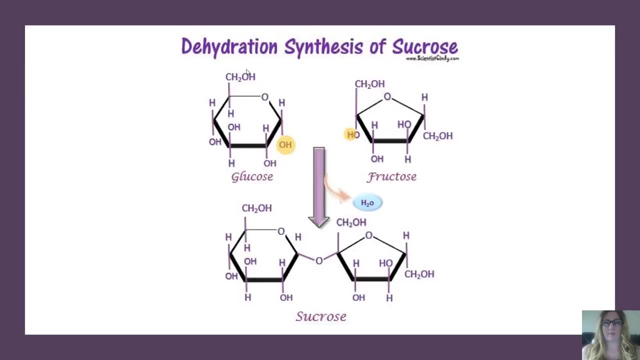 So lysis means to cut, Hydro means to cut with water, So hydrolysis to cut with water. We can also call that a decomposition reaction, because you're breaking the bond and breaking it down, And this is just another schematic that I made. 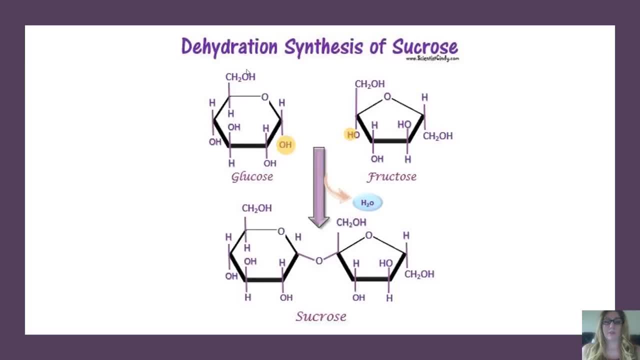 that I thought was pretty, so I put it up. And if you put glucose and fructose together, this is how you make our table sugar, which is sucrose And sucrose like if you go to the store and you buy a bag of sugar like. 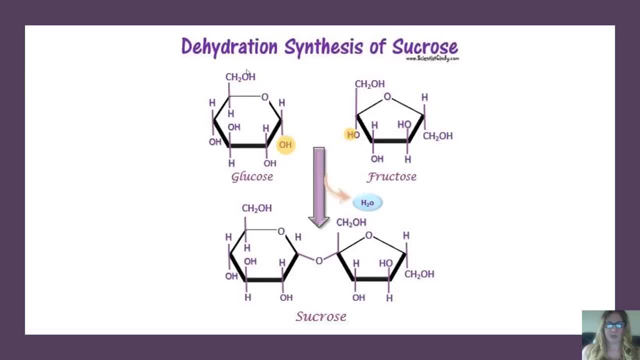 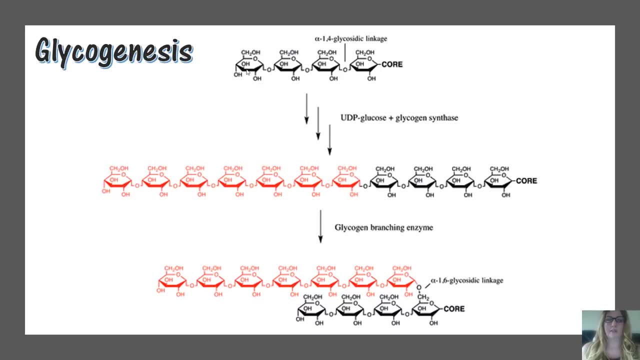 white bleached sugar, not the pure sugar, then this is what you would get. You would get sucrose. Glycogen is a very long chain of sugar And this is a good energy storage, So it is a polymer of sugar. 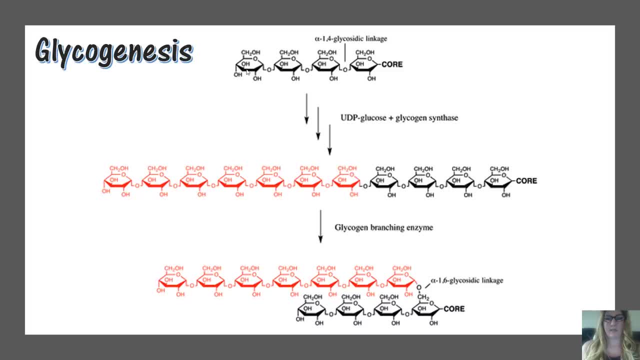 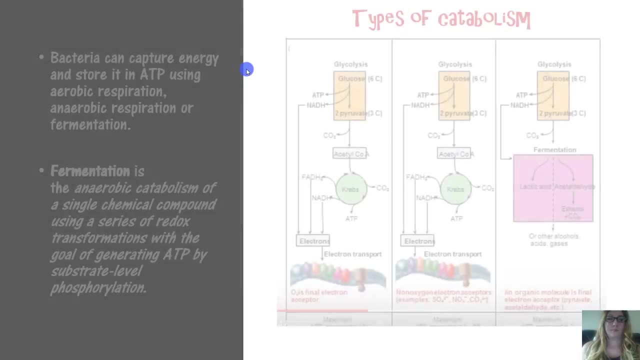 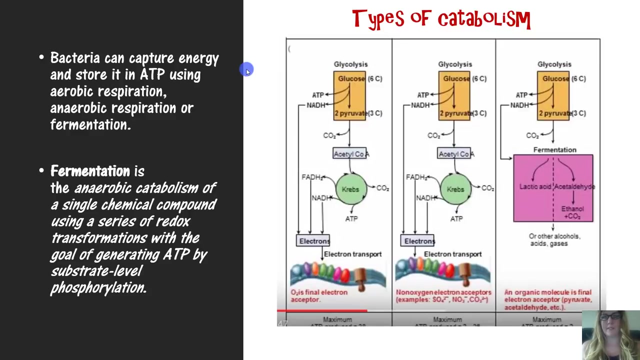 And it is just made up of a string of glucose And it can be branching here, Okay, Alright. So what about other types of catabolism? So let's continue to talk about some of these alternate forms. So we have talked at the beginning. 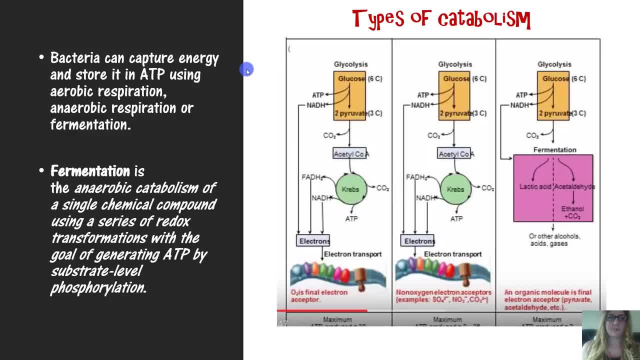 about cellular respiration. Let's talk about some of the variances that we see. So bacteria can capture energy and store it in ATP using aerobic respiration, like we went over at the beginning, or anaerobic respiration, which I'll teach to you in a 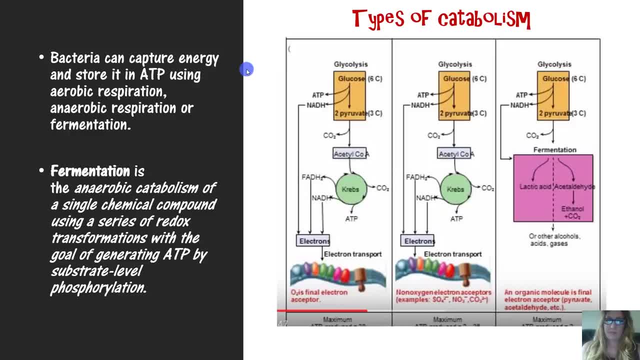 moment, or fermentation. Okay, So this first block, here is what we went over at the beginning. So here at the beginning we have our glycolysis, Here is our transition reaction, Here is our Krebs cycle or citric acid cycle, And then 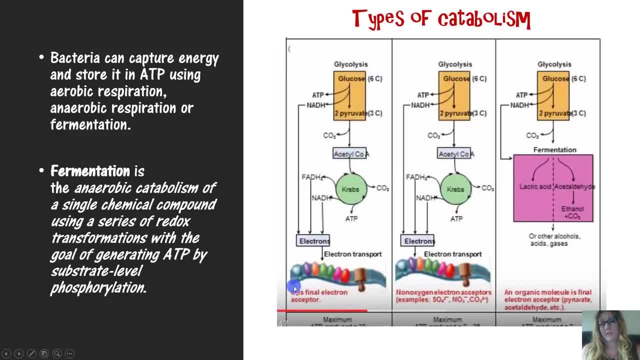 this is our electron transport chain, And then down here in blurry red you'll see that oxygen is the final electron acceptor. So, by definition, this first block is going to be our aerobic cellular respiration. The second block, the one in the middle here, 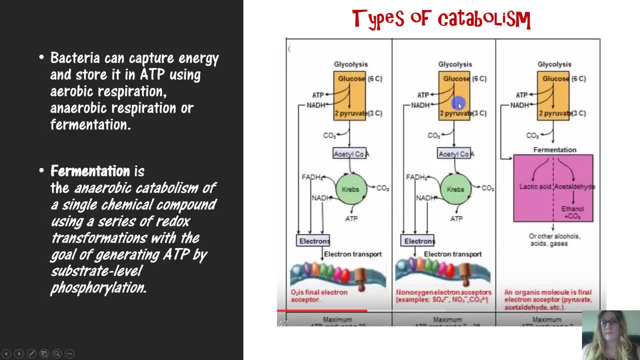 now the one in the middle. here you'll see, we've got our glycolysis, we have our transition reaction, we have our citric acid cycle, or Krebs cycle, and we have our electron transport chain. However, at the 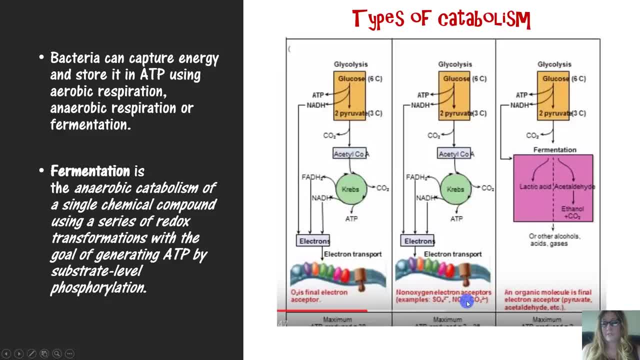 end here. instead of having oxygen, I have non-oxygen electron acceptors. So I've got carbonate, I've got nitrite, I've got sulfate, but I do not have oxygen. This is anaerobic respiration. Okay, this is. 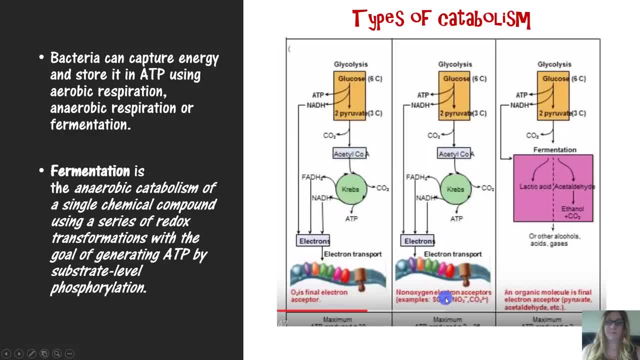 anaerobic respiration. Now, this third block is fermentation. Now, fermentation is also a type of anaerobic respiration And I'll explain a little bit more in just a moment. So this is also anaerobic respiration, because 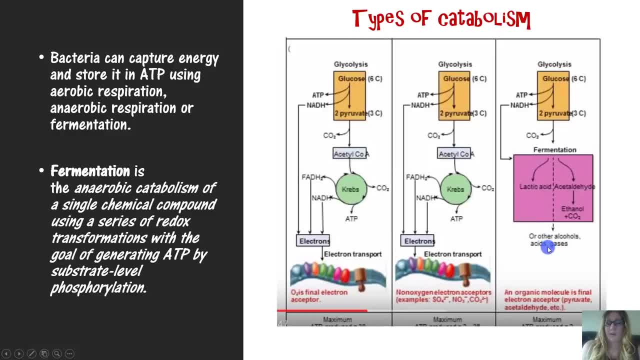 as you can see, this also does not have oxygen as a final electron acceptor. Right, Because that's the definition of aerobic respiration. This first block is the only one that has oxygen as its final electron acceptor. If it does not meet that criteria, 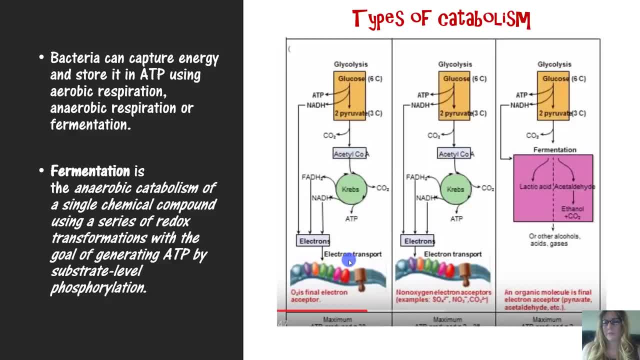 it must be anaerobic cellular respiration. Okay, So these two last blocks are considered anaerobic cellular respiration technically, But microbiologists kind of prefer a little bit, because we would never call fermentation, I mean we would. 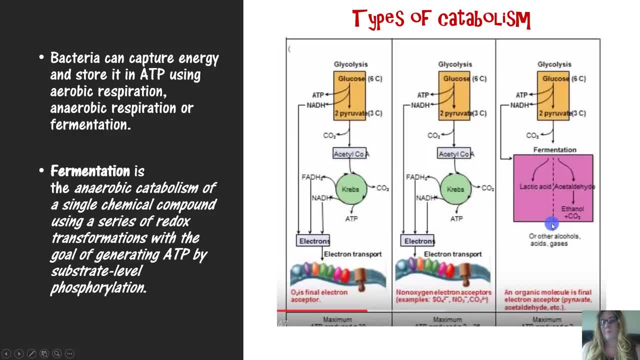 never call this second block fermentation, But it is often that people will call fermentation anaerobic cellular respiration, but you would never call cellular respiration fermentation. So it's just kind of weird. But I think the issue is really the reason why. 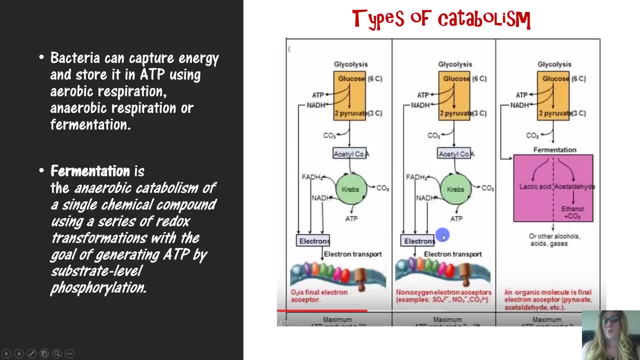 there's that issue is because this true, pure anaerobic cellular respiration has not been around for very long. We did not know this existed 15 years ago, So it's pretty new. I think that our terminology needs to change. 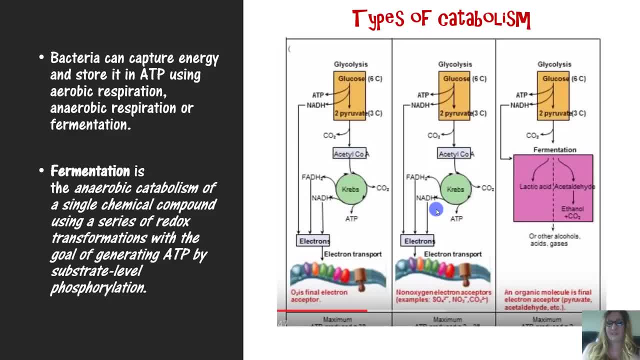 because it does make it very confusing for students, and I do understand that. So you just have to kind of go back to what the definitions are and just make sure you're remembering the definitions and stick to them. So the definition of anaerobic: 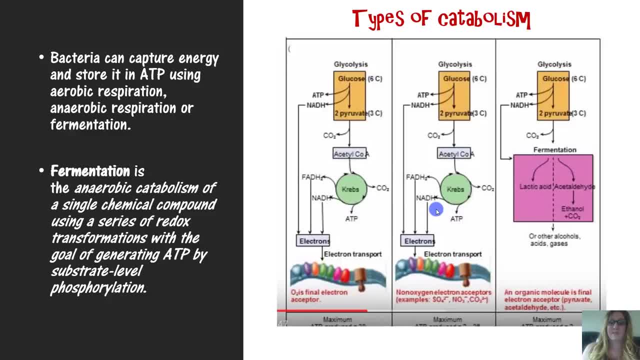 cellular respiration is that oxygen has to be the final electron acceptor Period. Okay, Now you'll notice. carbon dioxide is in all three of these. Do you see this? Okay, Hopefully you remembered at the beginning of the lecture cellular respiration. 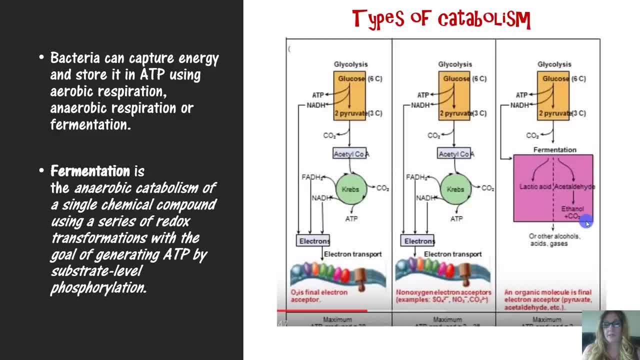 I didn't put aerobic or anaerobic at the beginning. Cellular respiration in general is defined by taking an organic molecule- usually carbohydrate, but it doesn't have to be carbohydrate- and oxidizing it completely into usually carbon dioxide and water And, believe it or not, all three. 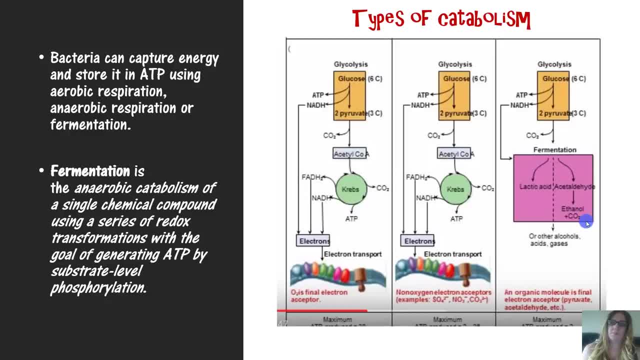 of these blocks will meet that criteria. Okay, So it's a very broad, open definition that does meet the criteria for all of these new metabolic pathways that are continuously being discovered. Alright, Now the definition for anaerobic cellular respiration is that: 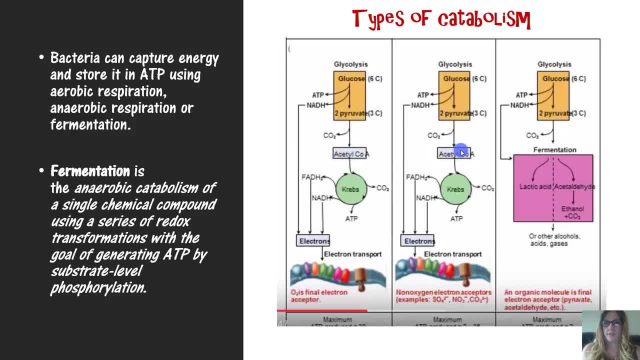 the final electron acceptor is not oxygen. So there you have it. But if it is fermentation, then the final electron acceptor is an organic molecule such as pyruvate or acetaldehyde. So it's weird. but 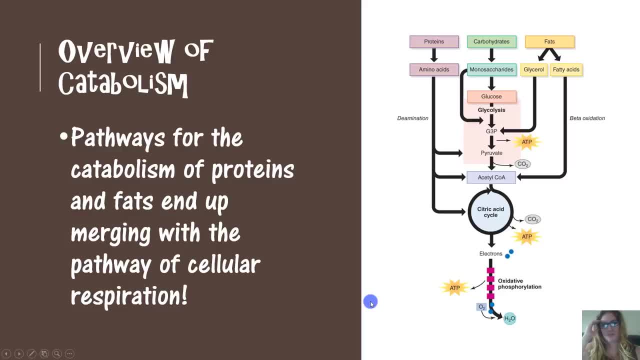 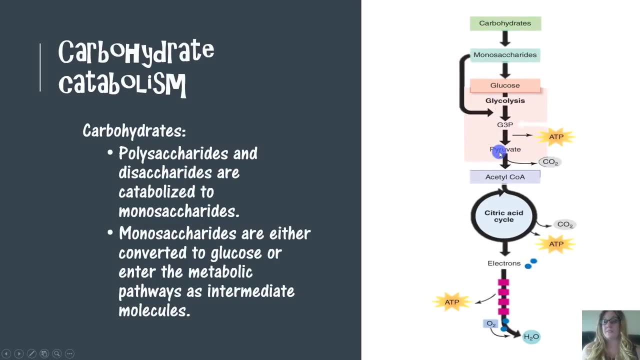 it is what it is, Alright, So overview of catabolism. So let's talk a little bit more about these alternate energy sources that we have. So this is the one that we started with, Just to get you kind of. 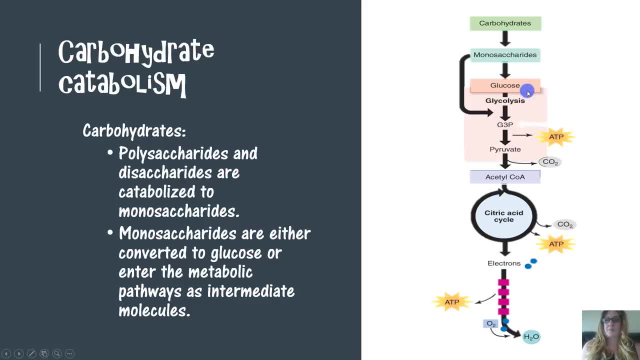 familiarized with this new figure that I'm going to be using. So it's a little bit bigger than just the normal cellular respiration, because we're actually going to start with the larger polysaccharide. So we've got our polysaccharide. 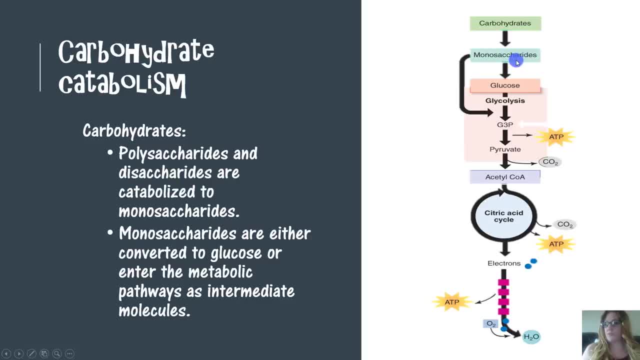 that is ingested, It gets broken down into its monosaccharide form. It gets converted. if it's not already glucose, It will get converted into glucose and then enter glycolysis. transition reaction, citric acid cycle, electron transport chain. 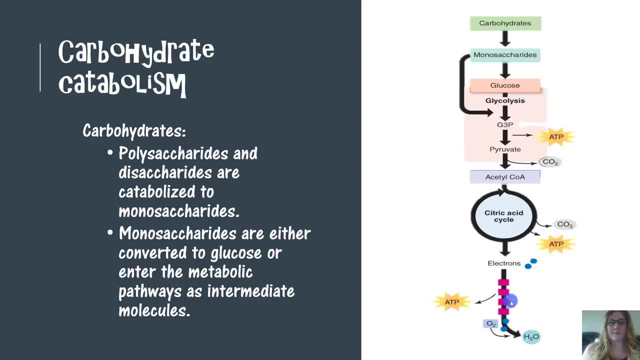 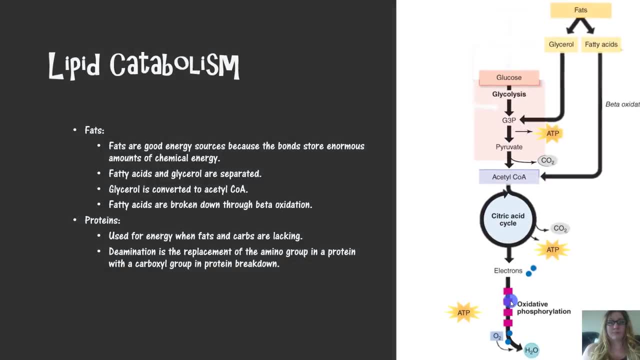 So that is the entire catabolism pathway for carbohydrates. What about fats? So let's talk about fats for a moment. So fats are good energy sources. Okay, They have a lot of hydrocarbon bonds. They store enormous amounts of energy. 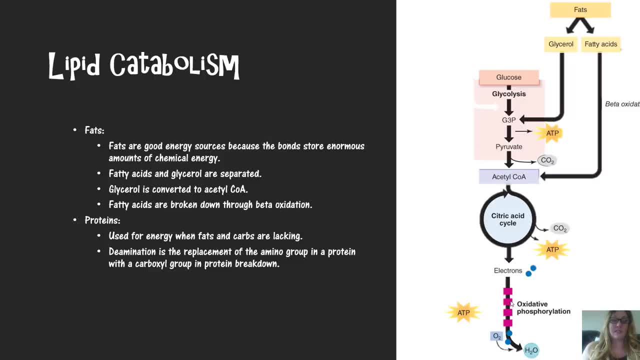 The fatty acid chains are actually separated from the glycerol. Okay, So I've got my fats. So fatty acid chains are going to be separated from the glycerol. So we see that at the beginning of our catabolic pathway here. 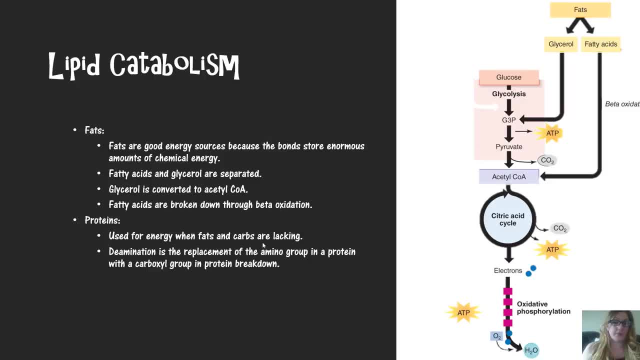 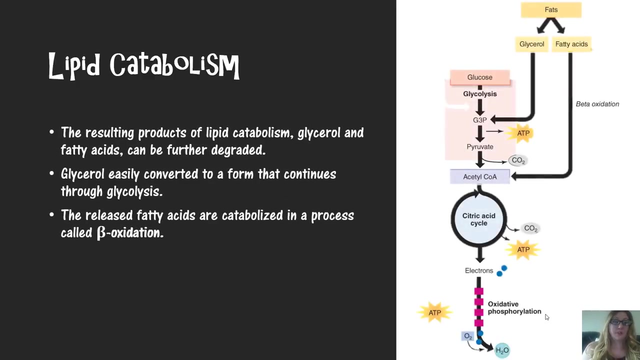 Now the fatty acids are broken down through beta-oxidation And the glycerol is converted to acetyl-CoA, And then after that, it just continues to go through the pathway of cellular respiration, The resulting products of lipid catabolism. 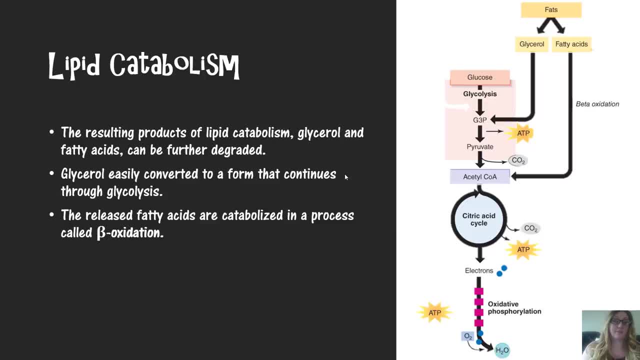 are glycerol and the fatty acids can further be degraded. Glycerol can easily be converted to a form that continues through glycolysis, And the released fatty acids are catabolized in a process called beta-oxidation. So we've got 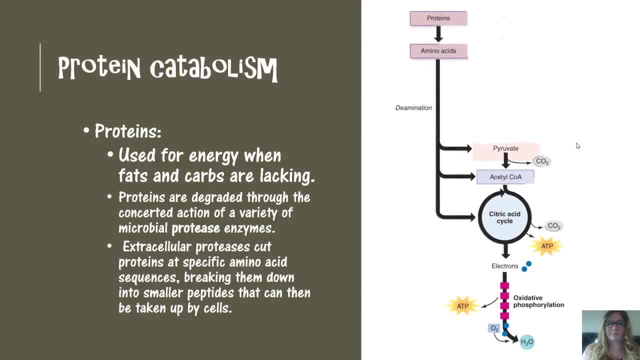 beta-oxidation. How about proteins? So proteins are used for energy as a last resort. So it will use carbs first, fats as a second choice and proteins are a last ditch effort. So proteins will be degraded through a bunch of different protease. 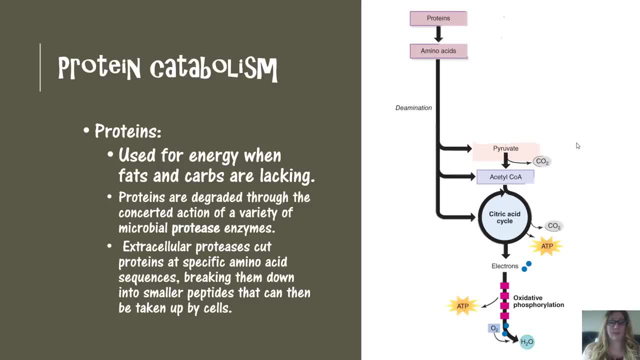 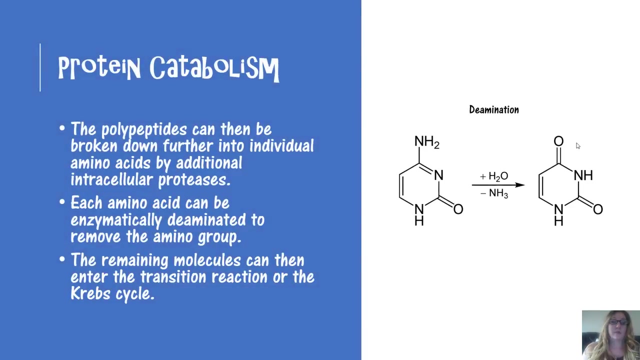 enzymes that are hanging out. Extracellular proteases are going to cut proteins at specific amino acid sequences and break them down into smaller peptides. Those smaller peptides can then be broken down further, So the polypeptides can then be broken down further into. 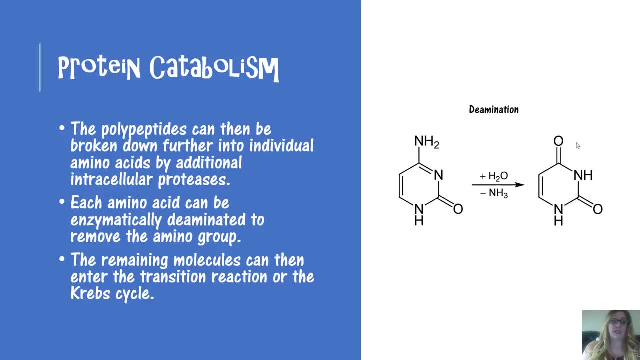 individual amino acids by additional intracellular proteases. Each amino acid can be enzymatically deaminated to remain the amino group. So here is the deamination. The remaining molecule can then enter the transition cycle or the transition reaction, or I can. 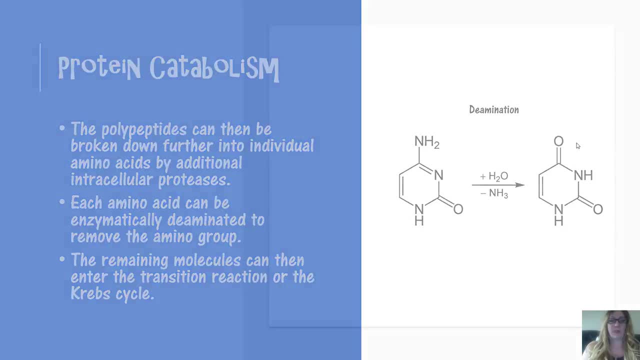 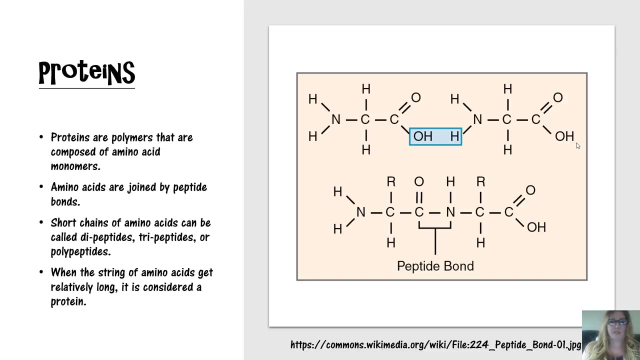 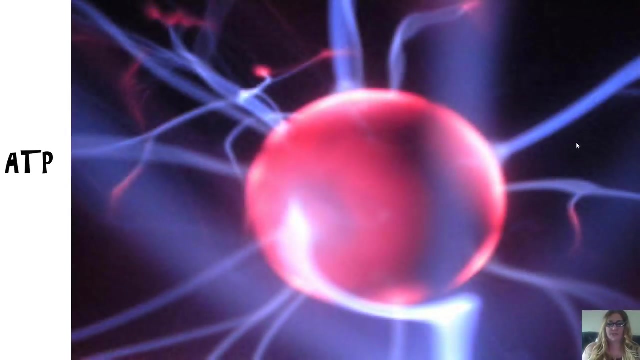 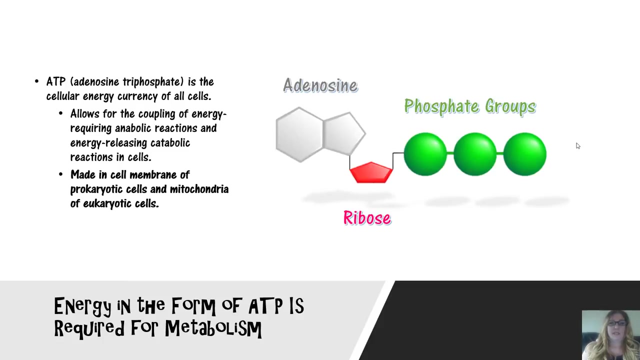 go directly into the Krebs cycle: Proteins. So proteins are polymers of the amino acids and they are joined by those peptide bonds. and here is where that peptide bond is formed. Alright, ATP. Okay, So ATP is adenosine. 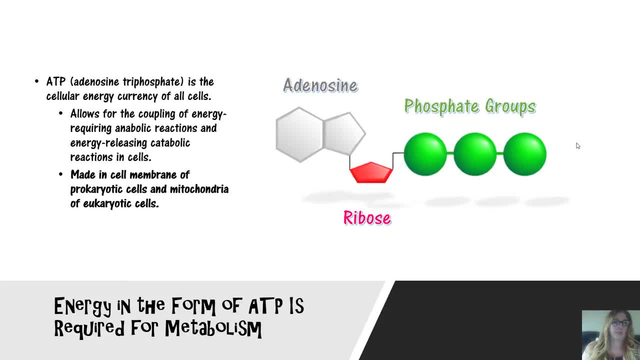 triphosphate, And it is the cellular energy for all cells, allowing for the coupling of energy requiring anabolic reactions and energy releasing catabolic reactions in cells. It is made in the cell membrane of prokaryotic cells and mitochondria of eukaryotic. 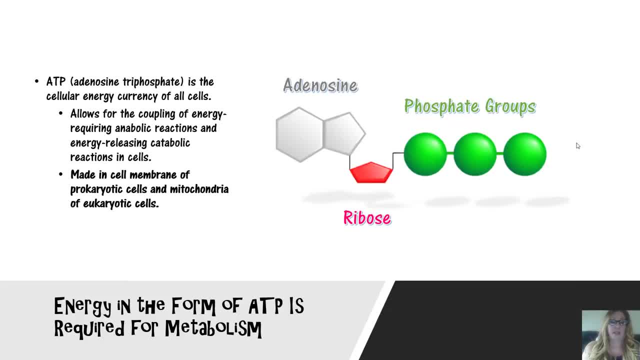 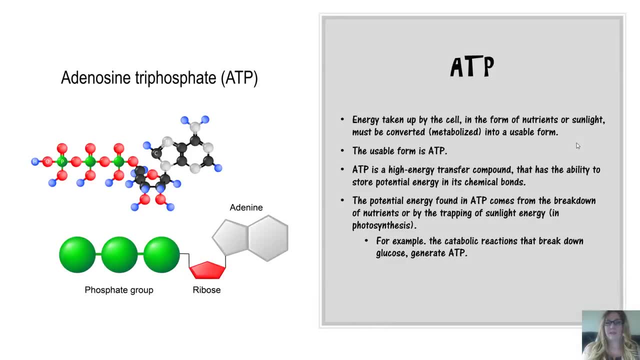 cells. So energy is in the form of ATP and it is required for metabolism. So energy taken up by the cell in the form of nutrients or sunlight must be converted or metabolized into a usable form. The usable form is ATP, ATP. 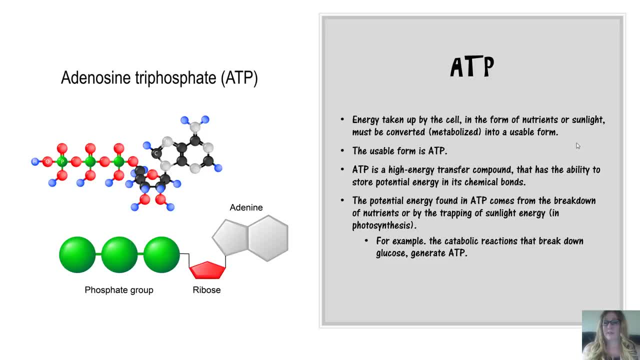 is a high energy transfer compound that has the ability to store potential energy in its chemical bonds. The potential energy found in ATP comes from the breakdown of nutrients or by trapping of sunlight. in photosynthesis, For example, the catabolic reactions that break down glucose. 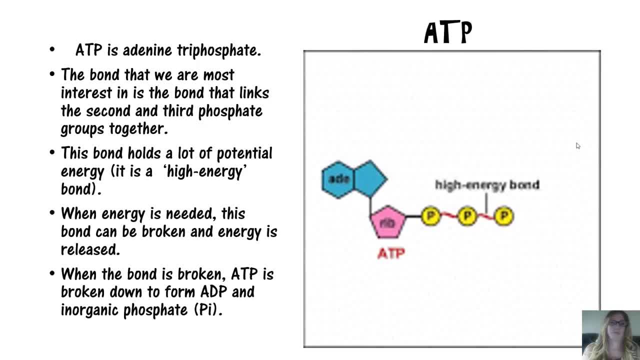 generate ATP. ATP is adenine triphosphate. The bond that we are most interested in is the bond that links the second and third phosphate groups together. This bond holds a lot of potential energy. It is a high energy bond When the energy is needed. this 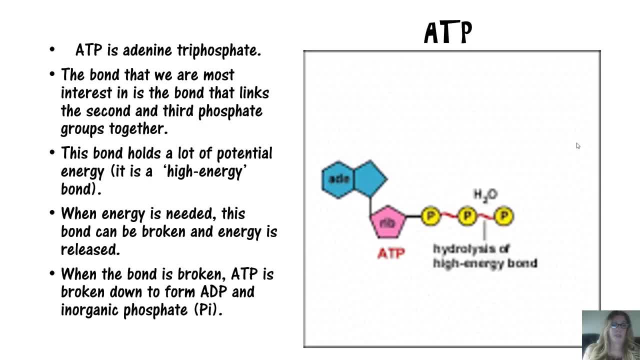 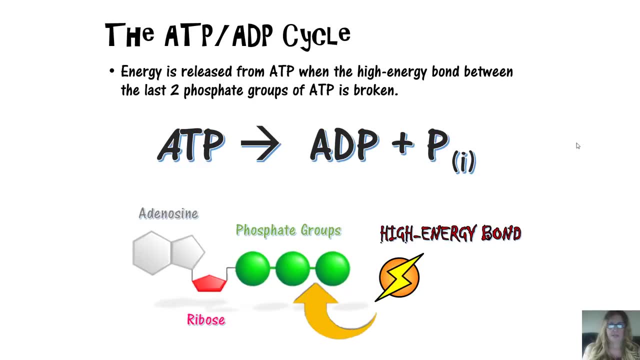 bond can be broken and energy is released. When the bond is broken, ATP is broken down to the form ADP and inorganic phosphate, The ATP ADP cycle. So we have our ADP, ADP- sorry, ATP ADP cycle. 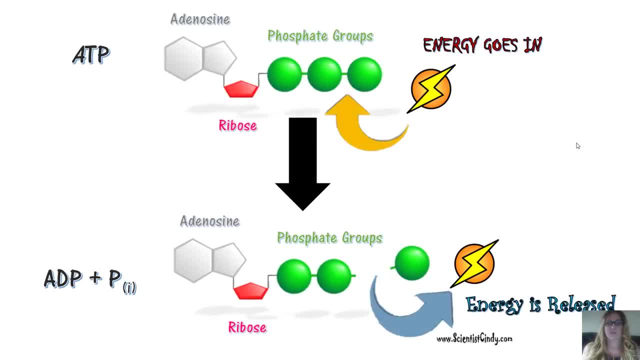 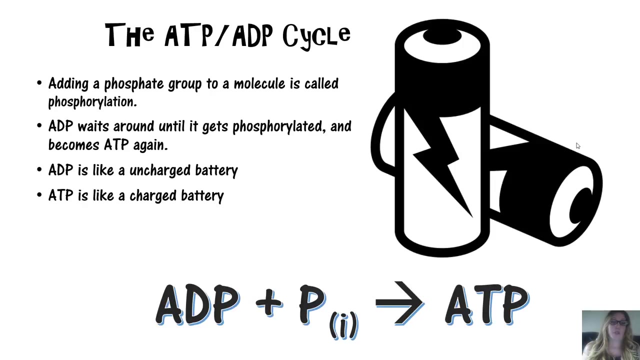 So this molecule is going to switch back and forth between ADP and ADP, So when that bond breaks, energy gets released and it will be like an uncharged battery. So adding a phosphate group to a molecule is always going to be called phosphorylation. 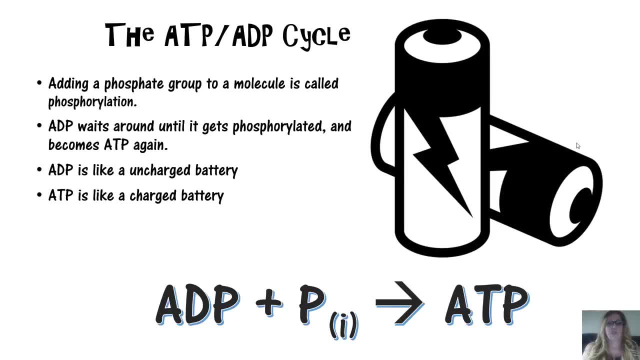 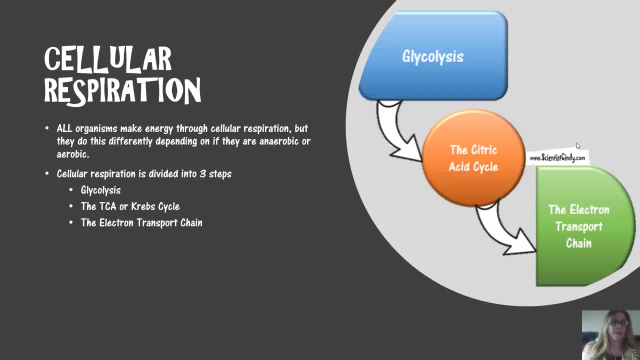 So ADP waits around until it gets phosphorylated and becomes ATP again. ADP is like an uncharged battery. ATP is like a charged battery. So all organisms make energy through cellular respiration, but they do this differently depending on if they are anaerobic. 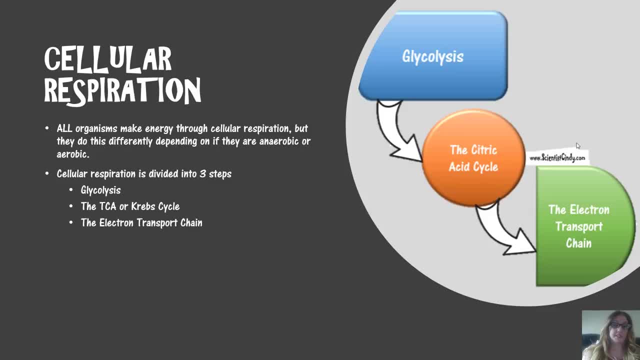 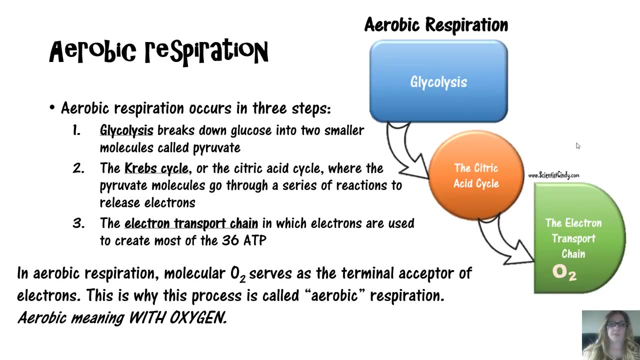 or aerobic. So cellular respiration is divided into these three steps: Glycolysis, the TC, or Krebs cycle, and the electron transport chain, or oxidative phosphorylation. So just to refresh your memory, aerobic respiration occurs in these three steps. 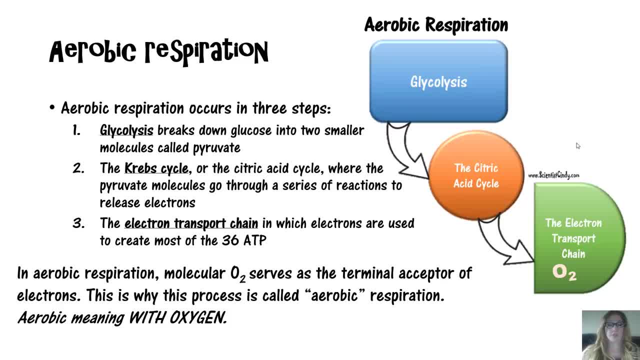 Glycolysis breaks down glucose into two smaller molecules called pyruvate. The Krebs cycle, or citric acid cycle, is where pyruvate molecules go after it's been converted into acetyl-CoA, just to be specific. to go through a series. 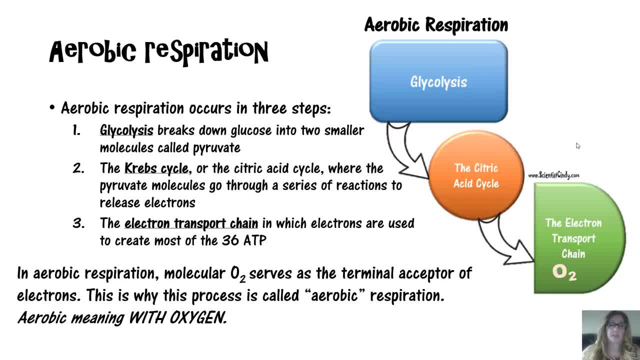 of reactions to release more electrons, and then the electron transport chain are used to create most of the 36 to 38 ATP In aerobic respiration. molecular oxygen serves as the terminal acceptor of electrons. This is why the process is called aerobic respiration, meaning. 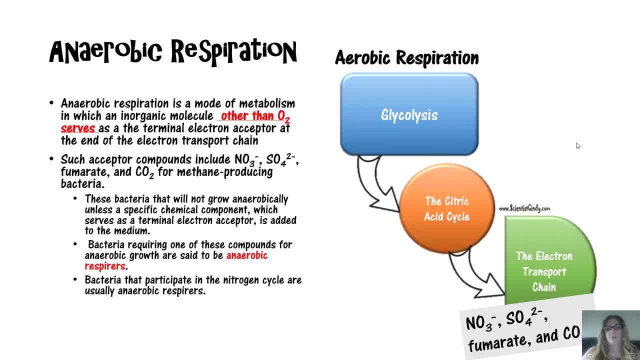 with oxygen. So what happens if it's anaerobic? So anaerobic respiration is a mode of metabolism in which an inorganic molecule other than oxygen as the terminal electron acceptor at the end of the electron transport chain. So 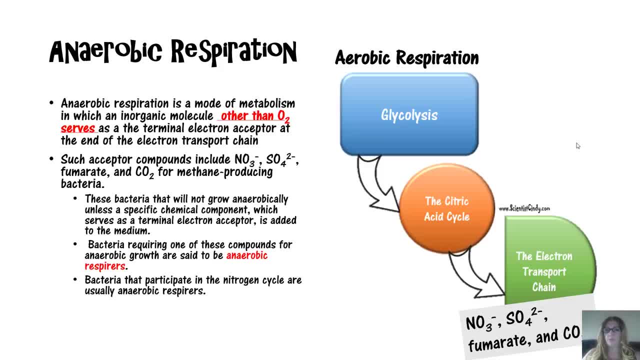 notice that I said inorganic, because if it's an organic molecule, it's actually going to be fermentation. So let me just repeat that If it's an organic molecule, we will call that fermentation and we will not go through all three of these steps shown. 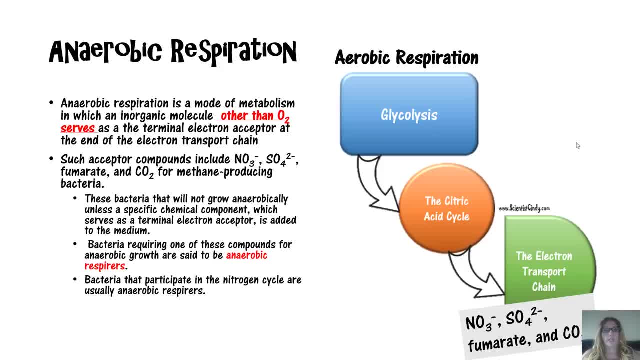 here. So anaerobic respiration is a mode of metabolism in which an inorganic molecule other than oxygen serves as the terminal or final electron acceptor at the end of the electron transport chain. Such acceptor compounds include nitrite, sulfate. 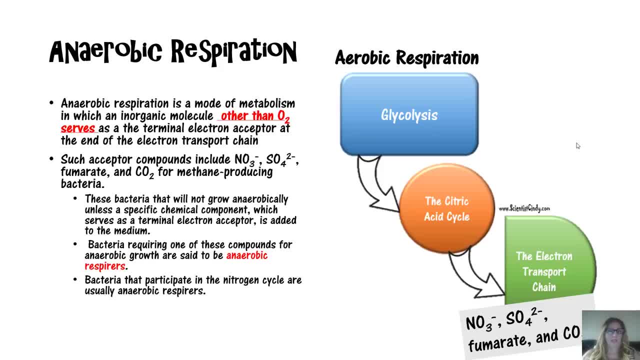 and fumarate and carbon dioxide for the methane producing bacteria. These bacteria will not grow anaerobically unless a specific chemical component, which serves as the terminal electron acceptor, is added to the medium Bacteria requiring one of these compounds for anaerobic growth. 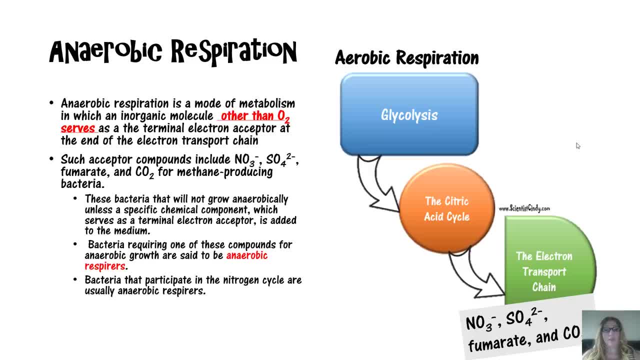 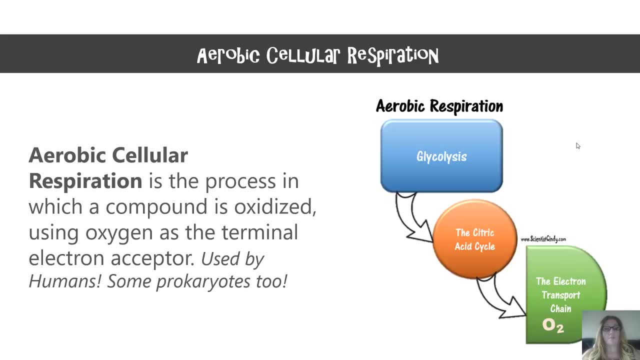 are said to be anaerobic respirers. Bacteria that participate in the nitrogen cycle are usually anaerobic respirers. Aerobic cellular respiration is the process in which a compound is oxidized using oxygen as the terminal electron acceptor. Now this is used by 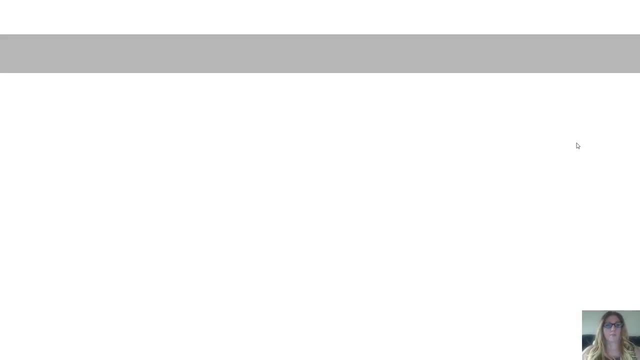 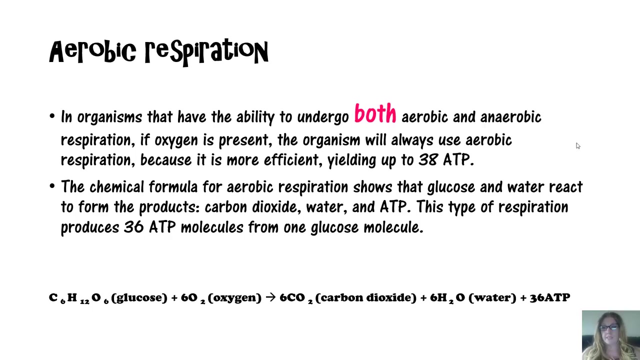 humans, as well as some prokaryotes, In organisms that have the ability to undergo both aerobic and anaerobic respiration. If oxygen is present, the organism will always use aerobic respiration because it is more efficient, yielding up to 38 ATP. 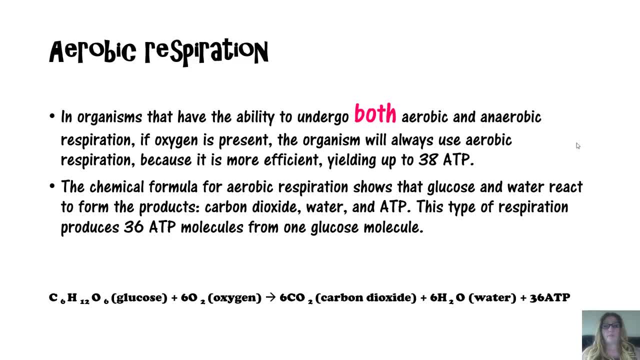 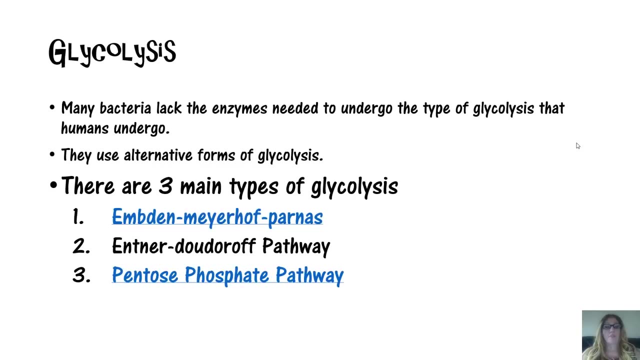 molecules. The chemical formula for aerobic respiration shows that glucose and water react to form the products carbon dioxide, water and ATP. This type of respiration produces 36 ATP molecules from one glucose molecule. Many bacteria lack the enzymes needed to undergo the type of glycolysis that humans. 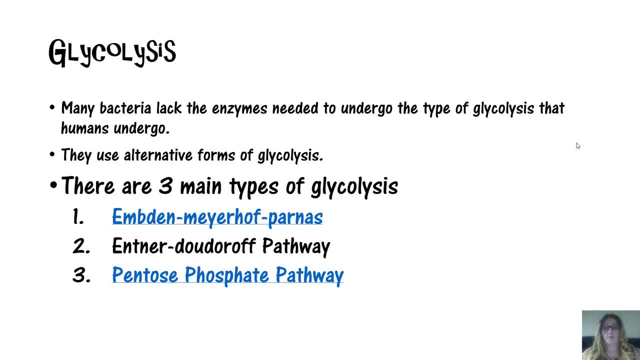 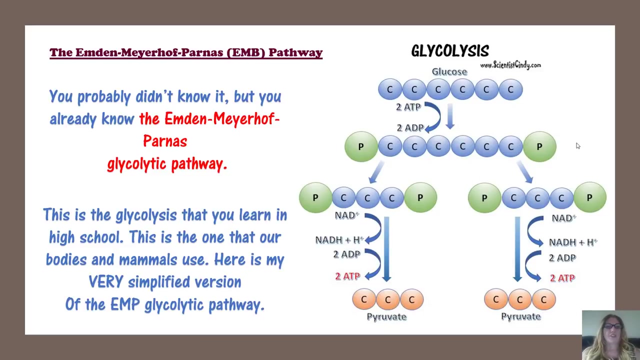 undergo, They use an alternative form of glycolysis. There are many more, but we'll only talk about three main types of glycolysis: The EMP, The EMP glycolysis pathway, the ED pathway and the PP pathway. I'm so immature. 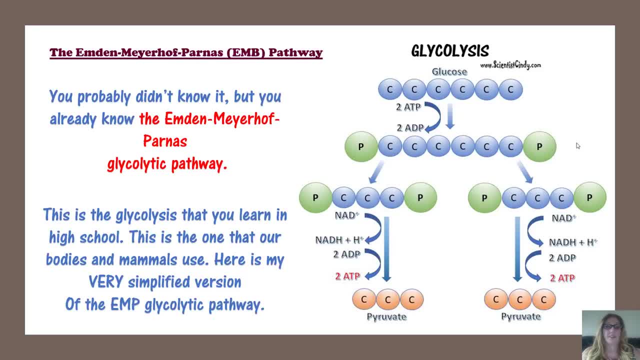 The EMB pathway. you probably didn't know it, but you already know the EMB pathway. This is the glycolysis that you learned in high school and also that I reviewed at the beginning of the video. This is the one that we use as humans. This is the one. 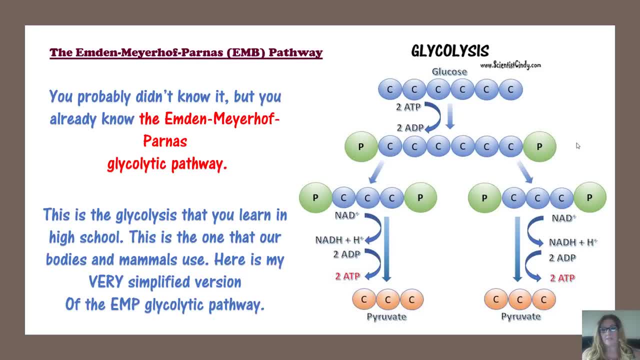 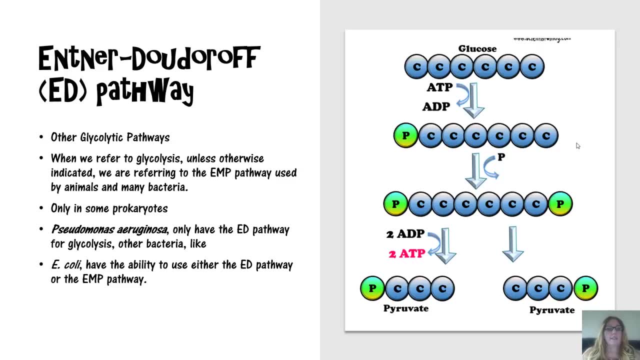 that mammals use. This is my again very simplified version of glycolysis. Now, this is the ED pathway of glycolysis, or the interdorof pathway. I think I'll stick with the ED pathway When we refer to glycolysis. 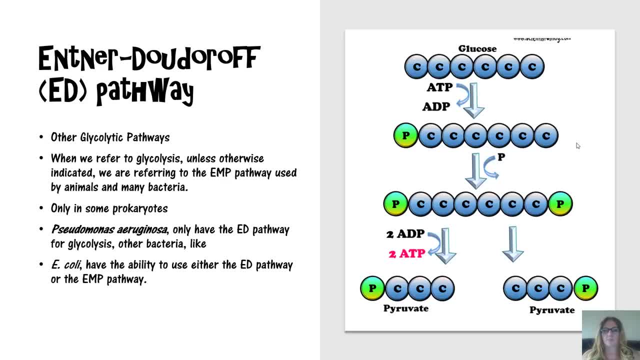 unless stated otherwise, you can just assume that we mean the EMP pathway, But the ED pathway is only in some prokaryotes, not even in all prokaryotes. So where can we find this? We find the ED pathway in bacteria such as. 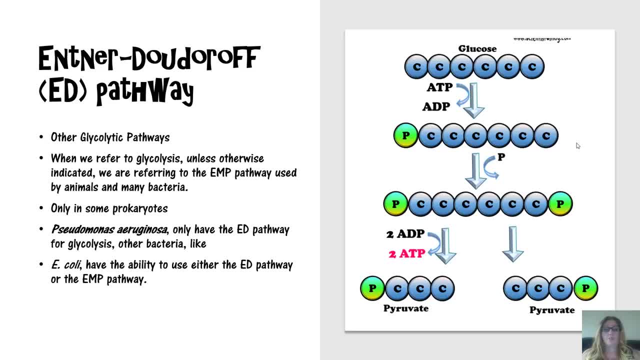 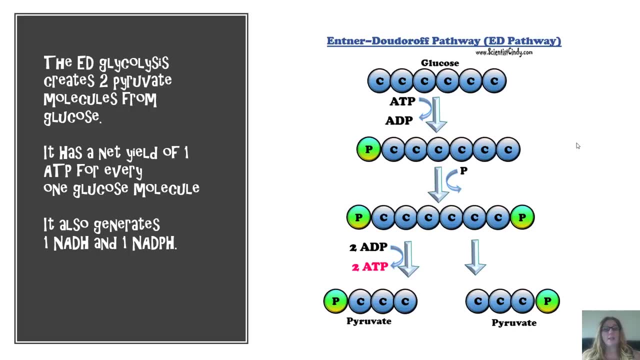 the Pseudomonas aeruginosa, Also E coli, are interesting because they have the ability to undergo either the ED pathway or the EMP pathway, which is kind of interesting. The ED glycolysis actually creates this, still creates two pyruvate. 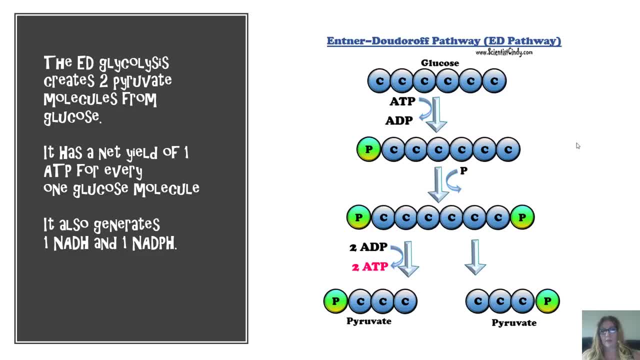 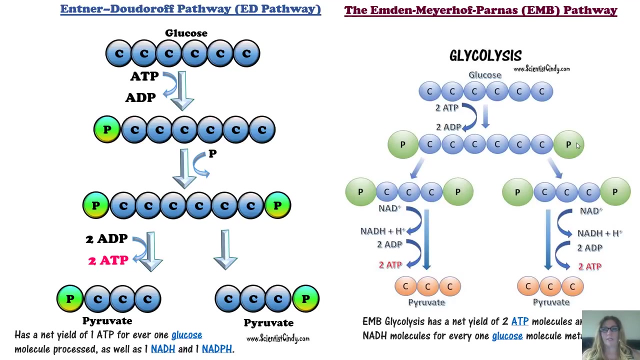 molecules from glucose, just like the EMP pathway does, But it has a net yield of only one ATP for every one glucose molecule. It also generates one NADH and one NADPH. So let's just do a quick side by side comparison between the EMP pathway. 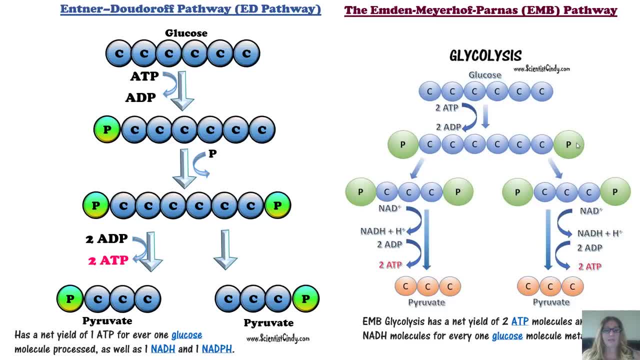 and the ED pathway. So the ED pathway has a net yield of one ATP and one NADH and one NADPH, versus the EMP glycolytic pathway has a net yield of two ATP, two NADH and that's it. So you actually get more ATP. 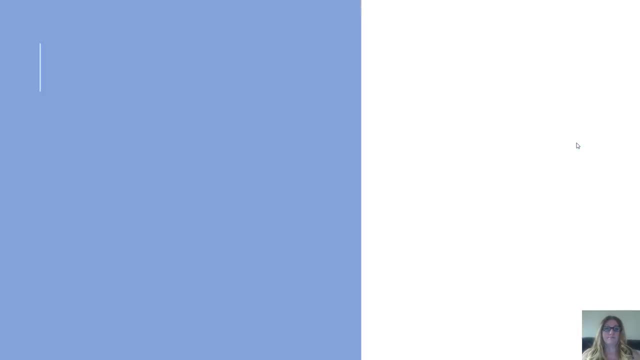 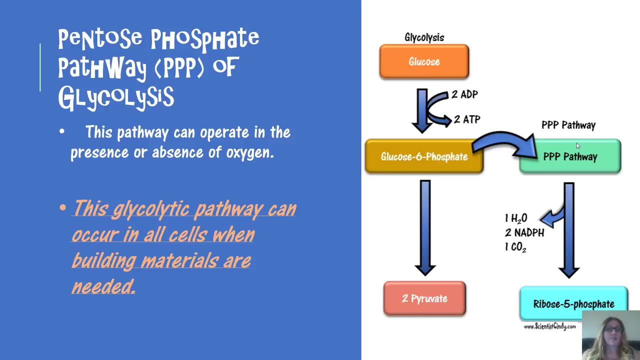 with the EMB pathway And, my favorite, the PP pathway. It's hard to say that without laughing. So the PP pathway, or pentose phosphate pathway, if I wanted to try not to laugh. This pathway can operate in the presence or absence of oxygen. 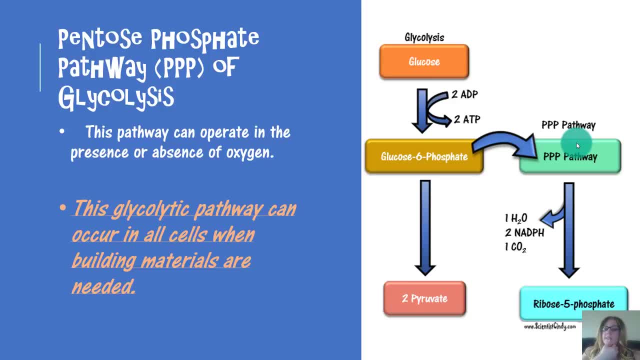 This pathway is something that can be activated in every cell in every organism, So it's a glycolytic pathway that can occur in all cells whenever building materials are needed. So if our bodies need to reconstruct a part of a damaged cell, and they're. 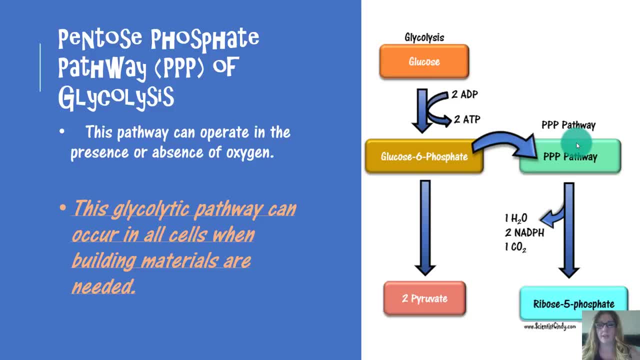 finding that they don't have the building materials necessary, then the pentose phosphate pathway will become activated. Now, in the schematic that I have here, this first group here, this is actually the cellular respiration, the normal pathway that I talked about at the beginning. So it starts with our glycolysis. 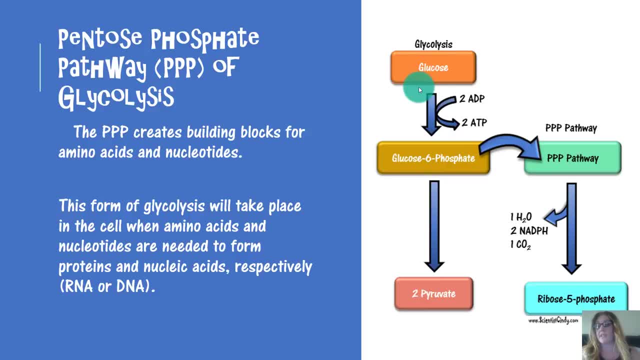 and then glucose 6-phosphate is an intermediate in the glycolysis pathway. Now glucose 6-phosphate, that intermediate that is produced during glycolysis, is actually going to branch off and go through the PP pathway. Now, during the PP pathway, you will 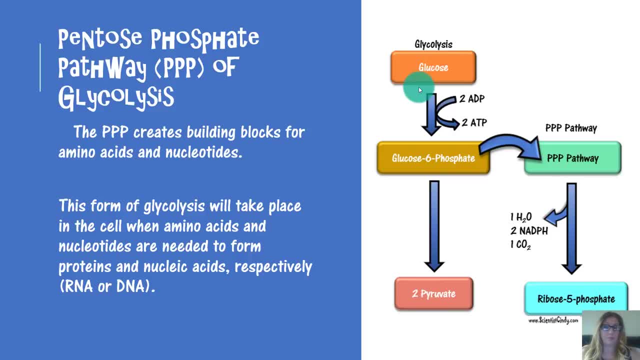 end up with? you will end up with ribose 5-phosphate and one water molecule, two NADPH, which is an electron carrier, and one carbon dioxide molecule. So the pentose phosphate pathway is going to create building blocks for amino acids and nucleotides. 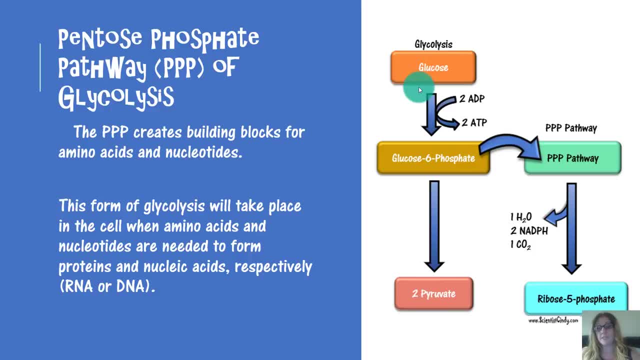 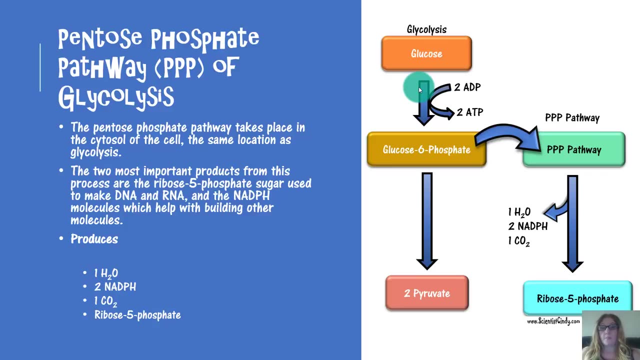 This form of glycolysis will take place in the cell whenever amino acids and nucleotides are needed to form new proteins and new nucleic acids, respectively for DNA or RNA. Now, the pentose phosphate pathway takes place in the cytosol of the cell. 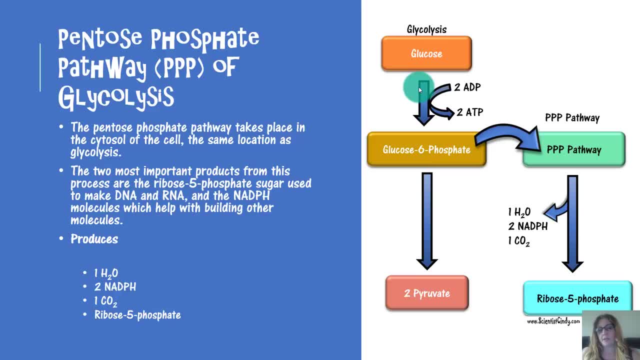 or you could say cytoplasm. that would be fine too. The pentose phosphate pathway takes place in the cytosol or cytoplasm of the cell, which is the same location as the other types of glycolysis would take place. The two most important products. 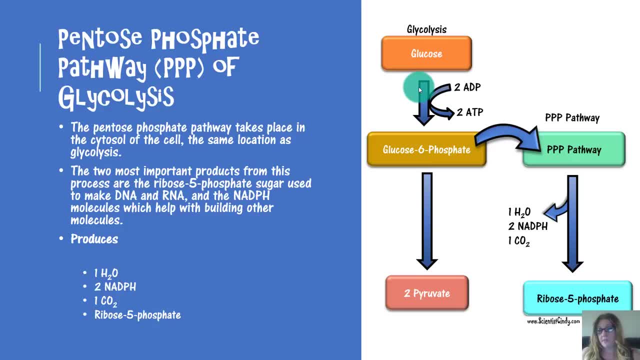 from this process are the ribose 5-phosphate sugar, which is a protein that is used to make DNA and RNA, but it also makes NADPH, which the NADPH is going to help with building other additional building blocks which will go on to build. 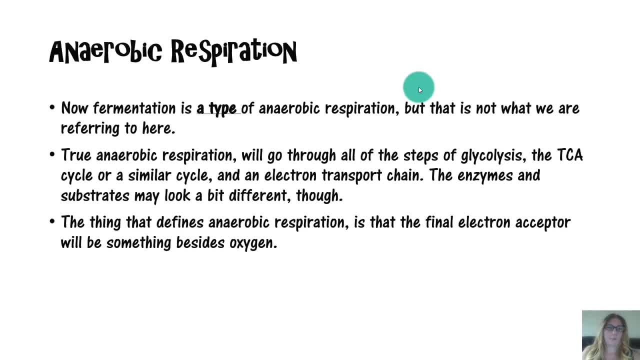 other macromolecules. Now, fermentation is a type of anaerobic respiration, but that is not always what we are getting to. so true anaerobic respiration will go through all of the steps of glycolysis, the TCA cycle or a similar cycle. 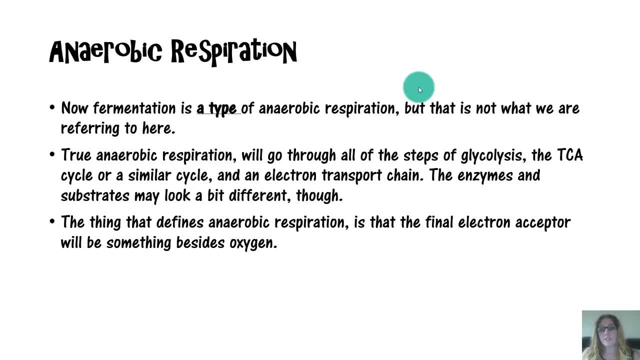 to TCA that is just modified and an electron transport chain. The enzymes and substrates might look a little bit different, though The thing that defines anaerobic respiration is that the final electron acceptor will be something besides oxygen, For example. let's look at 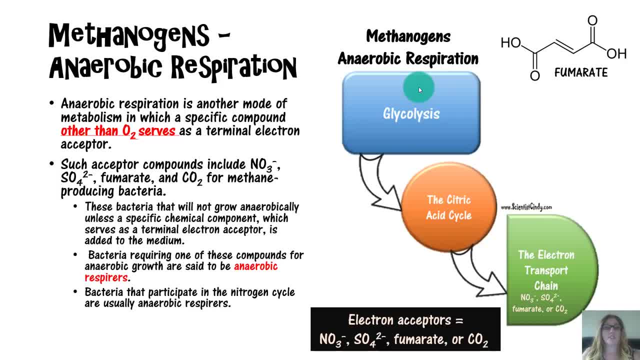 methanogens. Anaerobic respiration is another mode of metabolism in which the specific compound other than oxygen serves as the terminal or final electron acceptor. Such acceptor compounds include nitrate, nitrite, sulfate, fumarate and carbon dioxide. for your. 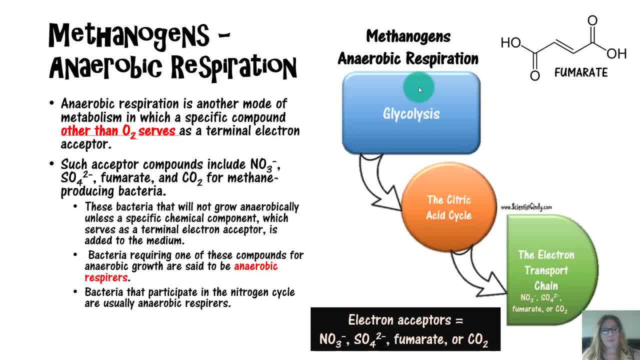 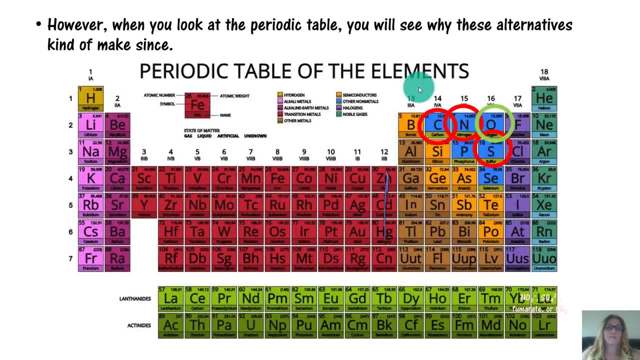 methane producing bacteria like we have here. I've already read this slide, didn't I? I certainly did. Now what's kind of interesting is, if you look at these alternates, these other alternates are actually pretty close to oxygen, which is kind of interesting. 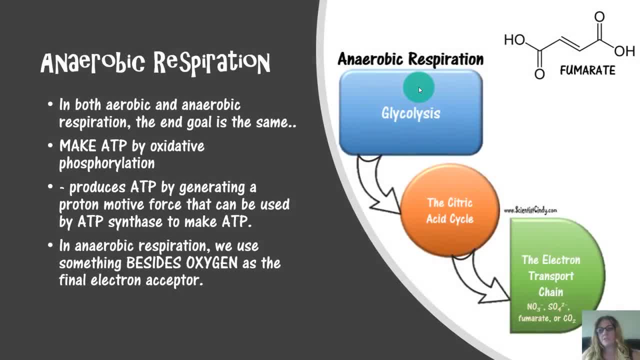 So it's not too much of a stretch of the imagination that these other compounds would be used in a similar fashion in other similar metabolic pathways in other organisms. So in both aerobic and anaerobic respiration the end goal is still the same: to make ATP. 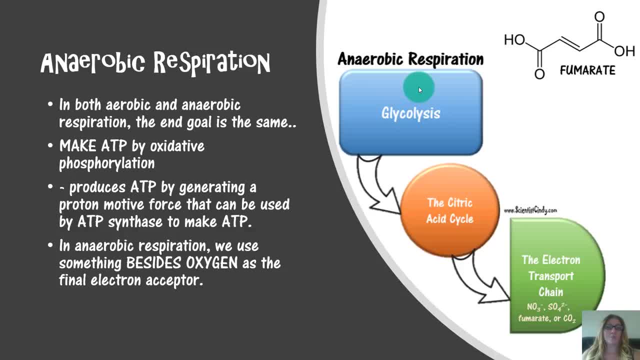 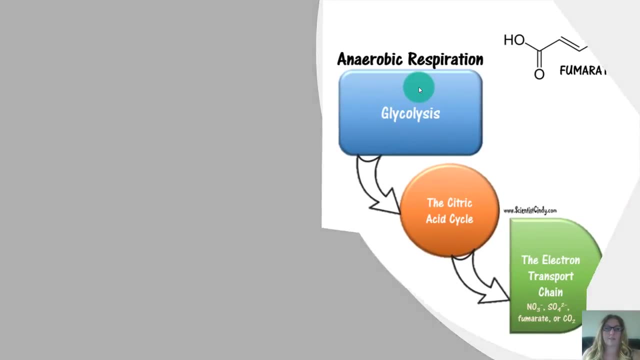 by oxidative phosphorylation, which produces ATP by generating a proton motive force that can be used by the ATP synthase to make ATP. In aerobic respiration, we use something besides oxygen as the final electron acceptor. Boy. I've said that a lot, so that's really going to be. 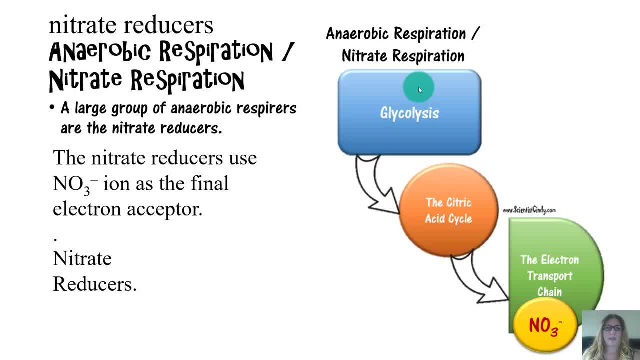 on your mind Now. another important group of anaerobic respirers are our nitrate respirers. This is a large group of anaerobic respirers and they, these nitrate reducers, are going to use nitrate nitrite actually as the final electron. 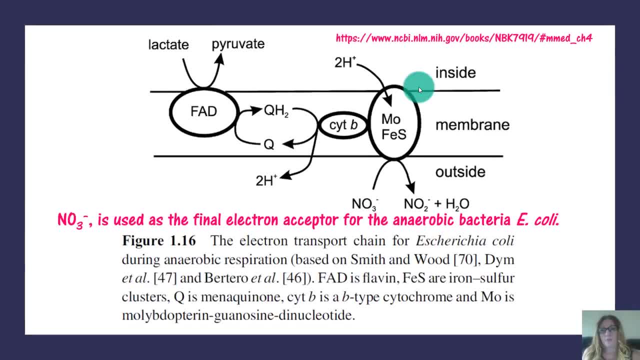 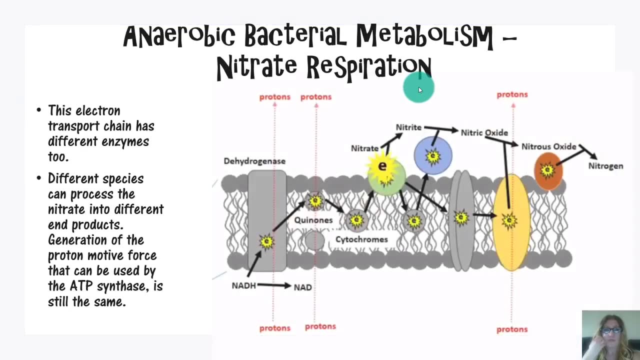 acceptor. Don't worry about the specifics, but I thought this was kind of cool. So this is actually the electron transport chain for E coli during the process of anaerobic respiration. This is another schematic for the anaerobic bacterial metabolism. 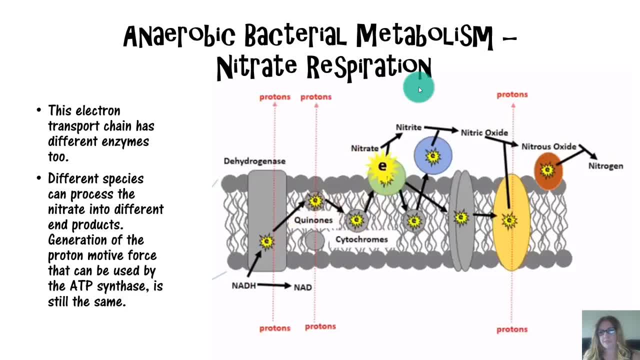 of nitrate respiration. But you don't have to worry about all these little things, but just thought it was kind of cool, Thought you might be interested. This electron transport chain also does have different enzymes than we see in the electron transport chain that we looked at earlier. 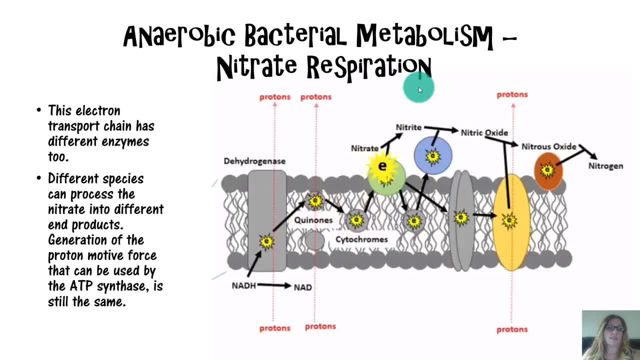 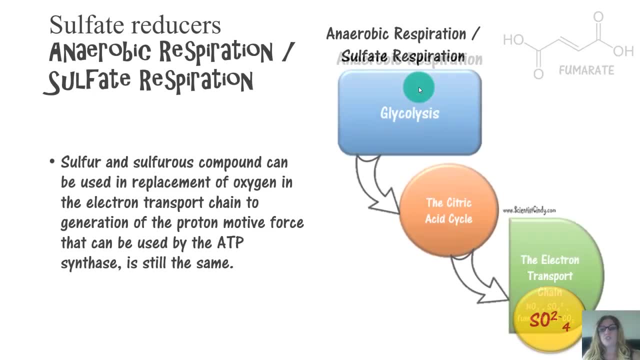 Different species can process the nitrate into different end products. The generation of the proton motor force that can be used to used by the ATP synthase is still the same, So the general concept is always still the same. Now our sulfate reducers are another group of our anaerobic 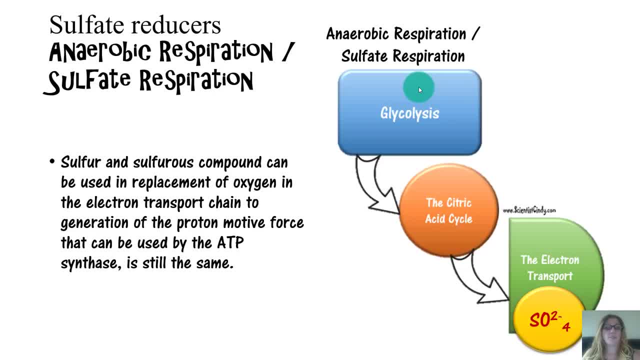 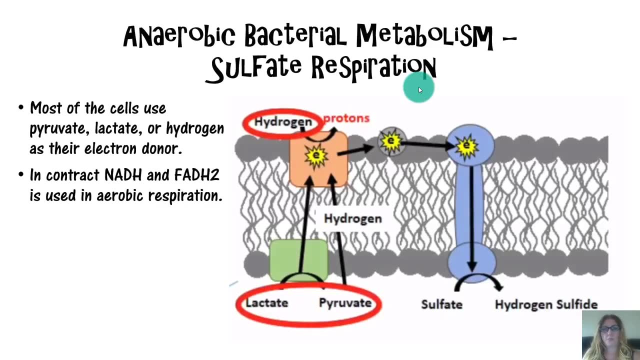 respirers, And here you're going to have some type of sulfur or sulfurous compound- is going to be used as the replacement for oxygen, as the final electron acceptor, And here is a schematic of what their electron transport chain looks like: Very, very different. 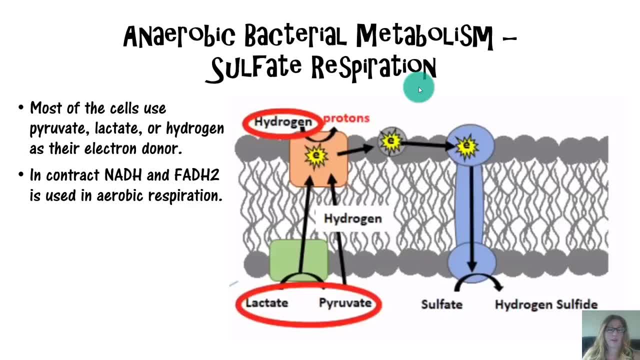 So most of the cells here actually will use pyruvate lactate or hydrogen as their electron donor to the electron transport chain. So that's supposed to say in contrast, not in contract, In contrast NADH and FADH2. 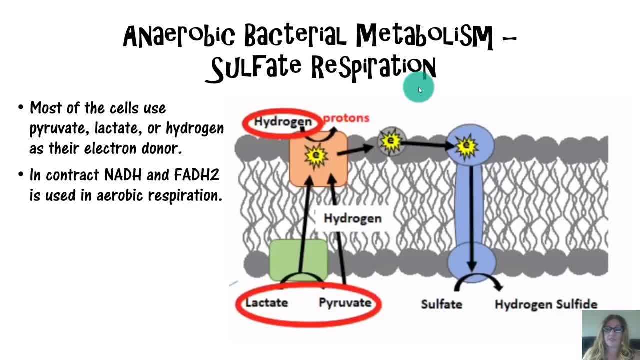 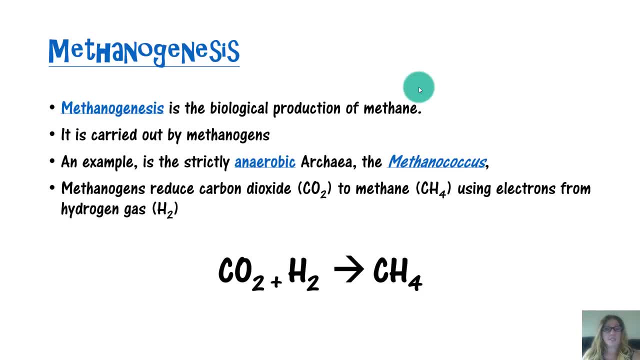 is used in aerobic cellular respiration, So the electron carriers are very, very different in sulfate respiration, which is kind of interesting. In methanogenesis these are our anaerobic bacteria and our archaea that are methane producers, like the ones. 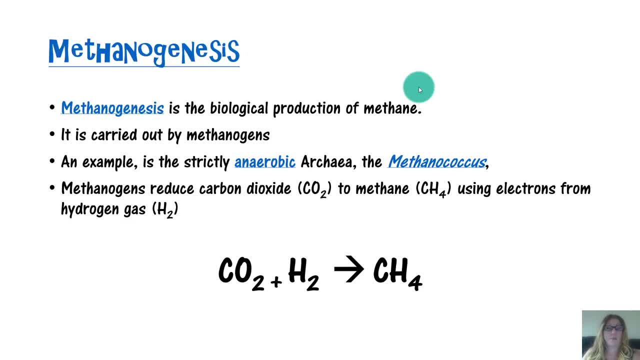 that exist in the rumen of cows, for example. So methanogenesis is the biological production of methane. This is a byproduct of the microbial metabolism for these methanogens, And one of the archaea that undergoes methanogenesis is methanococcus. 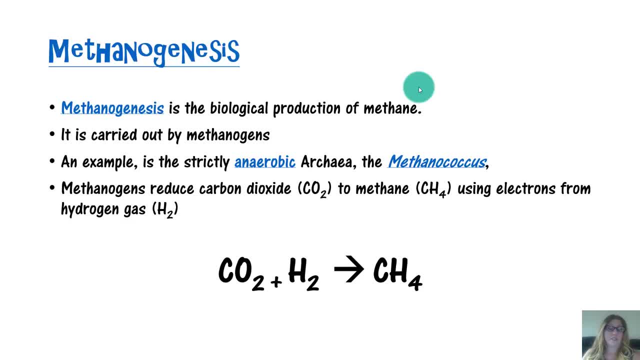 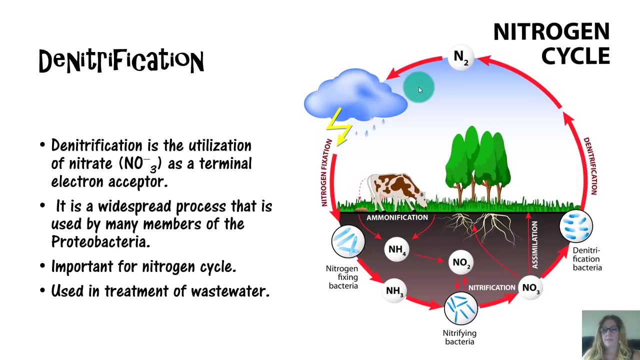 I guess it's aptly named, right? So methanogens metabolize by reducing carbon dioxide, and I have the equation here: They reduce carbon dioxide to methane and they do this by using electrons from hydrogen gas. We have a lot of bacteria which are really 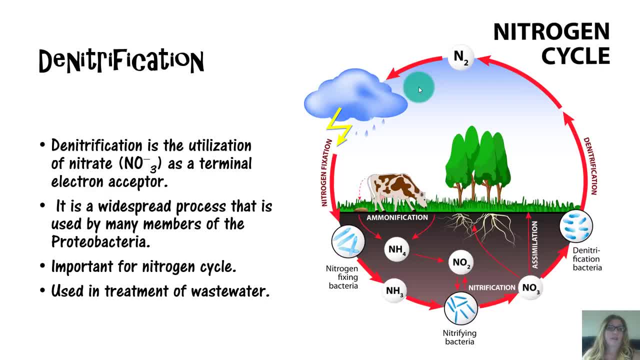 important to the nitrogen cycle. We have bacteria which are involved with actually each of these phases. So you've got your nitrogen fixing bacteria, your nitrifying bacteria and your denitrification bacteria. So bacteria are important for every phase of the nitrogen cycle. 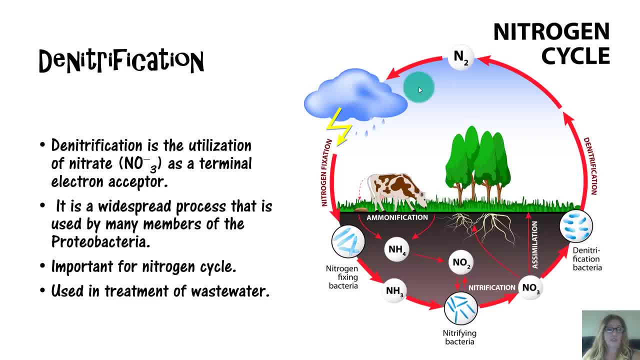 So denitrification is the utilization of nitrate, which is NO-3, and as a terminal electron acceptor. So this is when it is going through the anaerobic cellular respiration process and using nitrate as the terminal electron acceptor. It is a 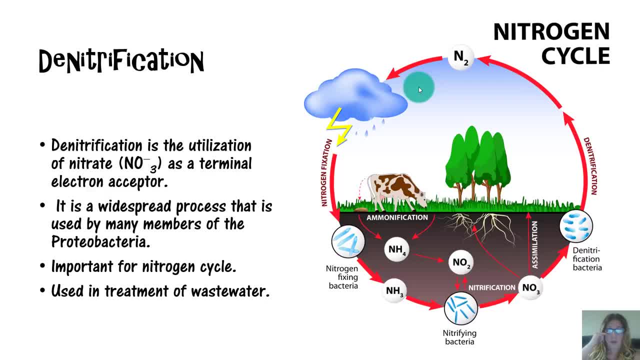 widespread process that is used by many members of our proteobacteria. So our phylum, the proteobacteria, use this. This is important for nitrogen cycling and it's also used for wastewater treatment. So what is the nitrogen cycle? So, the nitrogen cycle. 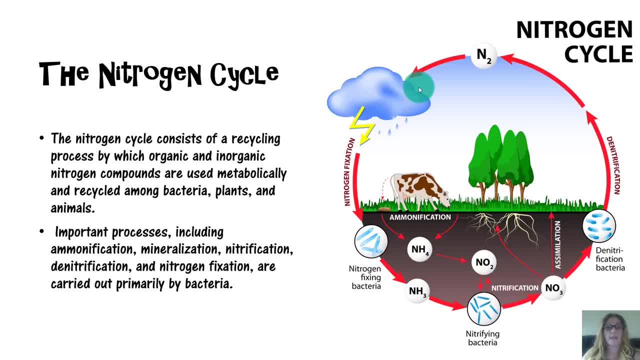 consists of a recycling process by which organic and inorganic nitrogen compounds are used metabolically and recycled among bacteria, plants and animals. Important processes include ammonification, mineralization, nitrification, denitrification and nitrogen fixation, And all of these are carried. 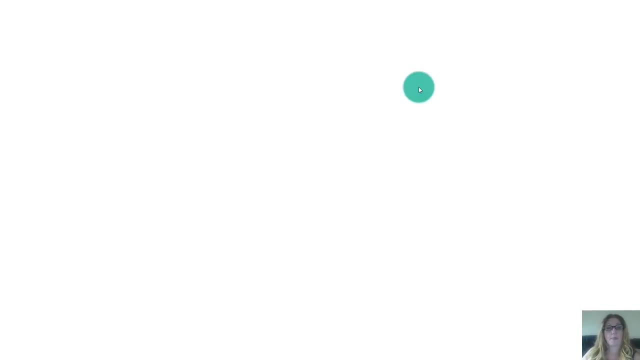 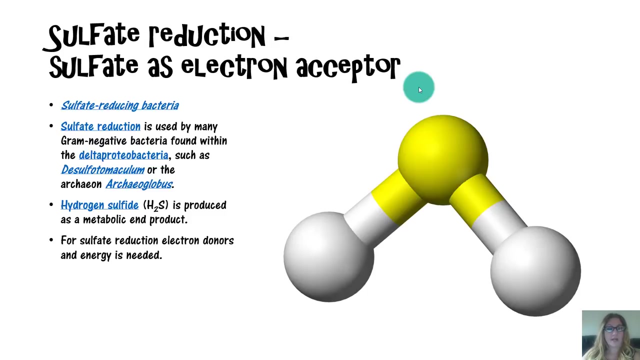 out primarily by bacteria. Let's look at our sulfate reducers. Are sulfate reducing bacteria? Sulfate reduction is used by many gram-negative bacteria, and these gram-negative bacteria are found in the Delta Proproteobacteria group, such as the desulfo-. 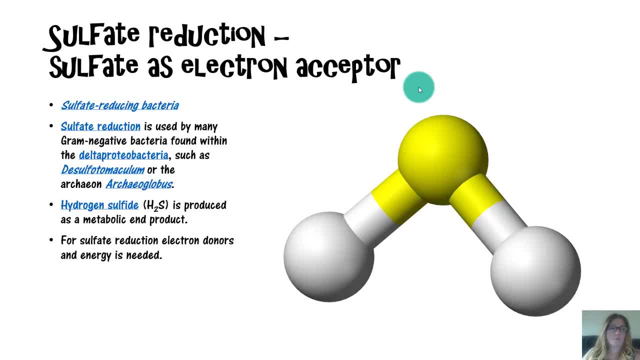 to maculum, Desulfo- to maculatum- I can't say that Desulfo-to maculum- There that's a little bit better- Or the archaea, or the archaean archaeoglobus. Hydrogen sulfide is. 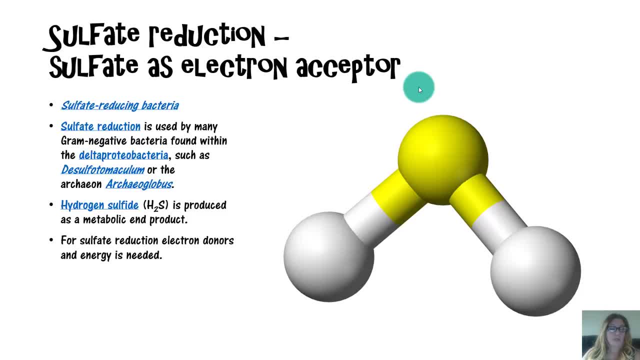 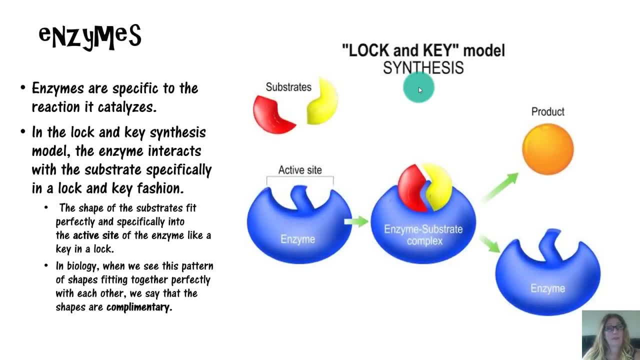 produced as a metabolic end product. For sulfate reduction, electron donors and energy is needed. Enzymes are needed to catalyze all of these different reactions. How a lot of these are done is through what we call the lock and key synthesis model. 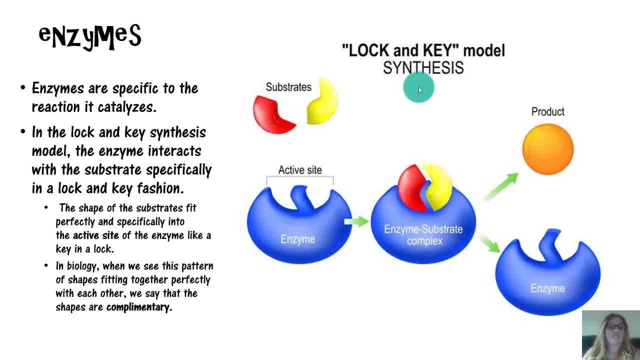 Enzymes are specific to the reaction that it catalyzes. In the lock and key synthesis model, the enzyme interacts with the substrate specifically in this lock and key sort of fashion. The shape of the substrates fit perfectly and very specifically into the active sites. 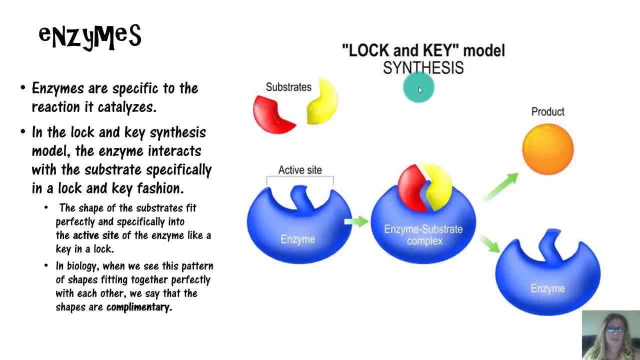 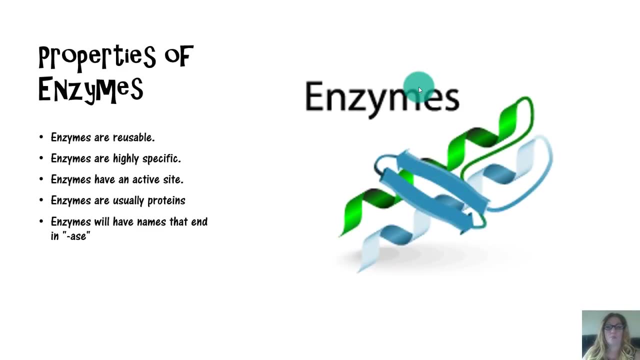 of the enzymes like a lock and key. In biology we see this pattern of fitting shapes together. We call this the complementary fit. So properties of enzymes. Enzymes are reusable, They are highly specific, They have an active site. 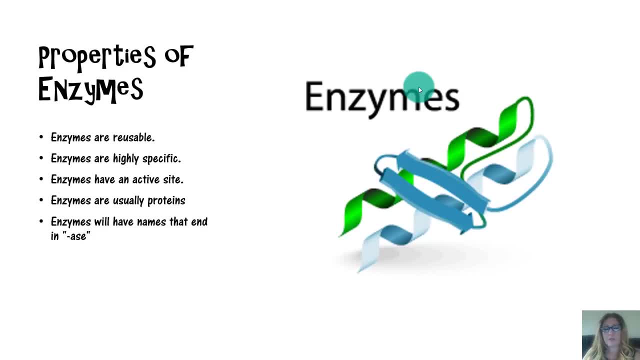 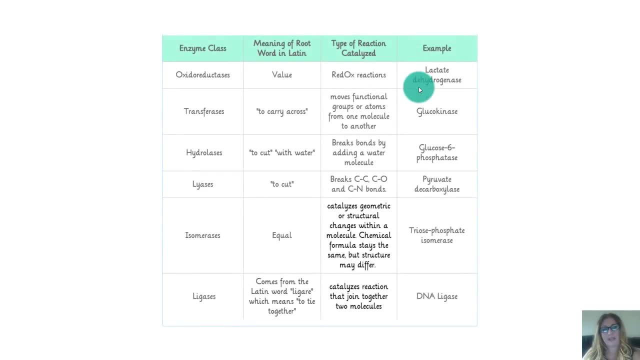 They are usually proteins and you can always recognize an enzyme just by its name, because it will end with A-S-E. It will end in A-S-E. Here's some examples of enzyme names. They will always end with A-S-E and the beginning of their name. 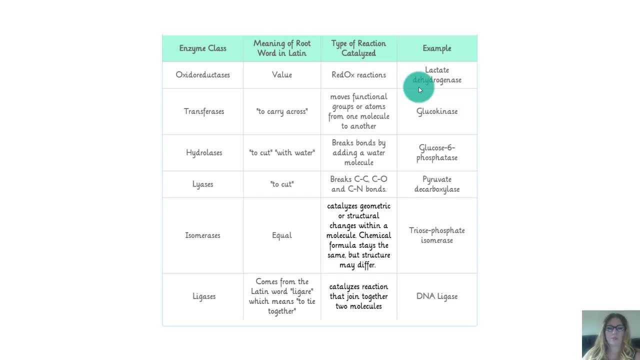 will always have something to do with their function, either what it does or what it acts on. For example, if it transfers something, then it might be a transferase. If it cuts with water, maybe it's a hydrolase. 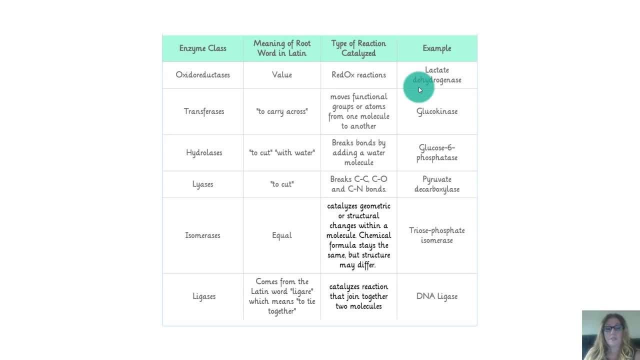 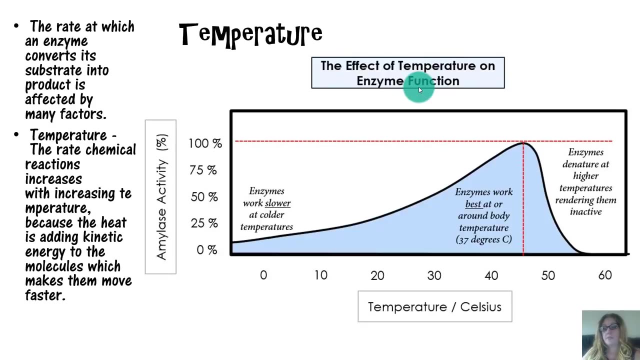 If it brings things together, glues things together, maybe it's a ligase. There are a few things that do affect the function of enzymes. Without our metabolic processes, we die. This is true for all organisms. If you have an organism, 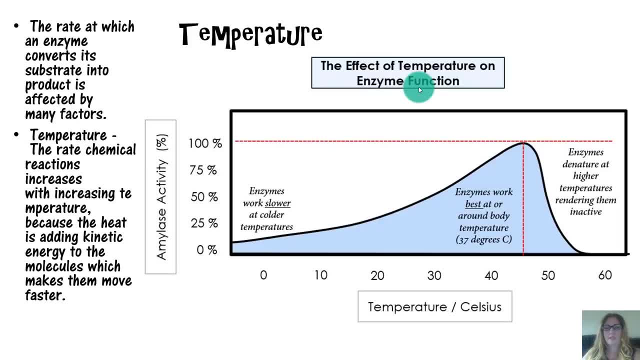 that you can kill its enzyme function. you have killed the organism, All of the metabolic functions, all those different steps and reactions of the process. almost all of them need specific enzymes for each of those. If you were to kill an enzyme, 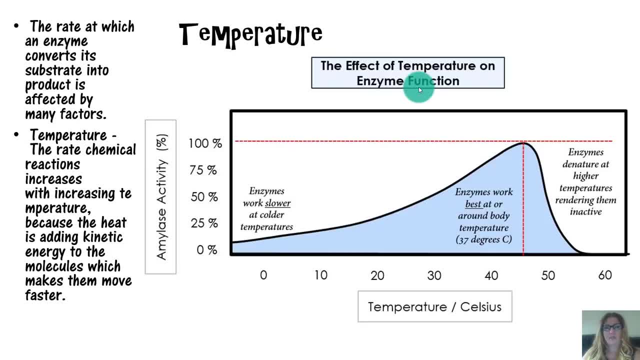 or kill those enzymes, you would kill the individual organism as well, which is one of the reasons why we care about this. This slide is particular to amylase, which is found in saliva in humans. That's why this says: enzymes work best around. 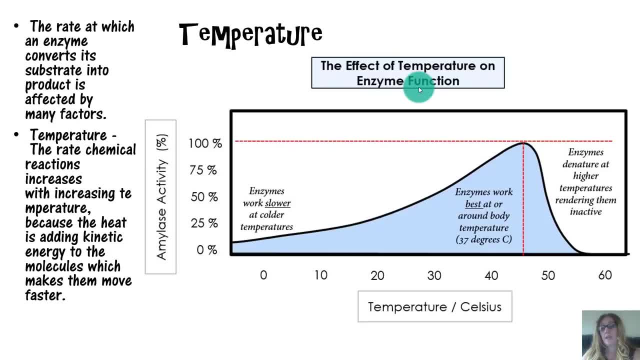 body temperature of humans, which is 37 degrees Celsius. However, if we're looking at an enzyme in an organism that is a psychophile and loves it at 10 degrees Celsius, which would be way too cold for me, then I'm sure that the enzymes 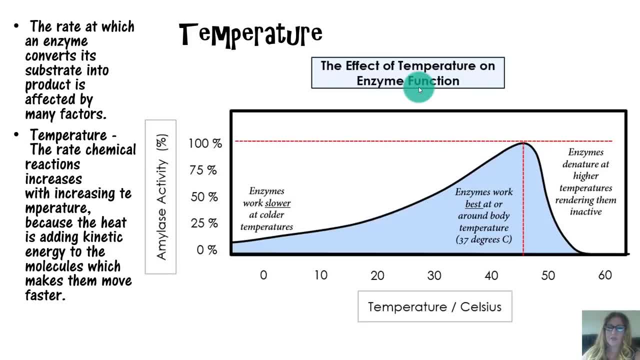 will have an optimal temperature that is much, much lower than that. Whatever the optimal temperature of that organism is is going to be right around the optimal temperature for that enzyme. It just makes sense. It has evolved that way for a reason, and 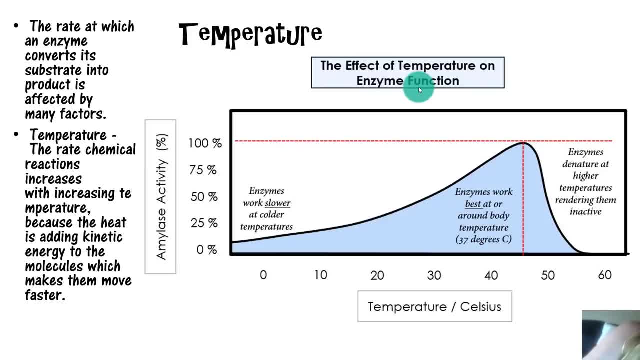 it's going to be its optimal function Alright. So the important thing here is: if you really look at this, you can also relate this to what we really see with organisms, too, with microbes. When you get a microbe really cold, 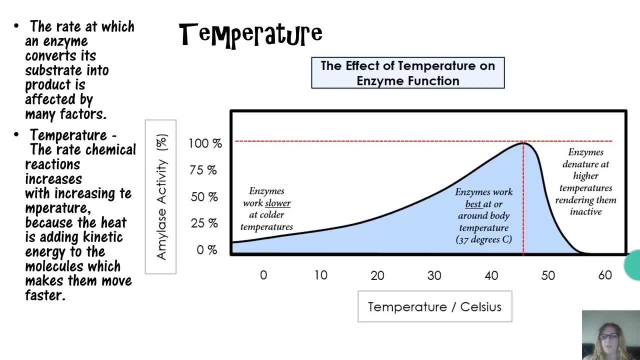 you usually don't kill it, You just put it into a state of hibernation, Which makes sense, because if you look at what happens to the enzymes of that organism, the enzymes are not degraded, they're not destroyed, they're just slowed down. 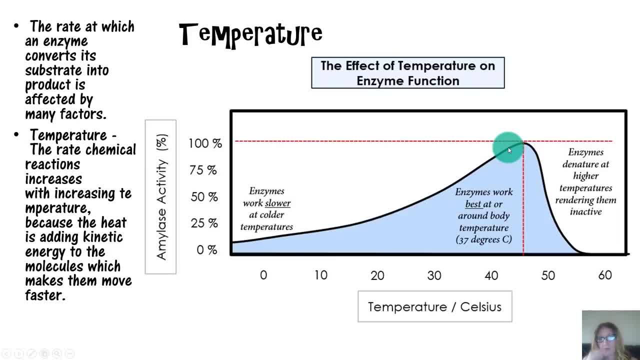 So when I get, for example, when I put something in the freezer, I have slowed down its decaying process. I've slowed down the growth of whatever bacteria might be rotting my food by putting it in a cold environment. Now, if I want to kill, 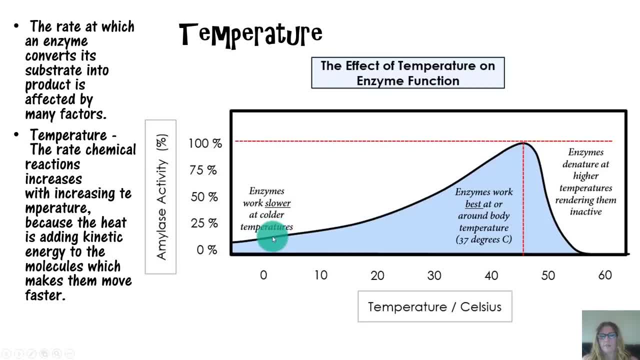 bacteria. if I want to kill bacteria, then what I need to do is I need to heat it. Now, of course, if it's an endospore, they're resistant to heat, so I'm going to have to really heat it. 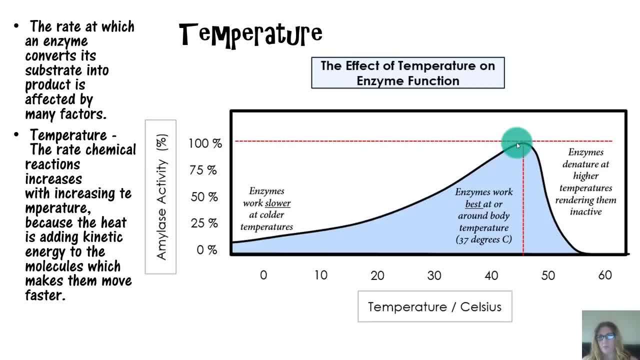 121 degrees Celsius with moist heat in an autoclave. So with 15 minutes, right 15 to 20 minutes, so it's a lot. But what happens with heat, depending on the organism and depending on the? 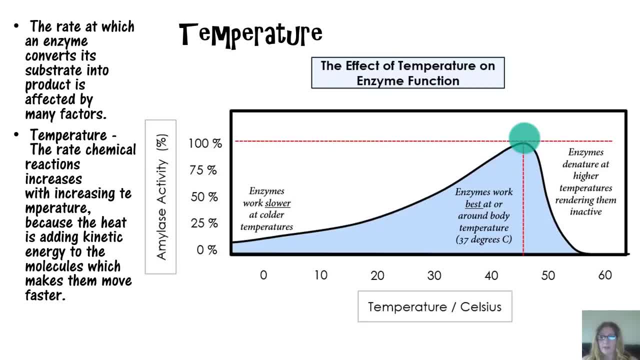 enzyme. if I can heat it hot enough, then I degrade the enzyme. And because it's a protein, once I degrade the enzyme I've killed that tertiary structure. it's not coming back. So I've essentially killed the enzyme and killed the creature. 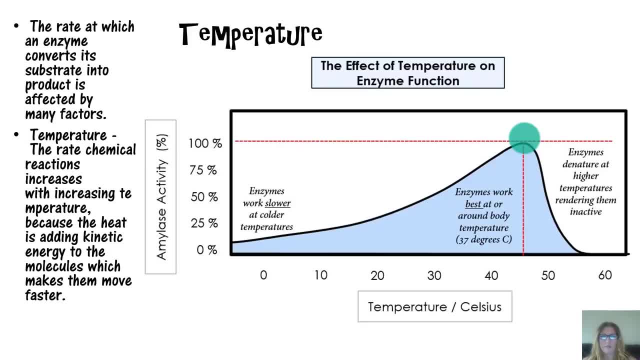 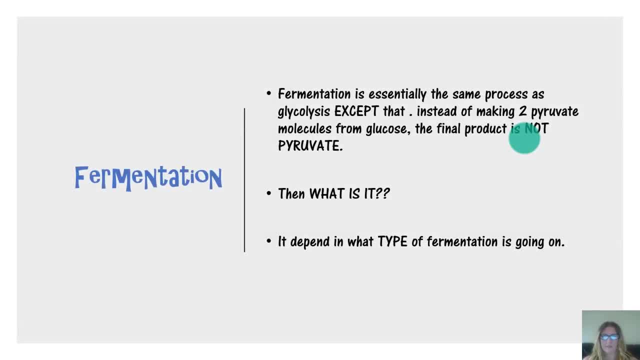 So this is one of the reasons why we talk about the function of enzymes and what they are sensitive to, because it is very relevant. Okay, Alright, so fermentation Now fermentation is. fermentation is essentially the same process as glycolysis, except instead of making. 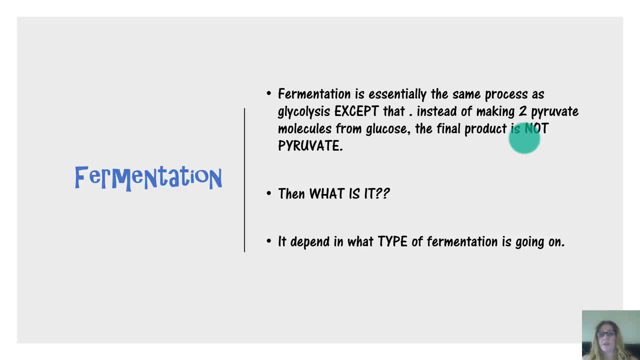 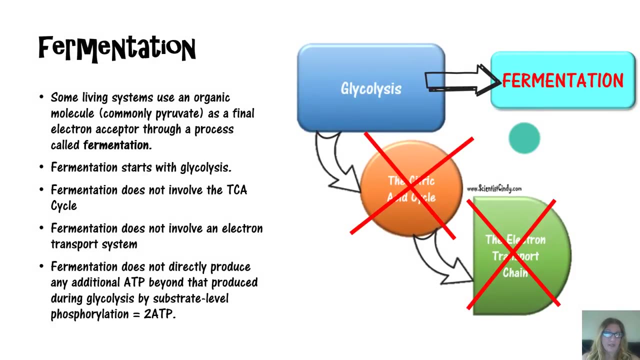 two pyruvate molecules from glucose, the final product is not pyruvate. Then what is it? So depends on the type of fermentation going on. So let's see what that is. So fermentation does not go through. 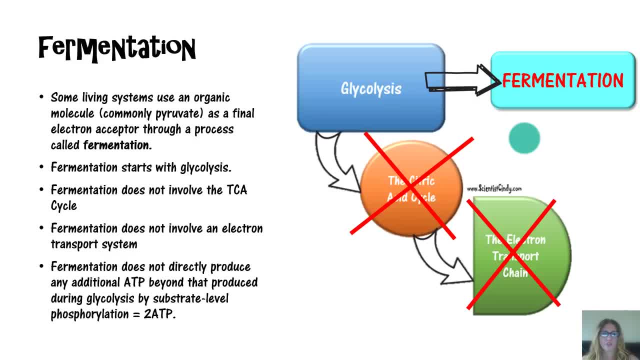 the citric acid cycle or the electron transport chain. Okay, So glycolysis, it does go through glycolysis, and remember, glycolysis does not need oxygen. Okay, it's an anaerobic process. So we go through glycolysis and then straight. 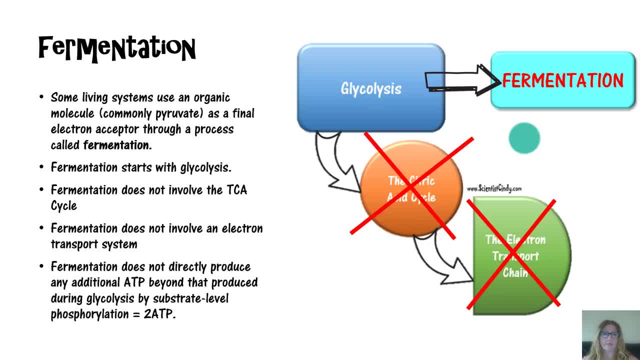 to fermentation, of whatever type of fermentation, it is Okay. So fermentation does not produce any ATP on its own, It only produces. I mean, it itself does not produce anything. So the ATP that is produced is just produced in glycolysis. 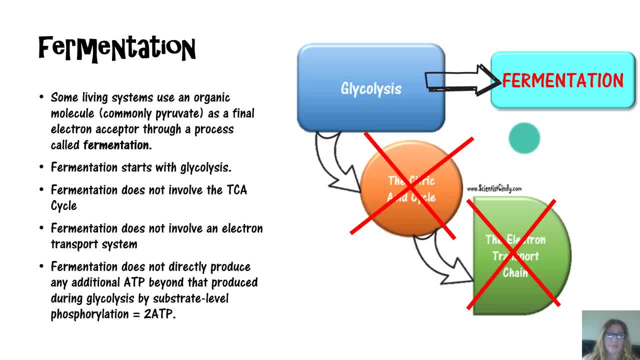 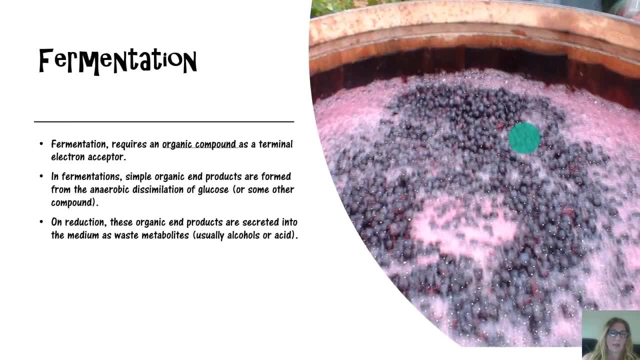 So yeah, and that glycolysis produces the two ATP that it would have normally, Alright. So fermentation: what does it require So in fermentation? the definition of fermentation is when it has an organic compound As a terminal electron acceptor. 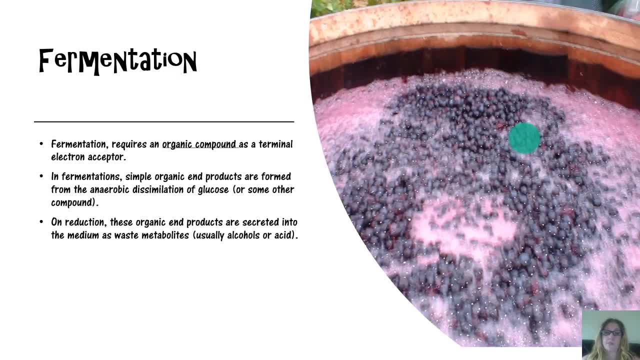 And usually that might be pyruvate, for example, as an electron acceptor. So in fermentations the simple organic end product is formed by the anaerobic dissimulation or taking apart of glucose or another similar compound. 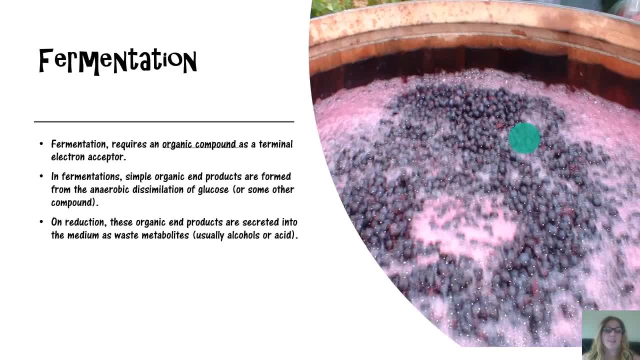 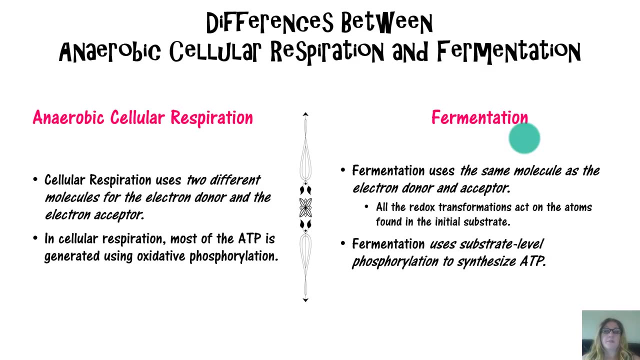 usually a carbohydrate. On reduction, these organic end products are actually secreted into the medium as waste products, as either alcohols or acids. So let's compare and contrast between the differences of anaerobic cellular respiration and fermentation. So anaerobic cellular 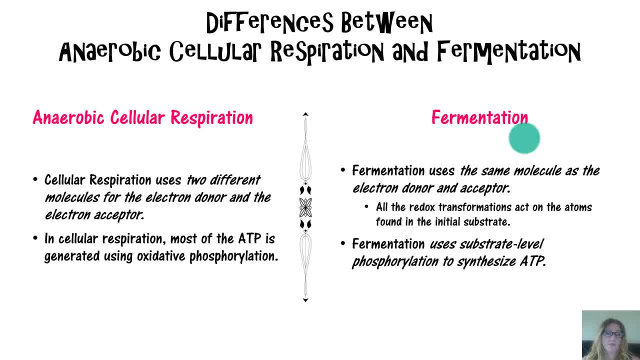 respiration. So cellular respiration uses two different molecules for the electron donor and the electron acceptor, Whereas fermentation uses the same molecule as the electron donor and the electron acceptor. So all the redox transformations act on atoms found in the initial substrate. 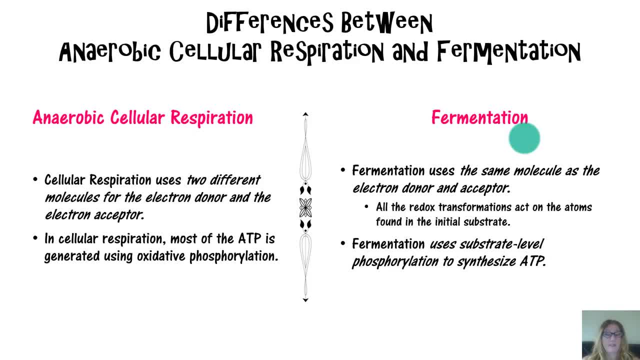 Anaerobic cellular respiration. Most of the ATP is generated using oxidative phosphorylation, That's in the electron transport chain In fermentation. fermentation only uses substrate-level phosphorylation, which is during glycolysis, to synthesize ATP, And we've seen this. 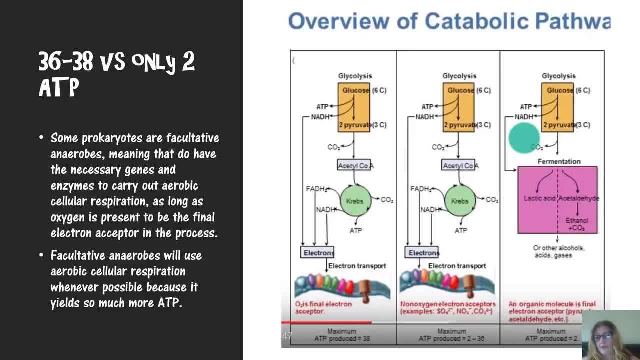 once before, but now that we've actually talked about all three of these different pathways, let's look at them again. So there's a wide variance, especially with this middle one here, where it says maximum ATP produced is anywhere between 2 and 36.. 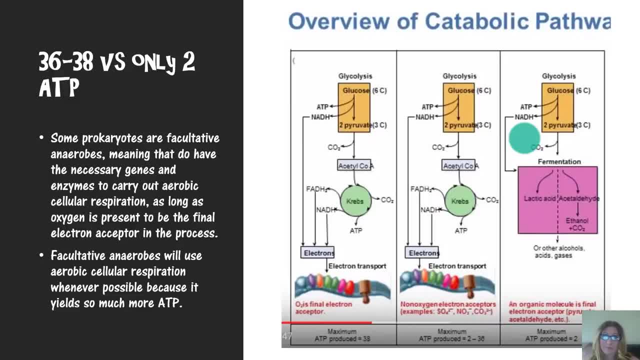 Molecules. right, There's a huge variance here. Yeah, Big difference. Fermentation: 2. 2 max. True anaerobic respiration just depends Anywhere from 2 to 36.. It's all over the place. 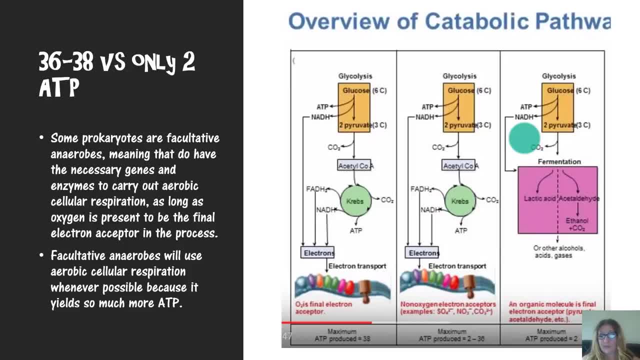 With aerobic cellular respiration a maximum of 38. On its best day. So some prokaryotes are facultative aerobes, meaning that they do have the necessary genes and enzymes necessary to carry out aerobic cellular respiration as long as oxygen is. 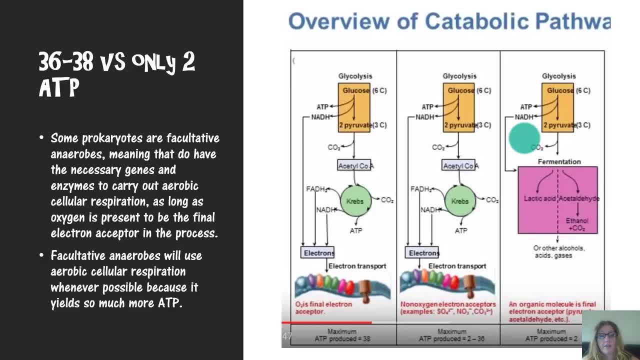 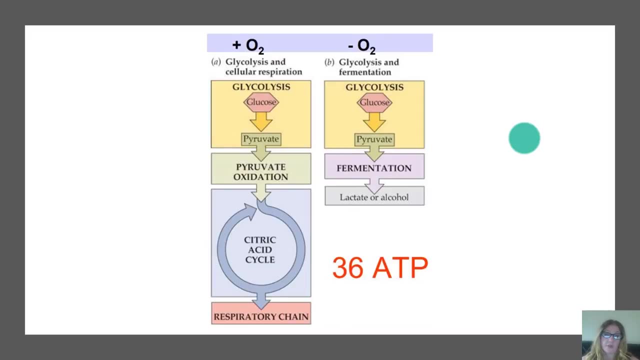 present to be the final electron acceptor in the process. Facultative anaerobes will use aerobic cellular respiration whenever possible, because it yields so much more ATP in most cases. So if I just look at glycolysis and cellular respiration, 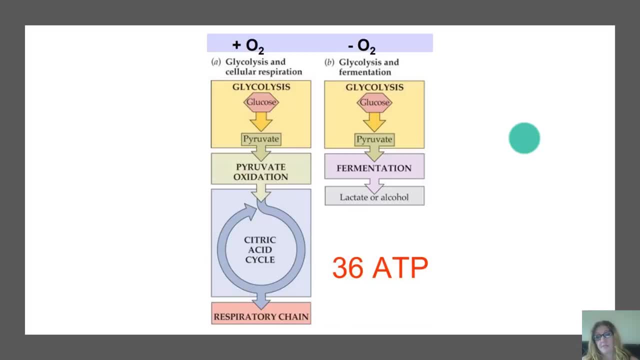 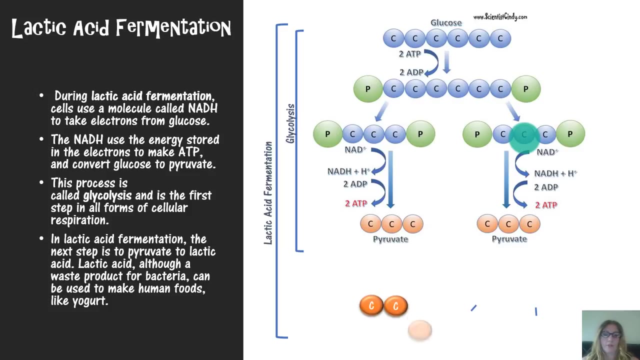 versus glycolysis and fermentation. there's a big difference. You're looking at 2 ATP versus 36 ATP, So yeah. So let's look at lactic acid fermentation. So, during lactic acid fermentation, cells use a molecule called NADH. 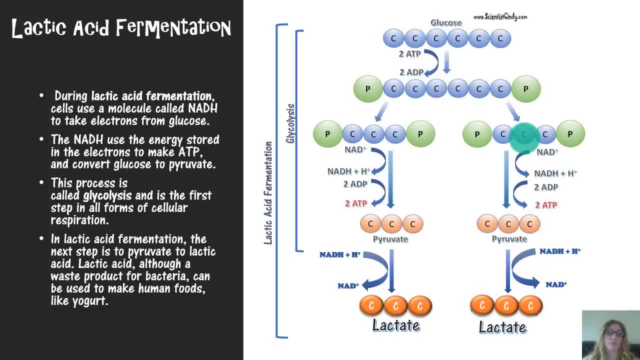 to transfer. I'm sorry to take electrons from the glucose molecule. The NADH uses the energy stored in the electrons to make ATP and converts glucose to pyruvate. This process is called glycolysis and is the first step in all forms. 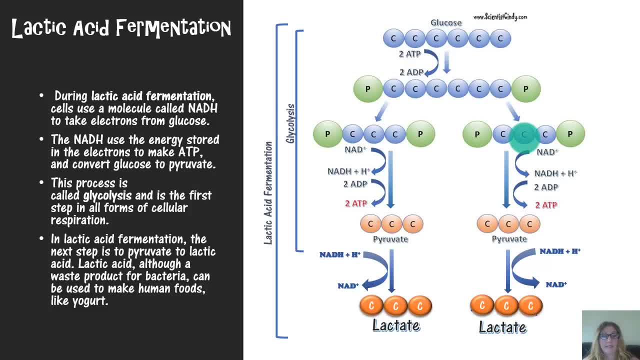 of cellular respiration In lactic acid fermentation. the next step is to convert pyruvate to lactic acid. Lactic acid, although a waste product for bacteria, can be used to make human foods like yogurt. Fermentation is most often triggered. 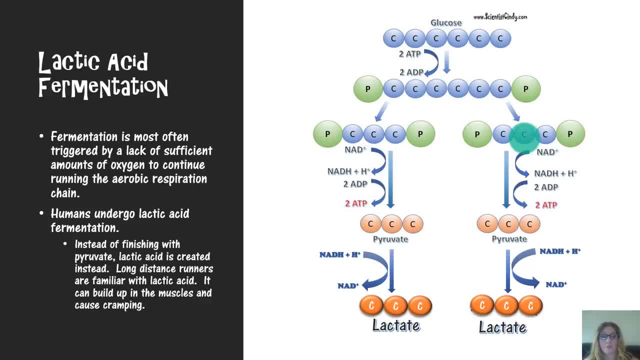 by a lack of sufficient oxygen to continue running. aerobic respiration, For example. humans undergo lactic acid fermentation instead of finishing with pyruvate. lactic acid is created instead inside of the muscles. Long distance runners are familiar with lactic acid. 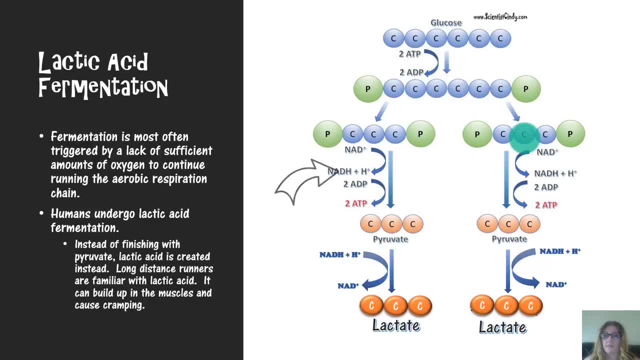 It can build up in the muscles and cause cramping. Another thing to note too, is that in glycolysis, NAD actually gets in fermentation. In fermentation we get a replenishment of the NAD plus molecule, which is really important to keep that. 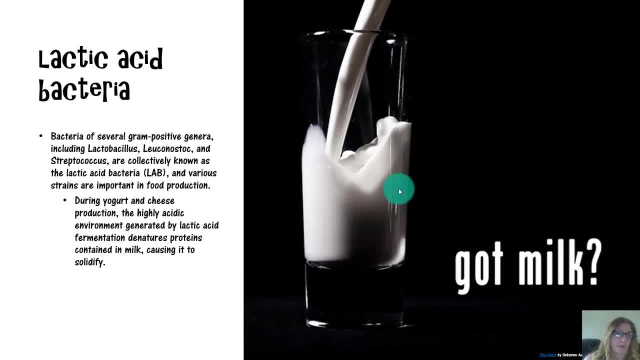 going. Lactic acid bacteria are really important for making yogurts and cheeses, for example. Um um. so bacteria of several gram-positive genre, including lactobacillus and leuconostoc and streptococcus, are collectively known as lactic acid bacteria. 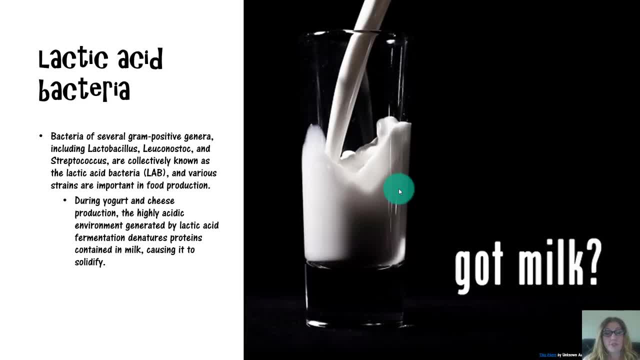 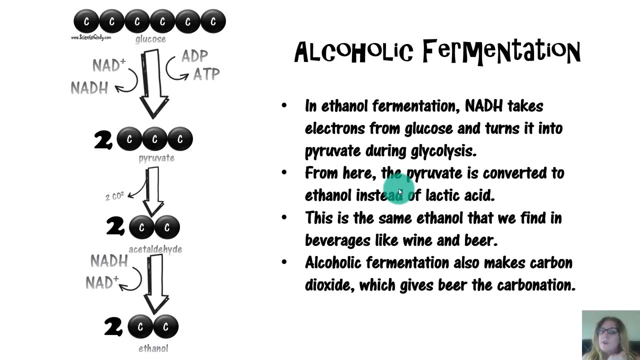 And various strains are important in food production. So during yogurt and cheese production, the highly acidic environment generated by the lactic acid fermentation acts to denature the proteins contained in milk, which cause it to solidify In ethanol fermentation or alcoholic fermentation, the NADH. 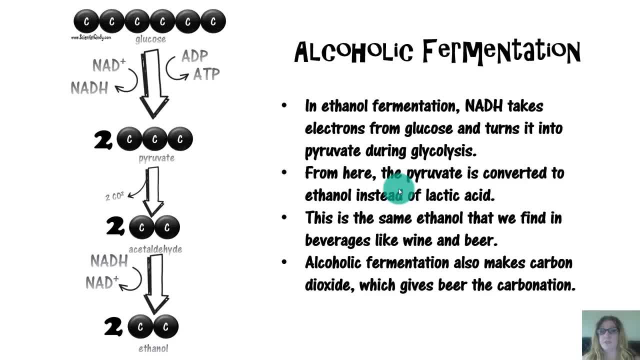 takes electrons from the glucose molecule and turns it into pyruvate during glycolysis. From here, the pyruvate is converted into ethanol instead of lactic acid, The same ethanol that we find in beverages like wine and beer. Alcoholic fermentation. 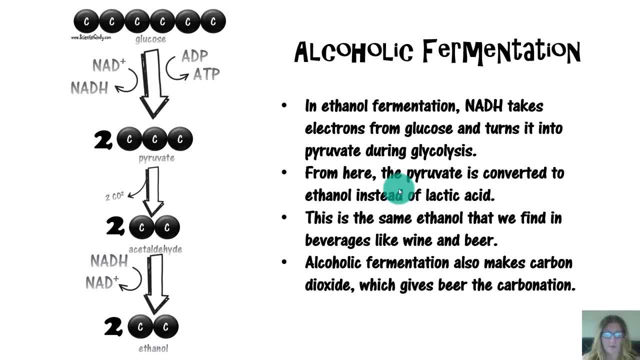 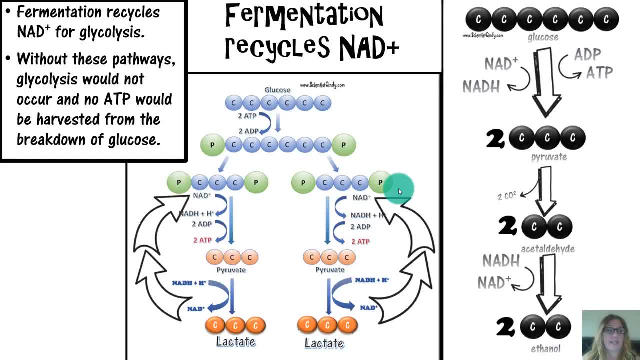 also makes carbon dioxide, which gives the beer its carbonation. Fermentation recycles that NAD molecule for glycolysis. So if it were not for the fermentation pathways then we would not have the NAD molecule to be recycled here for the glycolysis. 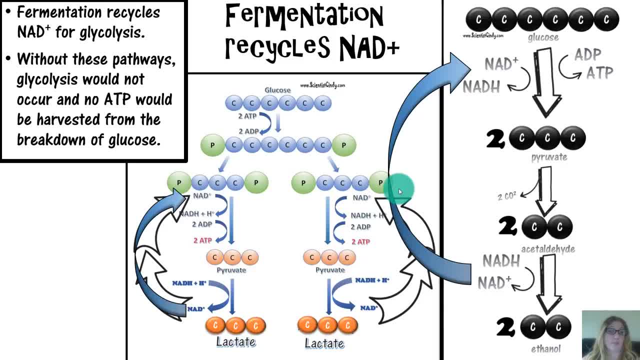 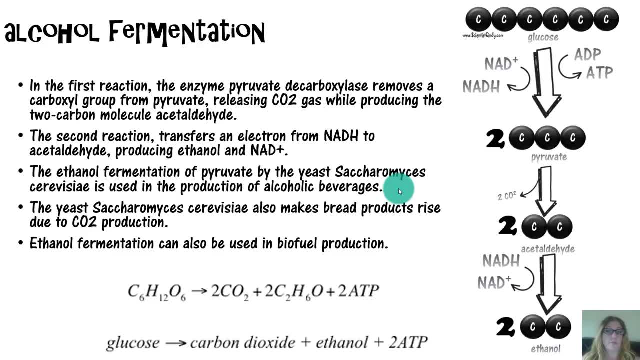 So no ATP would be harvested from the breakdown of glucose. So it's important to have these pathways. So alcoholic fermentation, what occurs here? So in the first reaction, the enzyme pyruvate. the enzyme pyruvate decarboxylase removes. 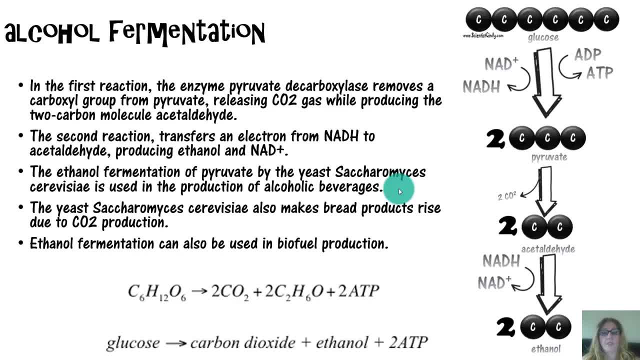 the carboxyl group from pyruvate releases carbon dioxide gas, while producing the two carbon molecule acetaldehyde. The second reaction transfers an electron from NADH to acetaldehyde, producing ethanol and NAD+. The ethanol fermentation of pyruvate by the 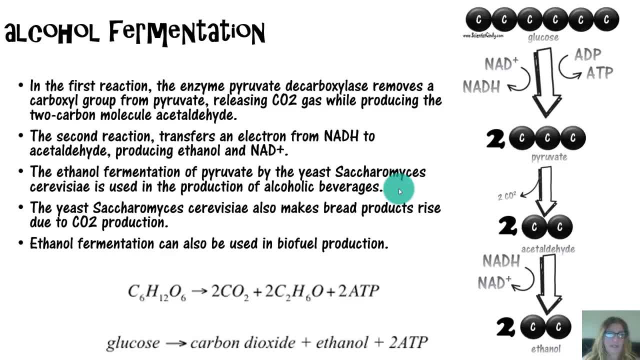 yeast saccharomyces cerevisiae is used in the production of alcoholic beverages. The yeast saccharomyces cerevisiae also produces bed products. bread products makes bread products rise due to its carbon dioxide production. Ethanol fermentation can also be used in biofuel. 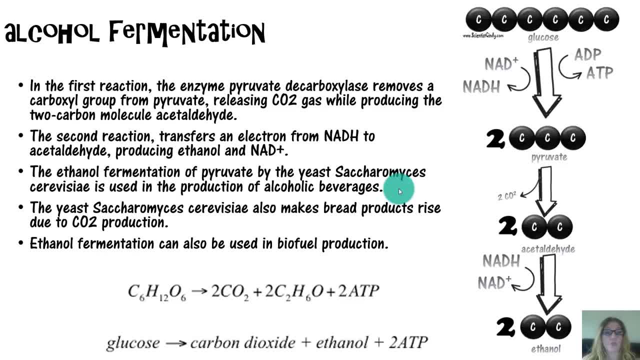 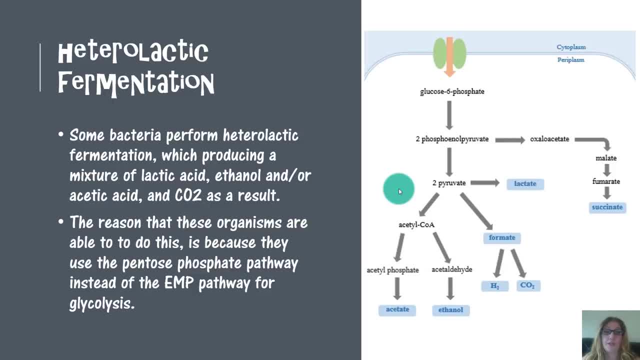 production- And here is the equation for alcoholic fermentation below. And there's even heterolactic or mixed fermentation. Some bacteria perform heterolactic fermentation, which involves producing a mixture of lactic acid, ethanol and or even acetic acid and carbon dioxide as a 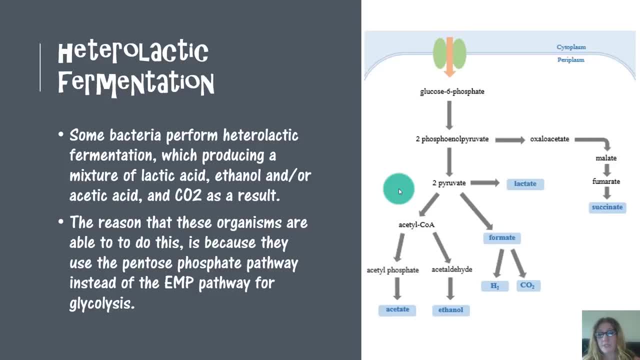 result. The reason that these organisms are able to do this is because they actually use the pentose phosphate pathway instead of the EMP pathway for their glycolysis. So we can see here that we're going to get all sorts of things We see succinate. 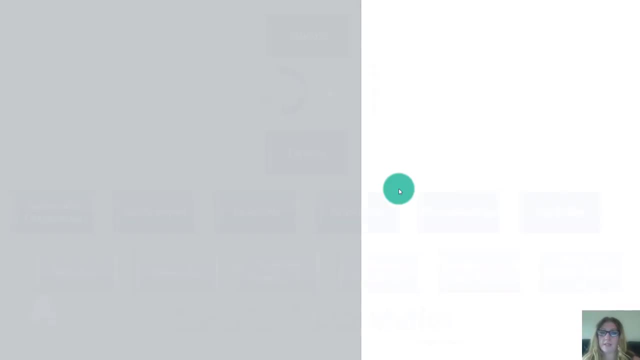 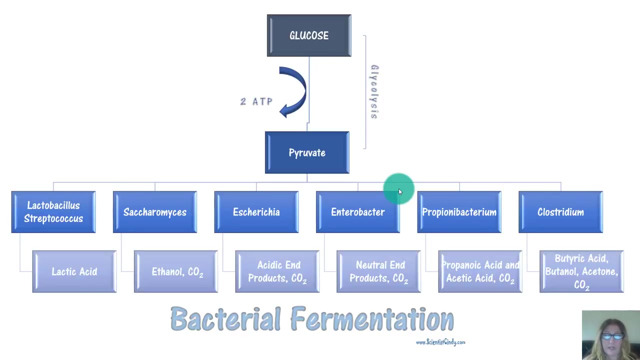 we see lactate formate, ethanol and acetate. So here's some of the important bacterial fermentation pathways that you should know. So we've got glucose generating 2 ATP during glycolysis and producing pyruvate, And then here 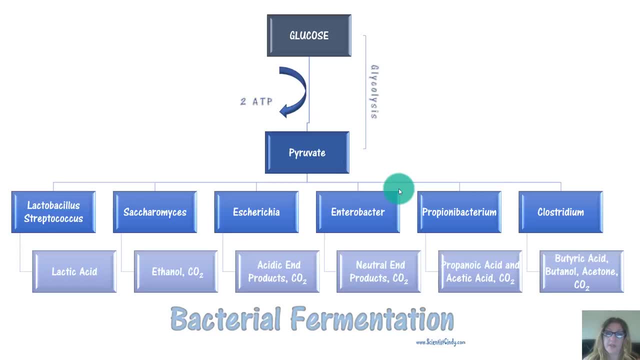 are some bacteria and some of their end products that they produce during their individual types of fermentation. So lactobacillus streptococcus are your lactic acid bacteria and they're going to form lactic acid fermentation, Your Saccharomyces cerevisiae. 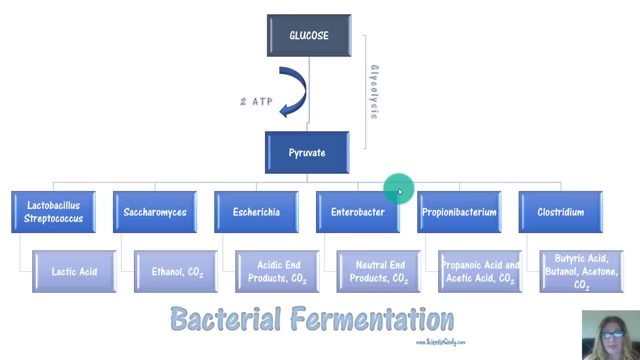 is going to perform your alcoholic or ethanol fermentation. E coli or Estercheria coli is going to create acidic end products along with carbon dioxide. Enterobacteria is going to create neutral end products, Propanoic acid and acetic acid is going to be. 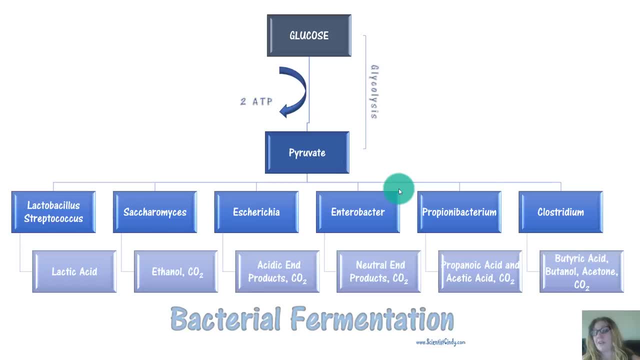 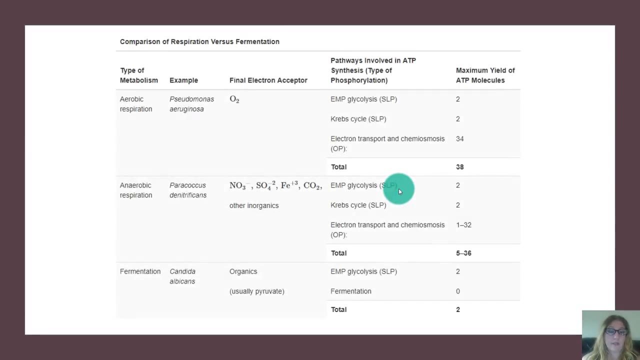 created by Propionibacterium and Clostridium is going to produce puric acid, butanol and acetone. Alright, so here's another great graph that I was able to find that shows different types of metabolism and different maximum yields. 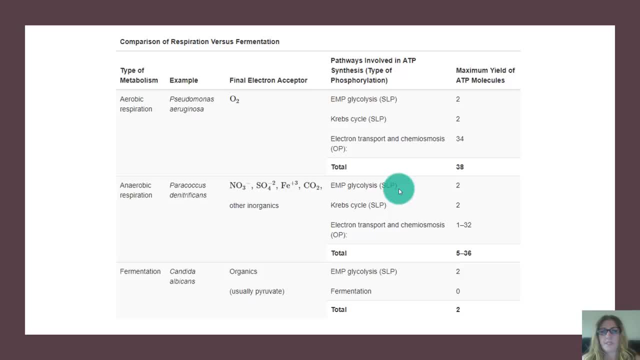 So here we see the different types of glycolysis and fermentation pathways and electron transport chain. So let's just take a look at this. So, types of metabolism. So let's first look at a microorganism called the Pseudomonas aeruginosa. 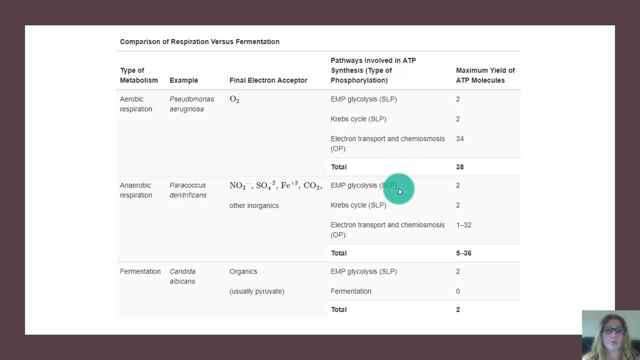 that undergoes aerobic metabolism. So this aerobic metabolizer uses oxygen, as it should. for an aerobic metabolizer, Aerobic respire, I should say. It uses the EMP glycolytic pathway, It uses the Krebs cycle And it uses the electron transport chain. 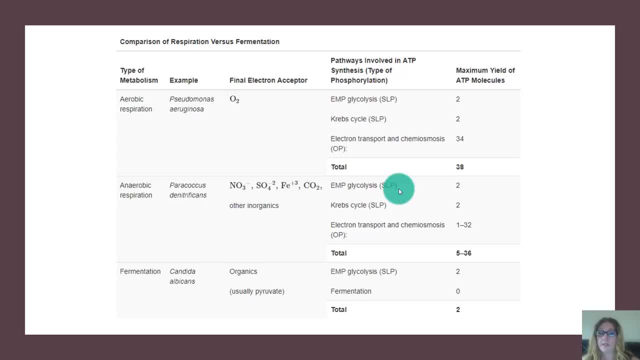 And it yields the maximum 38 ATP molecules. Here we have the anaerobic respirers, The pericoccus and the pericoccus denitrificans, which uses these inorganic molecules as electron acceptors And it is going to be able to produce. 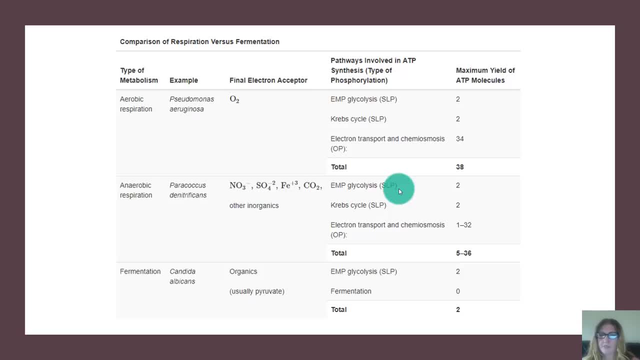 between 5 and 36 molecules of ATP, depending on what final electron acceptor is available at the time. interestingly, Fermentation, as it's being done by Candida albicans, will use an organic product such as pyruvate as its final. 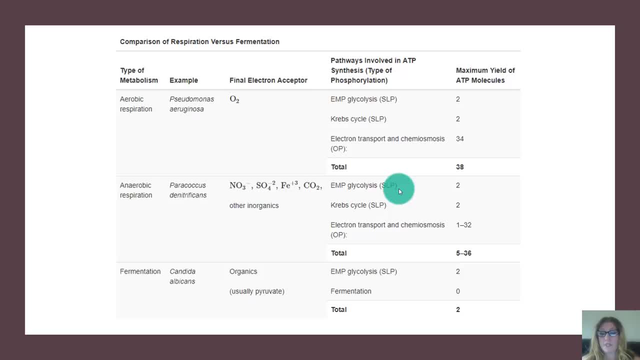 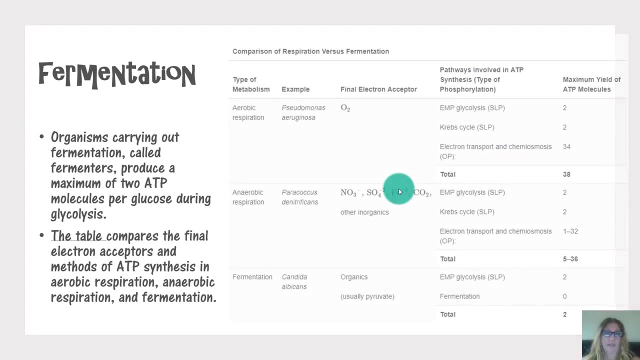 electron acceptor. So it is a fermenter and it is going to undergo the glycolysis process- the EMP version of the glycolysis process, followed by fermentation to yield only a measly 2 ATP. Okay, So organisms carrying out fermentation called fermenters. 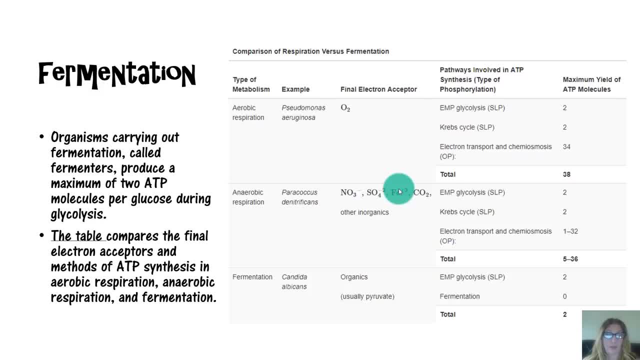 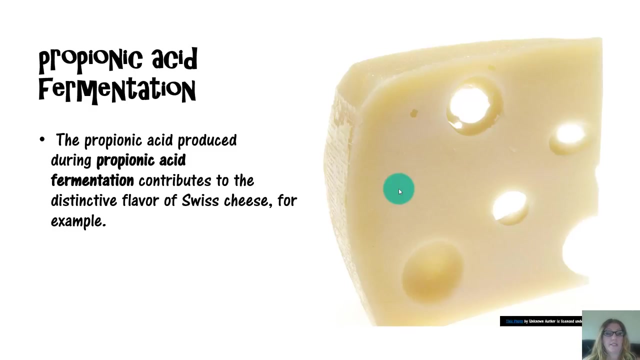 produce a maximum of only ATP molecules per glucose during glycolysis. So this table compares the final electron acceptors and methods of ATP synthesis in aerobic respirers, anaerobic respiration and fermentation. Propionoic acid fermentation is actually really cool. 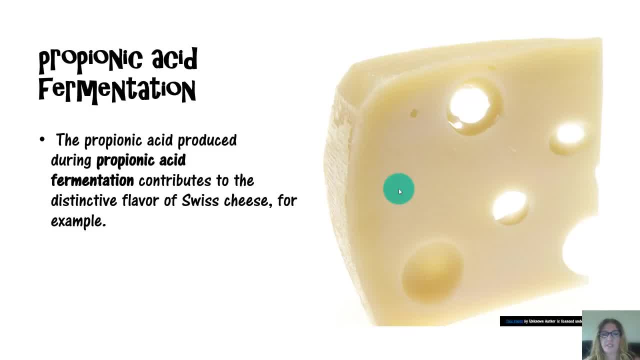 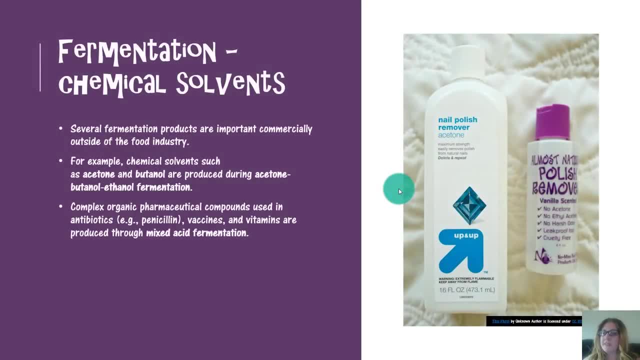 because we actually use it for Swiss cheese. It gives Swiss cheese that really distinct flavor That Swiss cheese has. Also, fermentation can give us things like acetone, which we use for nail polish remover, for example. We also get other products like butanol, which 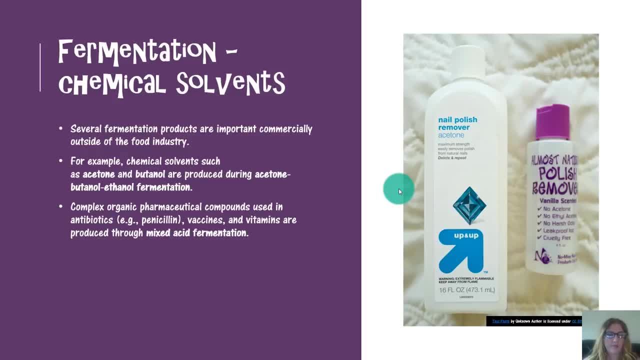 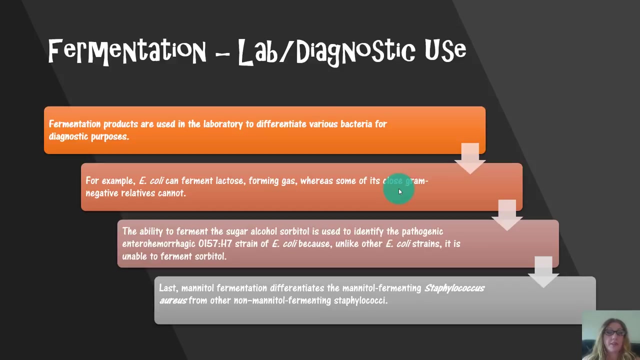 is another industrial solvent. We can also get things like pharmaceutical compounds, antibiotics, even vaccines and vitamins through things like mixed acid fermentation. We also can use fermentation products for lab and diagnostic use, For example. fermentation products are used in the laboratory to be. 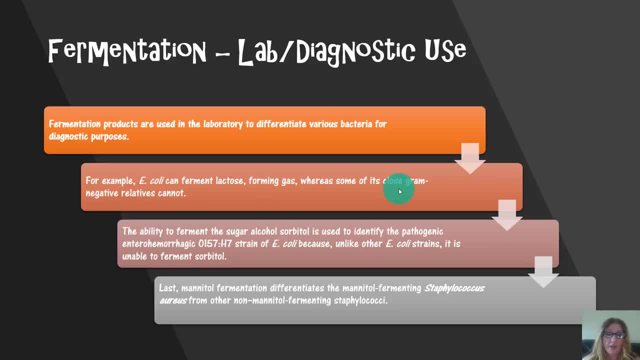 able to differentiate different types of bacteria from one another. E coli can ferment lactose And they form gas, whereas some of its close gram-negative relatives cannot, So that's a good test that can be used in the lab to distinguish it. 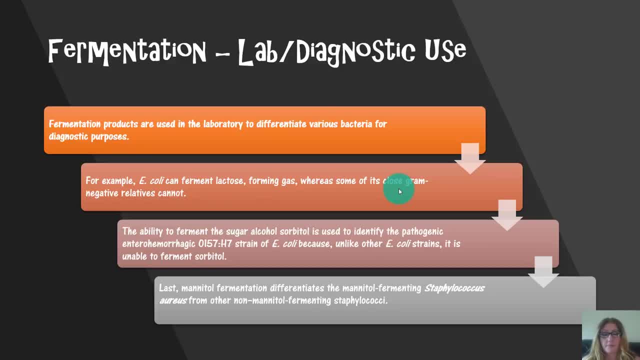 The ability to ferment sugar, sugar alcohol. sorbitol is used to identify the pathogenic enterohemorrhagic strain of E coli because, unlike other E coli strains, it is unable to ferment sorbitol, So that's very important. 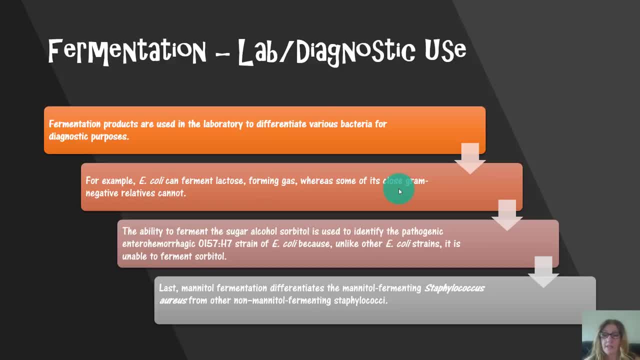 You want to know if you have that pathogenic version of E coli. And if it is unable to ferment sorbitol, then you know you might have that pathogenic version of E coli. So wonderful laboratory test that you can do to exploit that. 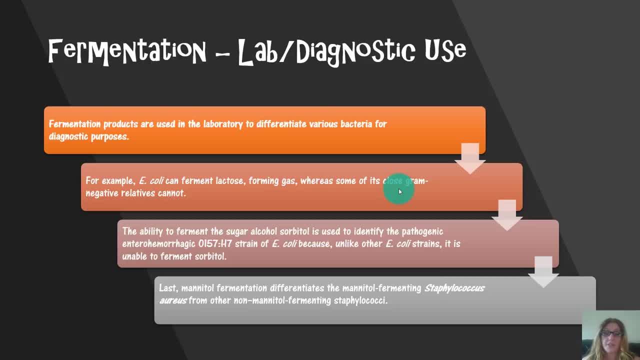 metabolic fact of that organism. Mannitol fermentation is going to be able to differentiate the mannitol fermenting pathways of Staphylococcus aureus from non-mannitol fermenting Staphylococci, So it's really good to be able to. 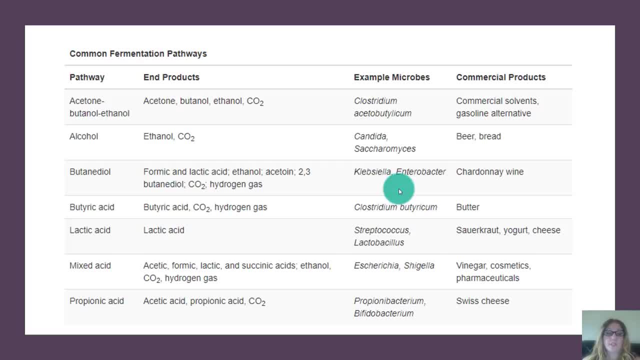 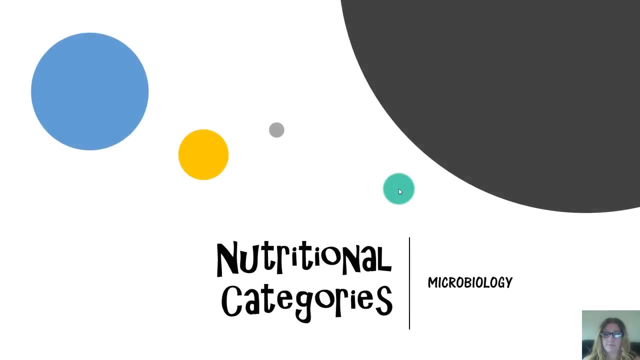 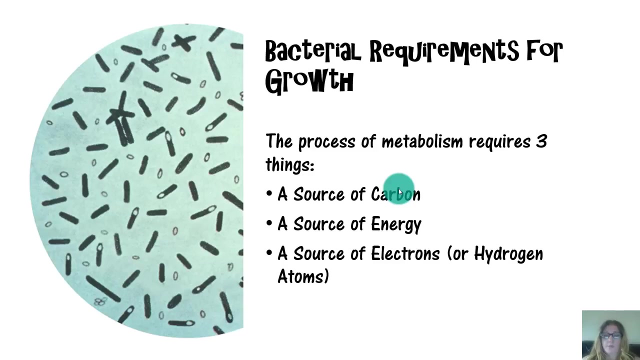 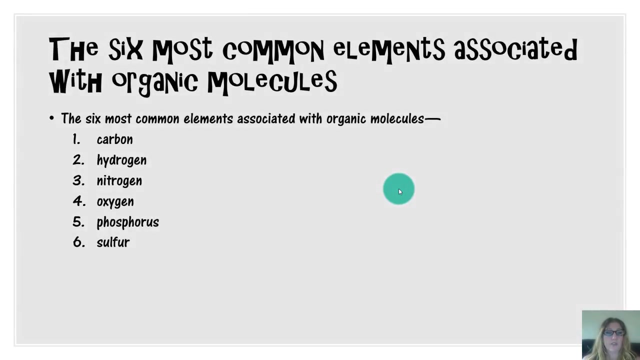 recognize one from the other. So here are some of the just another way to look at the common pathways. Alright, So in order for metabolism to occur, you really need three things: You have to have a source of carbon, you have to have a source of energy. 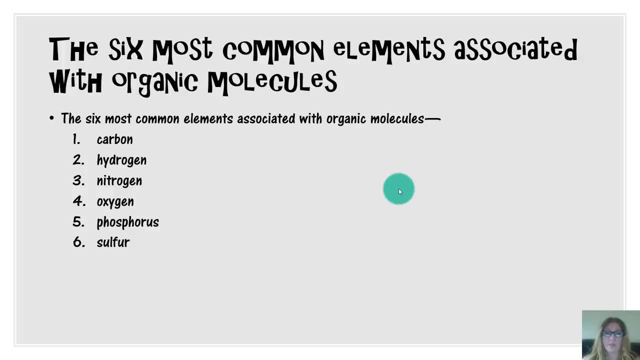 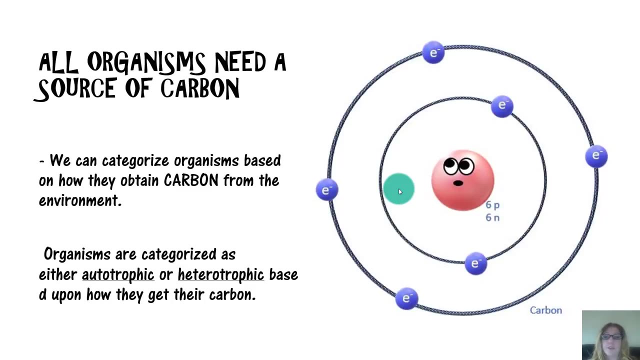 you have to have a source of electrons. So the six most common elements that we need to have is carbon, hydrogen, nitrogen, oxygen, phosphorus and sulfur. Alright, So how do we? we can actually categorize organisms based on what they use as. 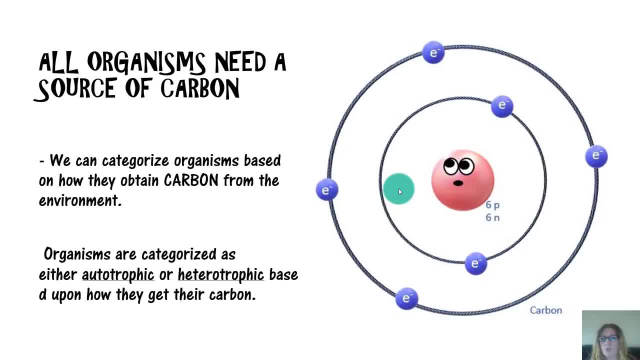 carbon sources what they use as energy sources. So I'll just give you just a couple of those things real quickly So we can categorize organisms based on how they obtain carbon from the environment. So organisms can be categorized either as auto. 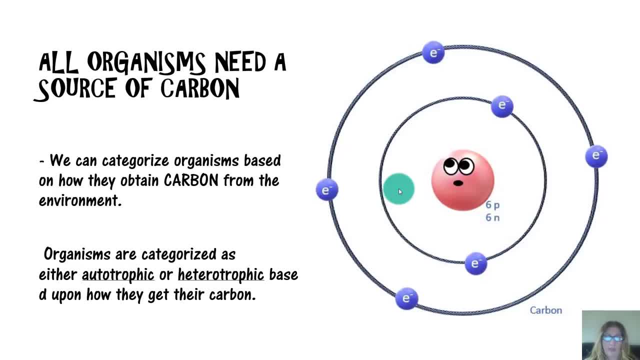 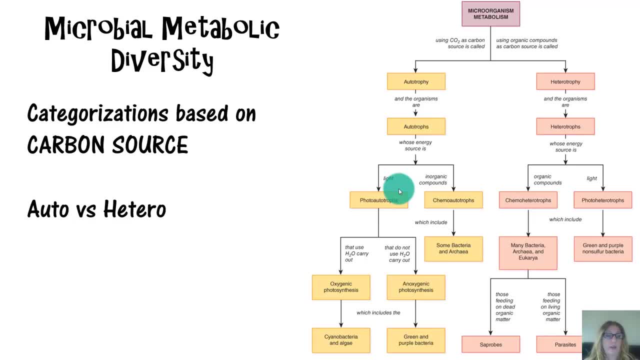 trophic or heterotrophic, based on how they obtain their carbon. So when we look at microbial metabolic diversity, here are some categorizations based on carbon sources. So we start here, at the top of our table, and it says microorganism metabolism. 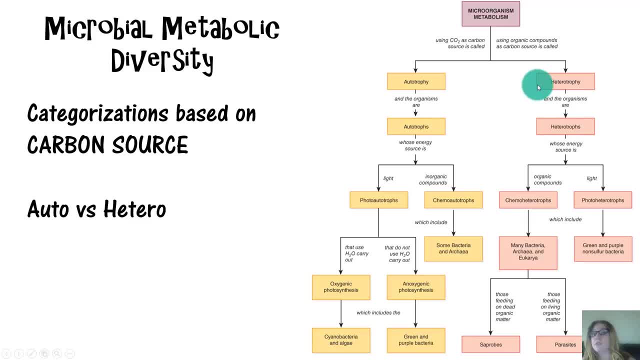 So if they are able to use carbon dioxide as a source of carbon, as a carbon source, then we can call them an auto-troph. When we say auto-troph, auto-troph means that they literally auto means self. 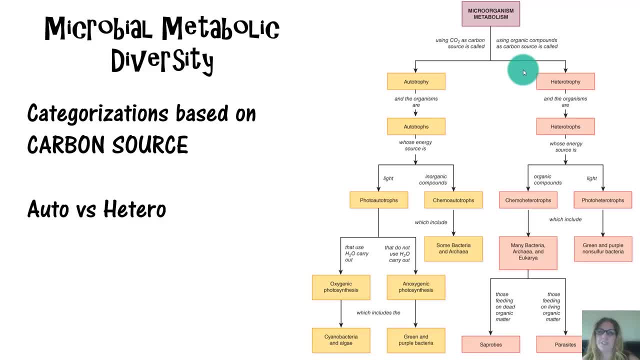 and troph means to eat, So the literal translation means to eat self, which is kind of weird. So it doesn't really mean that it's eating itself. What it means is that it's self-sufficient, that it doesn't. 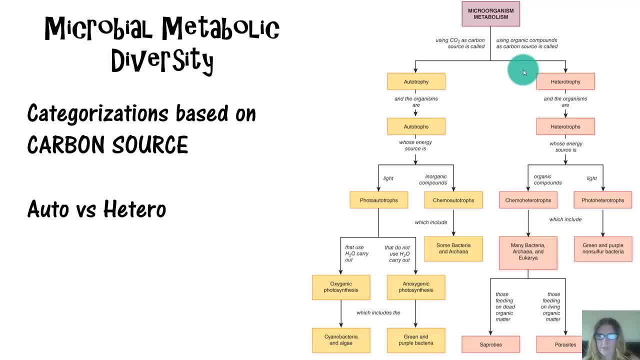 have to consume another organism. So, in other words, it's self-sufficient, It doesn't have to consume another organism. Versus heterotroph means eat other or eat another, So one doesn't have to eat anybody else. 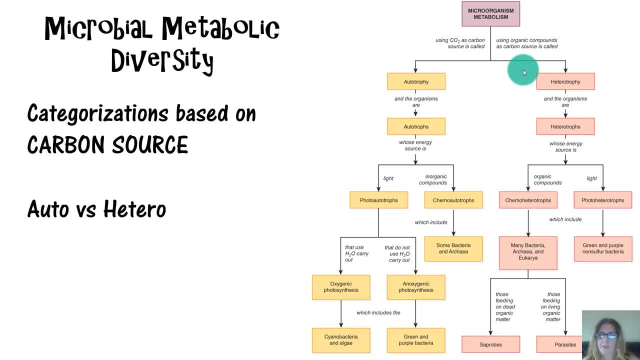 the heterotroph does. So we are heterotrophic. we have to eat other things in order to survive, Whereas a plant doesn't really have to eat anybody. So, unless it's a Venus flytrap or something like that, So okay, 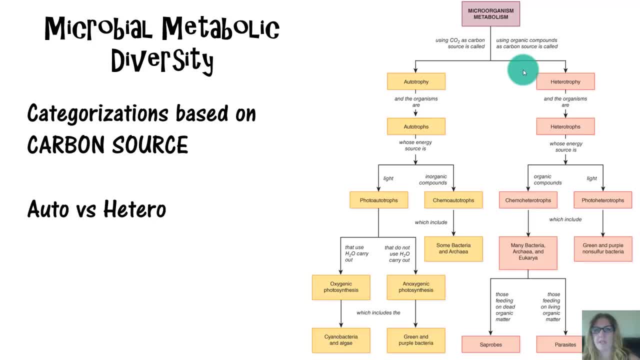 So the categorizations, so you just always have to go back to the pure definition. So if it uses carbon dioxide as a carbon source, then it would be categorized as an autotroph. As an autotroph, Alright, If. 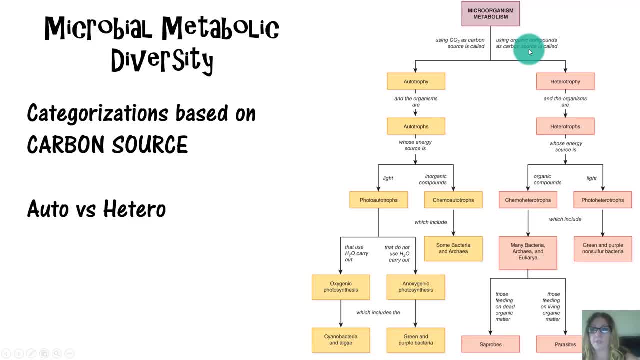 it uses an organic compound as a carbon source. it is a heterotroph. So when we say it uses organic compounds specifically, what we are referring to is lipid carbohydrate protein. That's it, Okay. An organic compound is a lipid carbohydrate. 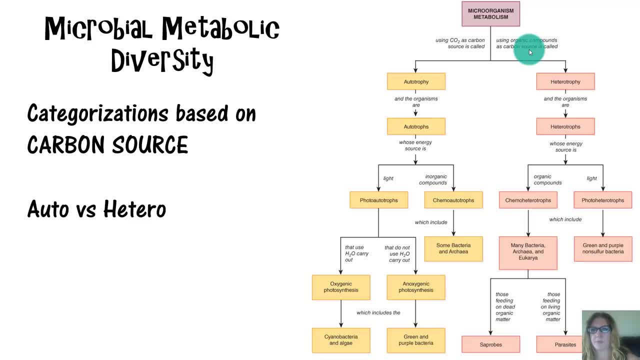 protein Always. So that's what we mean by organic compound. Alright, So let's go ahead and let's do the heterotroph side first. So we're going to go ahead and continue down the heterotroph side, So. 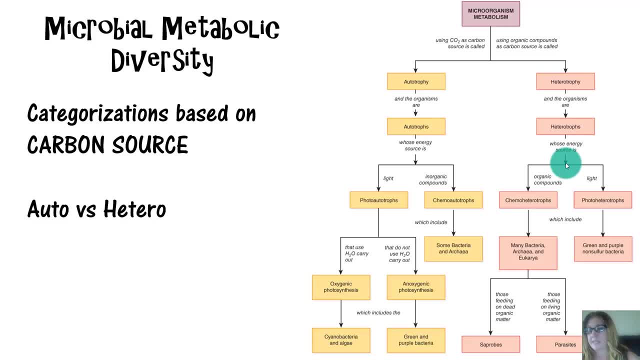 we're going to go down heterotroph and we see now it's going to split off into organic compounds and light. Okay, So some organisms are able to use organic compounds as a carbon source? Okay, So if it can use an organic 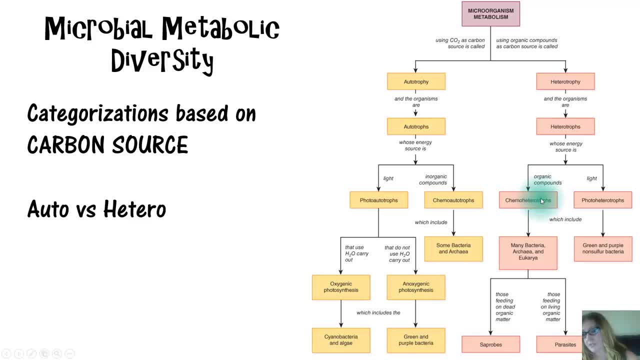 compound as a carbon source but it needs to use, and it needs to use an organic compound as an energy source, then it would be a chemo heterotroph. A chemo heterotroph- Okay, Chemo in this sense comes from the. 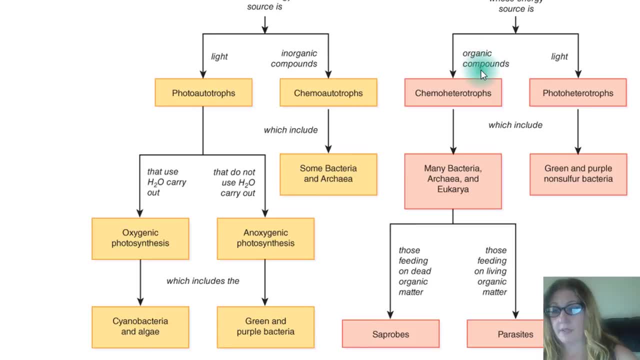 organic compounds here. Okay, So what does this mean? Alright, So we see, feeding on living organic matter, living on dead organic matter, That sounds great. So, yeah, So eating the living and eating the dead, That sounds wonderful. 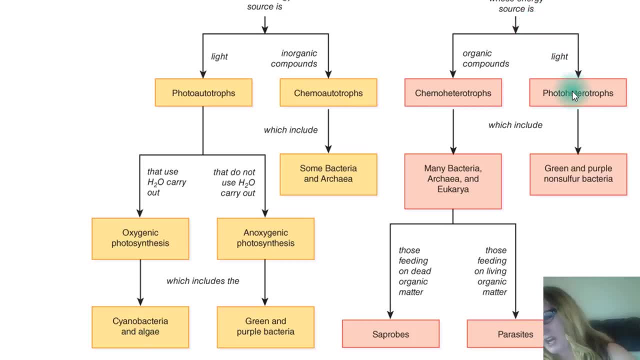 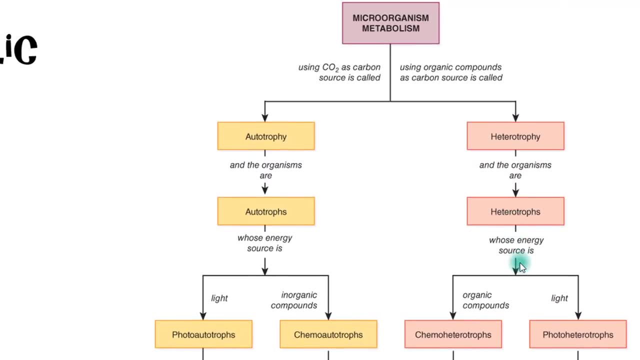 Will you get me a chocolate? And then let's see, Okay, And then if it's able to, if it's able to use an organic compound as a carbon source but light as an energy source, then we call it a photo-heterotroph. 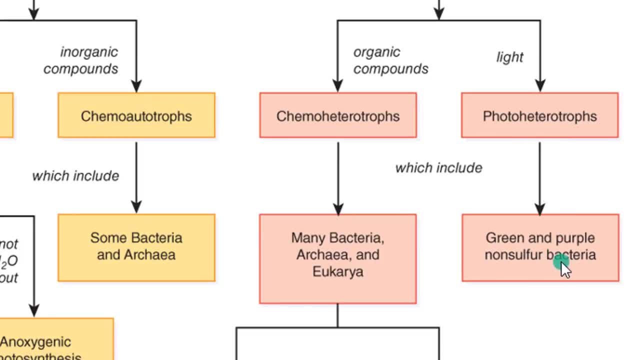 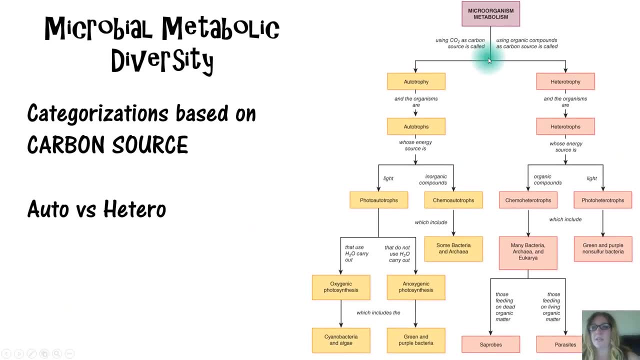 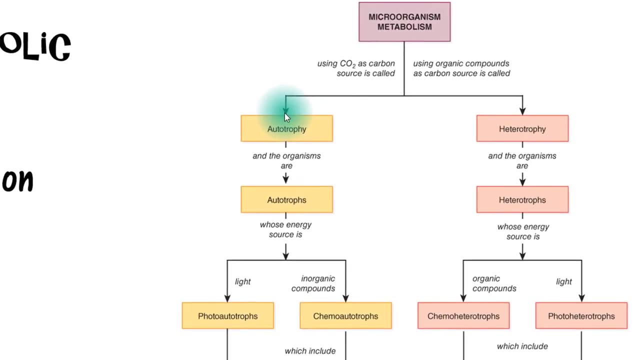 Examples of this would be green and purple non-sulfur bacteria, So they do that Alright. So let's go the other side, So using carbon dioxide as a carbon source. these are our autotrophs, Okay. 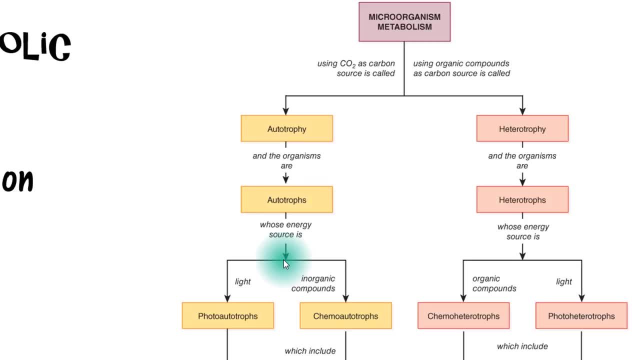 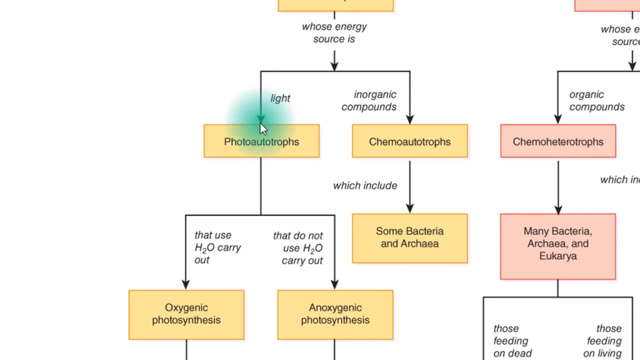 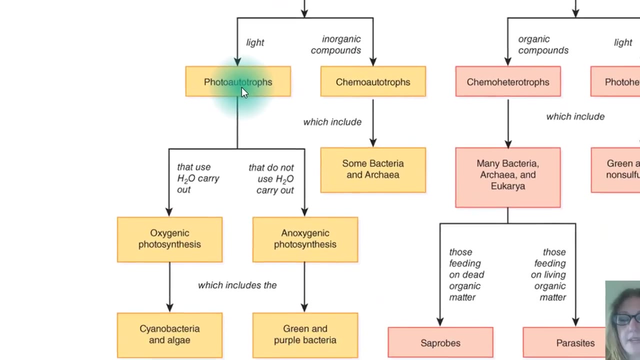 So autotrophs and using carbon dioxide as a um, as a carbon source, using light as an energy source, we get our photo autotrophs. So the auto part comes from the carbon dioxide carbon source, The photo part comes from the 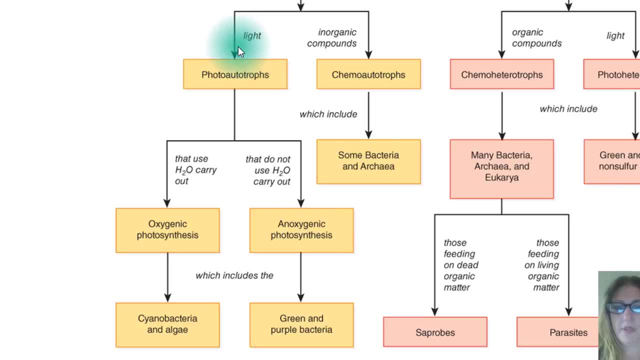 light as the energy source. Okay, Now we will continue down, And now we're going to have the ones that use water and the ones that don't use water. Okay, That use water carryout and the ones that don't use water carryout. 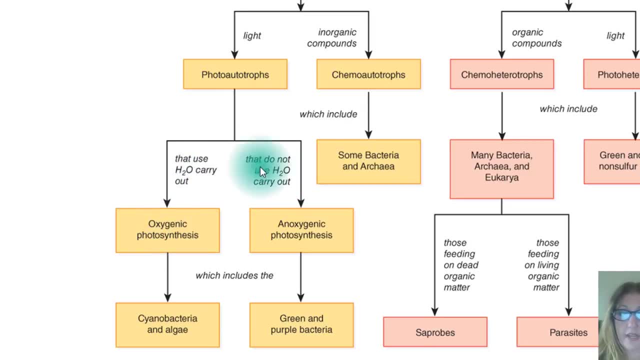 Okay, And we get our oxygenic and our anoxygenic, So some make oxygen and some don't during the process. The ones that do make oxygen, those are cyanobacteria that changed our atmosphere right, And algae, which are 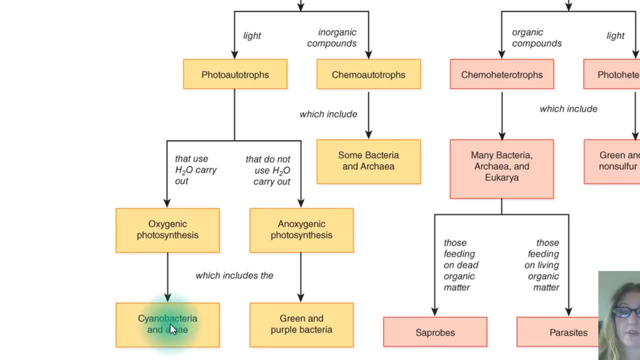 eukaryotic Algae are eukaryotic, Cyanobacteria are prokaryotic. Now our anoxygenic photosynthesizers would be green and purple bacteria, for example. Now what if I go the other way? 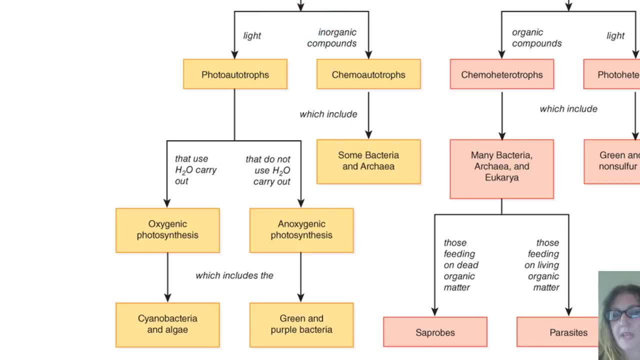 So, um, we have organisms, microorganisms, that use carbon dioxide as a carbon source, And then they can use inorganic compounds. Okay, These are chemo autotrophs, And this can include some bacteria and some archaea. So really, 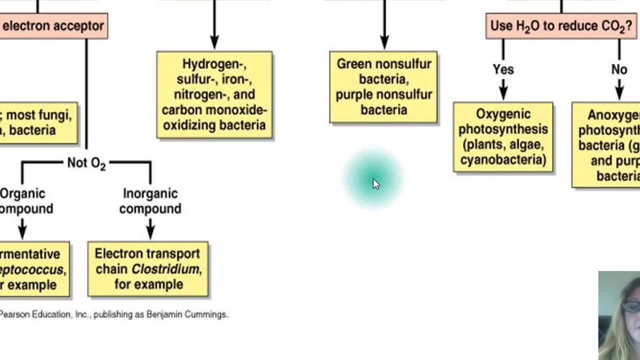 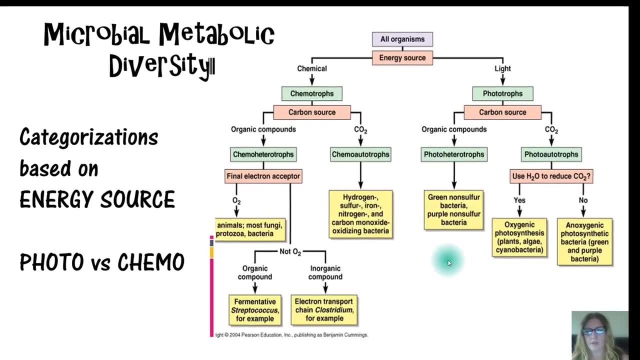 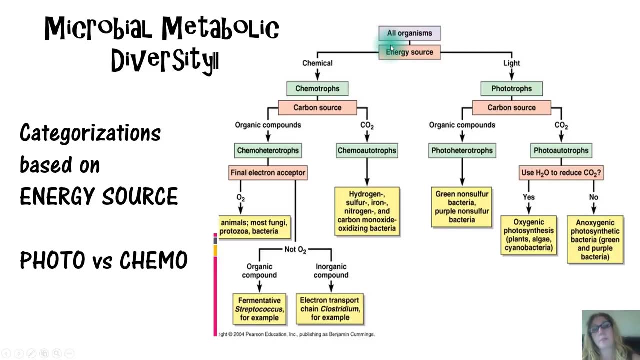 it's like boy, anything goes. Um, we could also reorganize the table in another way to categorize based on the energy source first, And if we did that, then it would look like this: So we have energy sources, So if it's chemical, 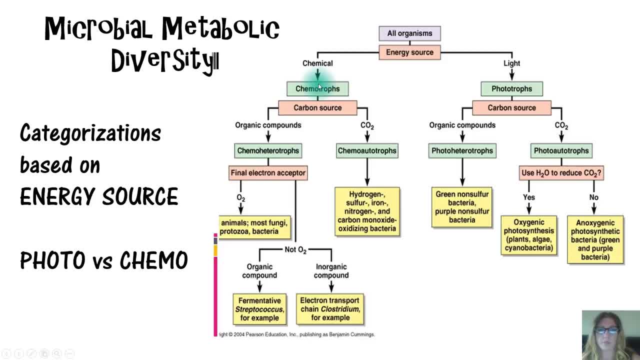 okay, and that would include, um, you know, food, like having to eat, versus I can't eat sunlight and live for long, So you have your phototrophs, photonewing light, So eat light okay. so this is our light. 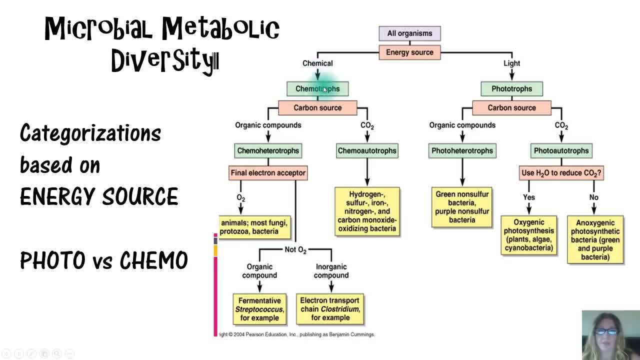 eaters. Okay. versus chemical. well, we need chemical energy, so we actually have to ingest things that have molecules that we can break down and metabolize right. So we have our chemotrophs and our phototrophs. 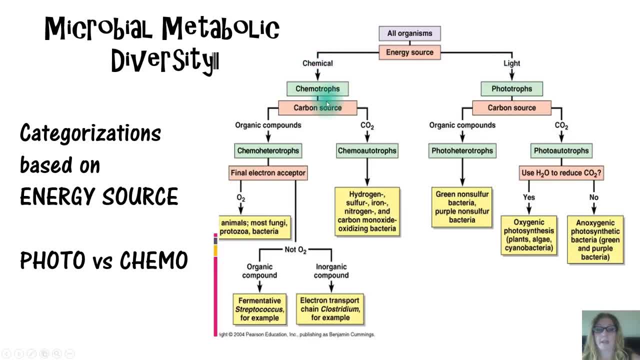 Alright, Now and then after that. then we can go ahead and separate it into its individual carbon sources. So we have our chemo heterotrophs and, depending on its final electron acceptor, if it uses oxygen versus if it does not use. 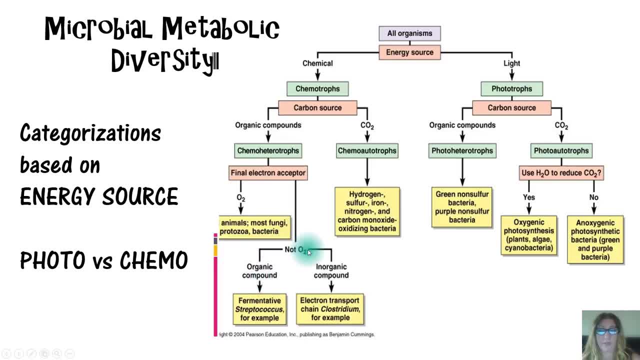 oxygen. So if it's anaerobic, it would be here. okay So, but it could be, um, it could be anaerobic, but it could use an organic compound. Okay so, if it's anaerobic and it uses an organic compound. 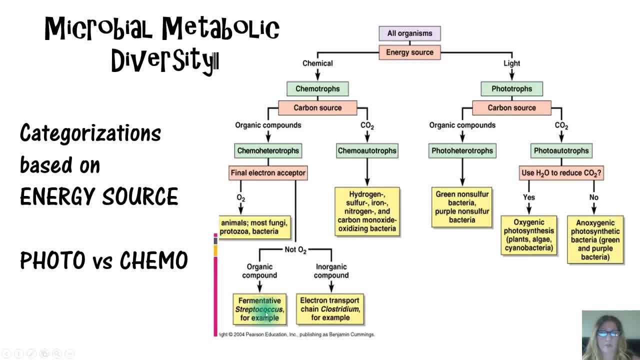 these are going to be our fermenters. Alright, These are our fermenters. They're going to undergo fermentation, Okay. However, if they are here, then that means, um, that they are going to undergo anaerobic cellular respiration. 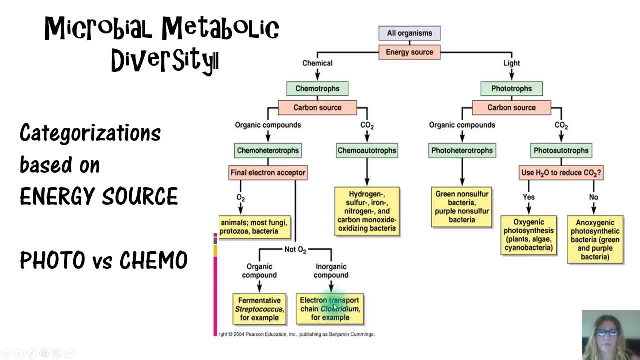 Not fermentation. Okay, Anaerobic cellular respiration, that is not fermentation. Alright, Versus, we could go this way too. You've got your chemo heterotrophs, so this is where we would be here on this, on this map. So, organic compounds. 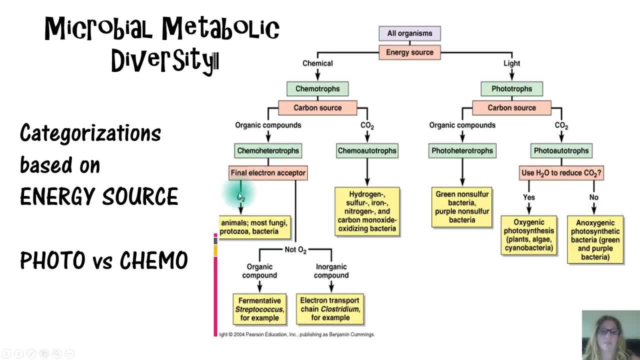 we have to consume them, Um, and our final electron acceptor is oxygen, And we would be here. Alright, let's look at the other side. So we've got our um, our photosynthetic organisms that eat light, Alright, so 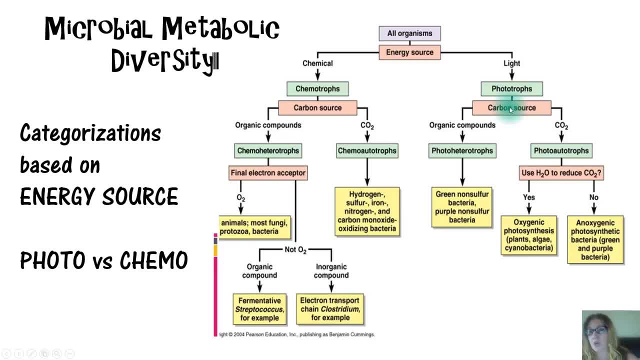 as an energy source they're going to take in light, But they still need their carbon source, right? So, um so, some can use carbon dioxide Is their carbon source. Those would be your photoautotrophs- Photoautotrophs. 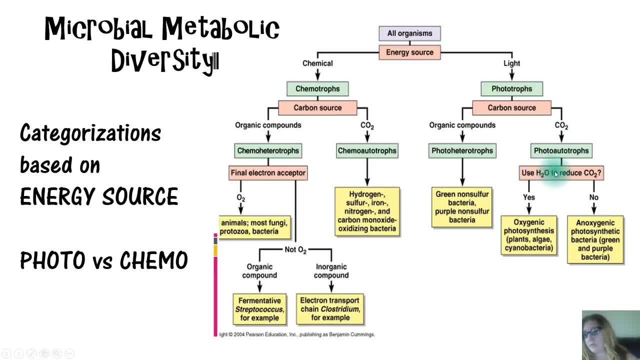 And some are going to use water to reduce carbon dioxide. If it does, it's called oxygenic Because it's actually going to create oxygen. If it does not use water to reduce carbon dioxide, it does not produce oxygen. Okay. And on the other side we've got 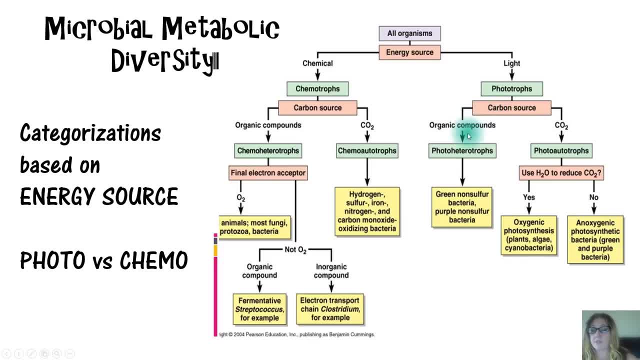 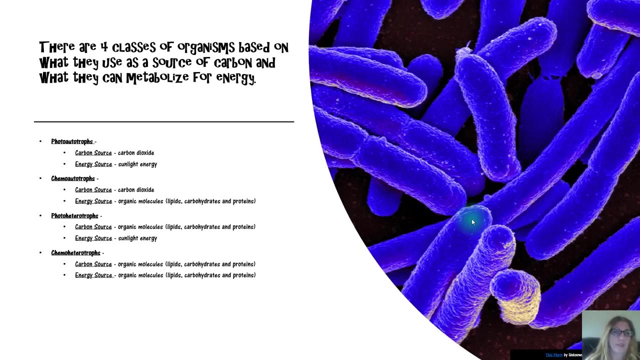 organic compounds As the carbon source. So our organic compounds are needed for our photoheterotrophs, And these examples of this would be green non-sulfurous bacteria and purple non-sulfur bacteria. Okay, So there are four main classes of organisms. 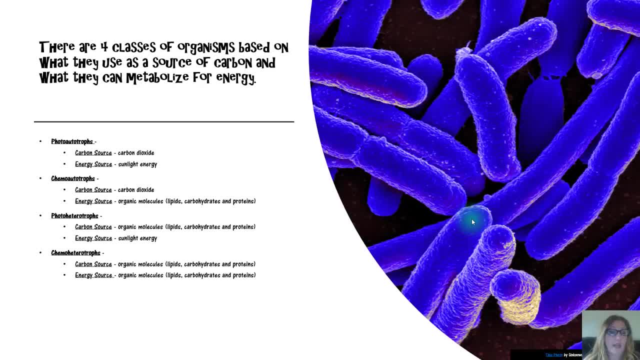 based on what they use as a source of carbon And what they can metabolize for energy. So when we say photoautotroph, photoautotroph means that the carbon source is carbon dioxide And the energy source is sunlight. Okay, 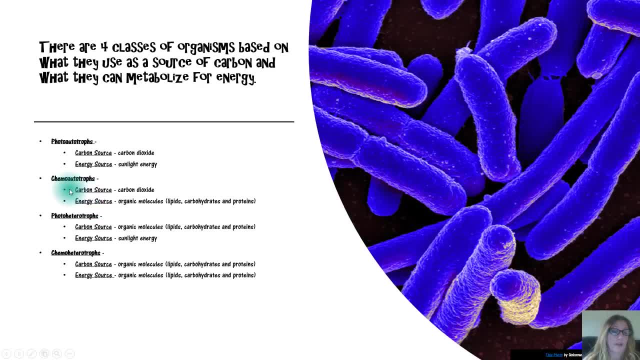 Chemoautotroph. um, chemo means, uh sorry. The carbon source is carbon dioxide and the energy source is organic molecules. The photoheterotroph is carbon source, is organic molecules And the energy source is sunlight. The chemo. 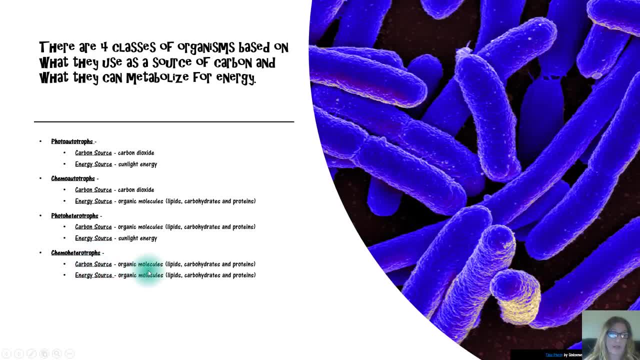 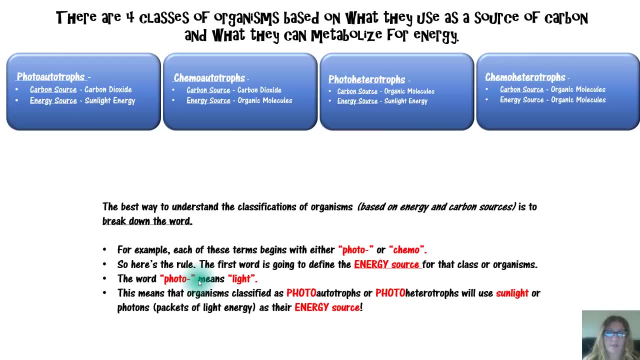 heterotroph is, the carbon source is organic molecules, And the energy source is also organic molecules. Okay, Okay, so I think this is more of the same here. So I think the best way to do this is just to break it down into its carbon source and 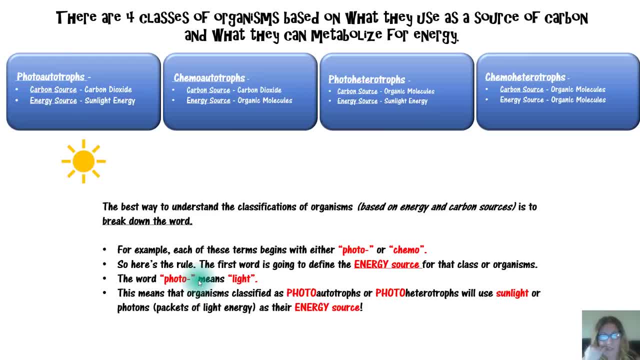 its energy source right. So first of all you just want to look at is the best way to understand its classifications based on energy and carbon sources is just to simply break down the word. For example, each of these terms begins with either photo or chemo. 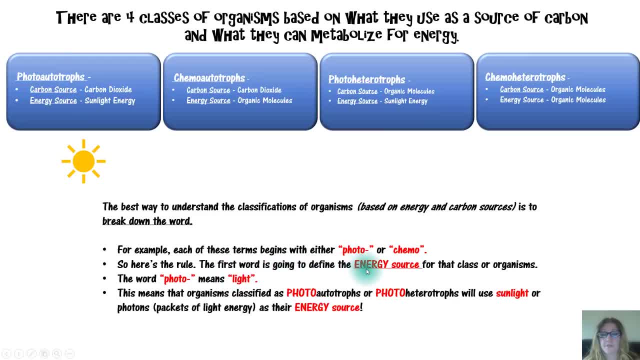 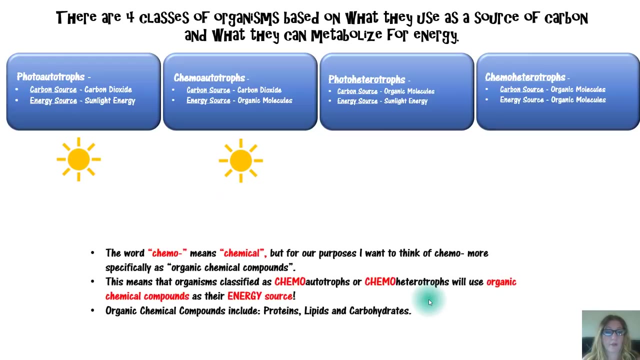 So here's the rule, For the first word is going to define the energy source for that class of organism. Photo means light. This means the organism classified as photoautotrophs or photohepatitis. Heterotrophs will use sunlight or packets of energy called photons as their energy source. 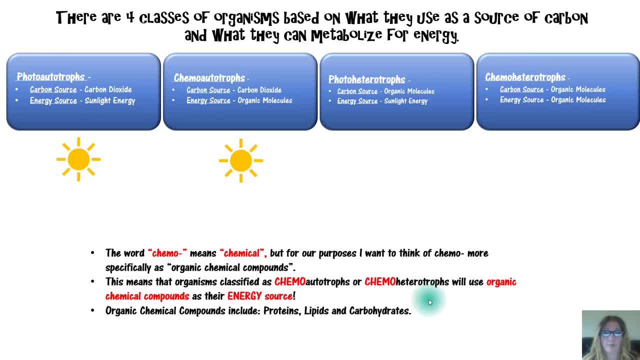 The word chemo means chemical, but for our purposes I like to think of chemo as specifically organic chemical compounds. This means organisms classified as chemoautotrophs or chemoheterotrophs will use organic compounds. Organic chemical compounds mean proteins, lipids and carbohydrates. 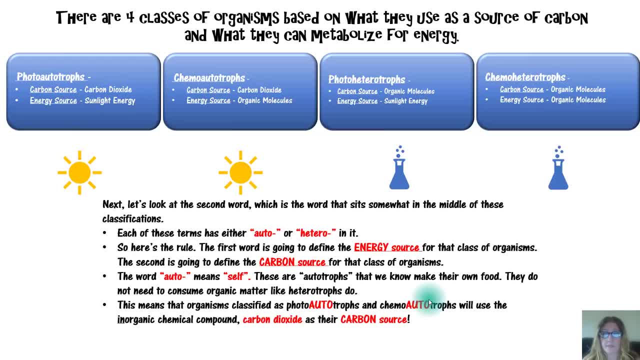 Next we can look at the second word. The second word sits somewhat in the middle of these classifications. Each of these terms is either auto or hetero in it, So here's the rule. The first word is going to define the energy source for that class of organism. 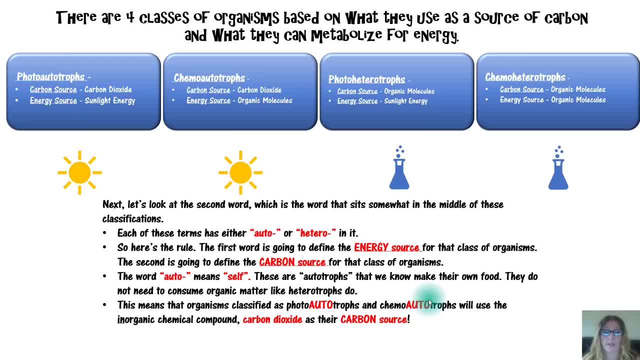 The second is going to define the carbon source for that class of organism. The word auto means self. These are autotrophs we know to make their own food. They don't need to consume organic matter like the heterotrophs do. 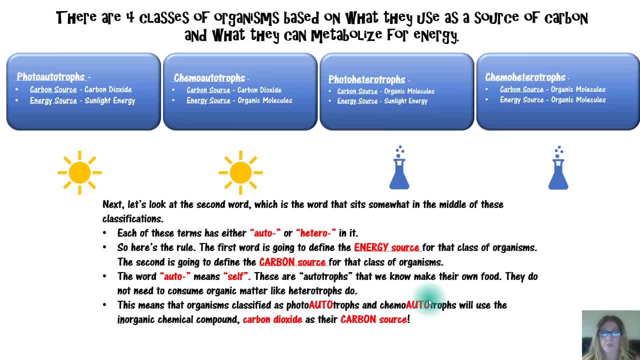 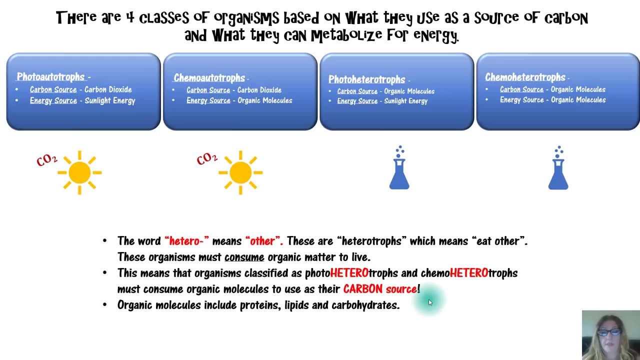 This means that organisms classified as photoautotrophs- Their name Chemoautotrophs- will use the inorganic chemical compound carbon dioxide as their carbon source. So here comes your carbon dioxide for your autotrophs. Now, the word hetero means other. 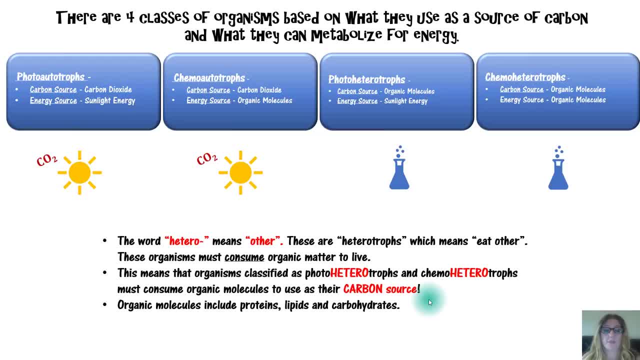 These are heterotrophs, which means eat other. These are organisms that must consume organic matter in order to live. This means that organisms classified as photo-hetero-trophs or chemo-hetero-trophs must consume organic molecules to use as their carbon source.